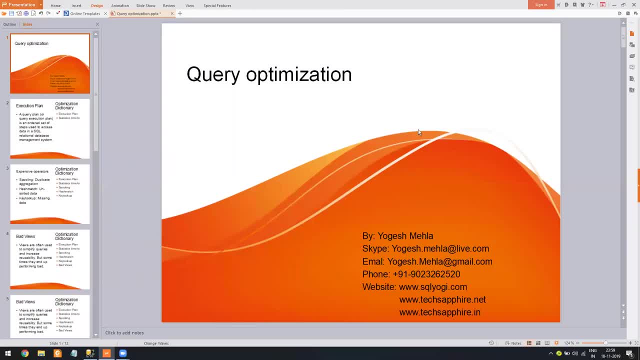 Hello everyone, my name is Yogesh. In today's video, I will explain you how to do a query optimization in SQL Server. Now this session is, you can say is, split into two things. This session will cover only one of them. The worst thing is like finding which are the queries. 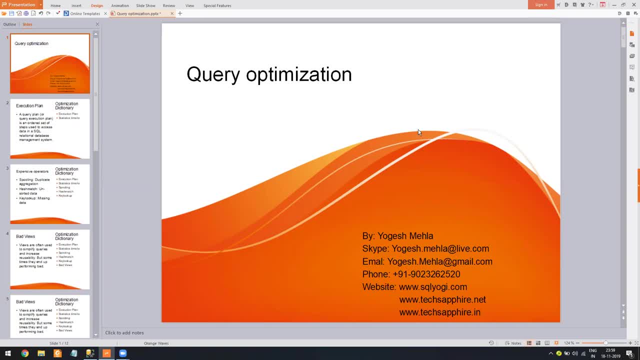 which need an optimization- and that's a separate video I will be making in future- and there are a lot of thick, you can say, not a trick, a mechanism to figure out which query need an urgent performance tuning so that your server can have an impact. Now understand one, almost the main thing. It's 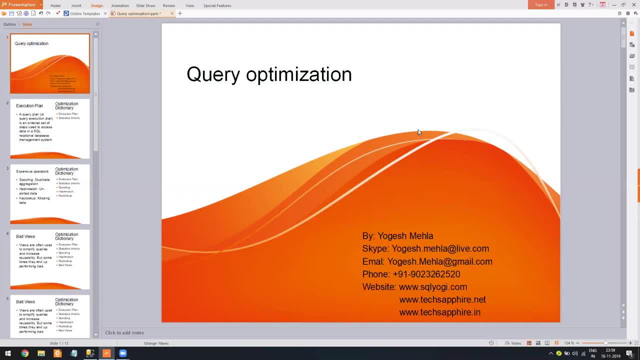 not about the query which is running for a long time is damaging your server. In a lot of the cases, small running queries can also damage. So that will cover in this scenario and we will figure it out how it makes a difference. Okay, so in this video, to be very clear, I am telling you. 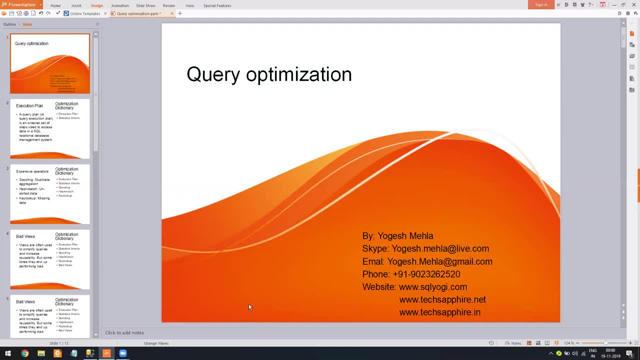 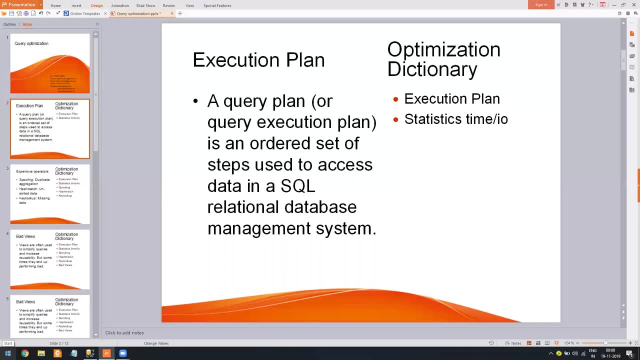 how to optimize your query, not how to find the bad queries, So that's a separate topic. Okay, so let's start Now. before starting any tuning, the first thing is you should be able to know how to see an execution plan, and most of the time I have seen people they don't know how to see the execution. 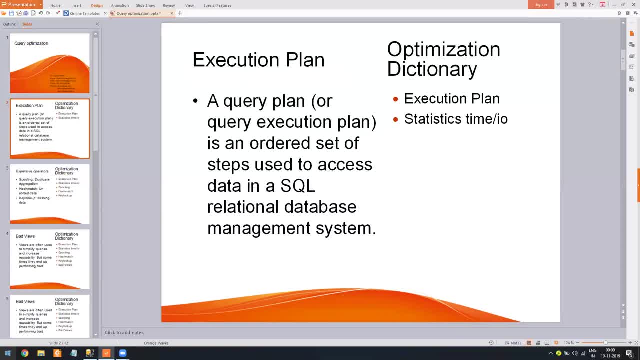 plan itself. They know the basic rule, data form: right to left and so on. So the execution plan is from left to right. but that's very basic. Even I don't even look into those part till the time it's not necessary. So the first thing is just seeing an execution. When suppose you have a plan of like? 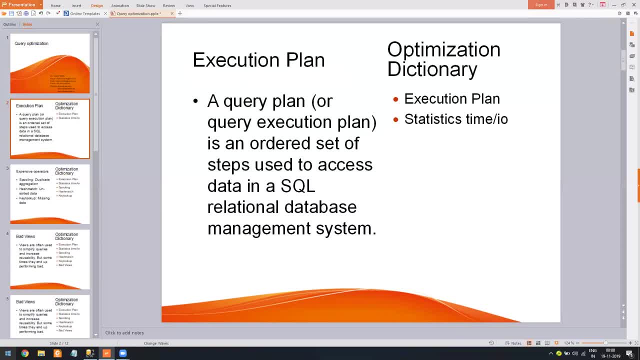 1000 lines. that's it, line of query which is having 100 joins, you can say, and 10-20 sub-queries. you won't be able to figure it out where the problem is, So this session will. 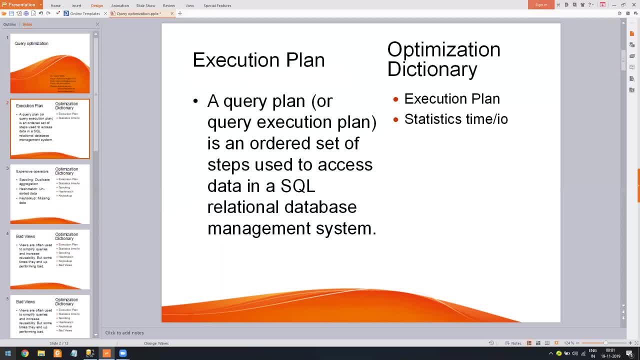 be more focused on that. Just by seeing the plan, you will be able to understand which part is having the problem and you will be able to figure it out: where is that part and then how to fix it. Now, how to fix it will depend upon. 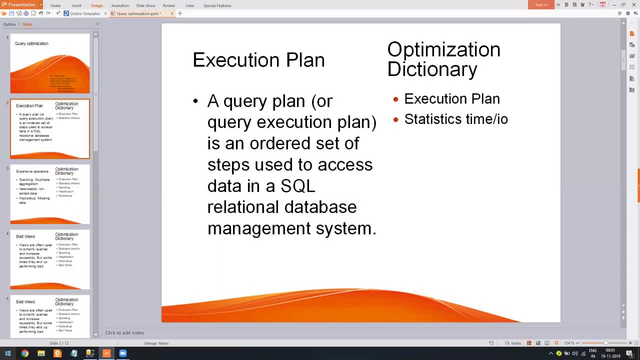 you can say query to query because you understand, like SQL server is something where general programming rule doesn't apply. Give an example. So in a programming, let's say if you are a NET developer, if I ask you, what are the OOPS concepts? 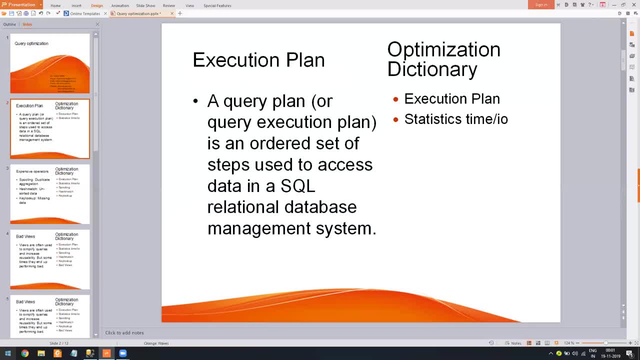 what is solid principle? you will be able to answer and there is a way of doing certain things. But in SQL server there is a way of writing the query. It can be possible, Naming convention can be possible, but your database will be different and my database 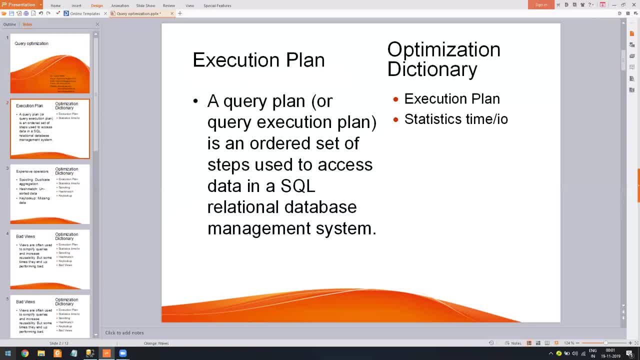 will be different, So your join condition will, be for sure, different than mine. So that's why we cannot assume one solution will apply everywhere, but I will tell you where. so these things, what I will be explaining, will be common across all the execution. 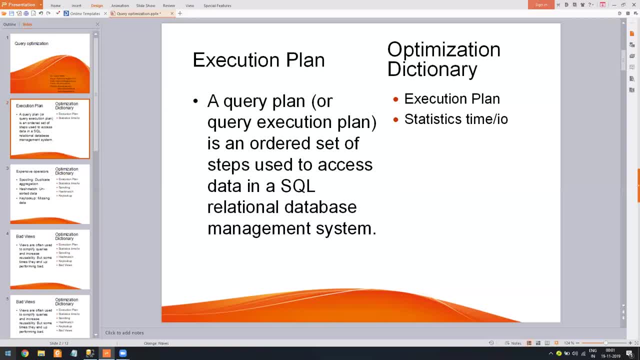 plans. So it doesn't matter whether you are using any database, it will still tell you, like where is the problem and how to fix it. I will cover few scenarios, Okay, So let's start with the first basic thing. So first thing is like how to read an? 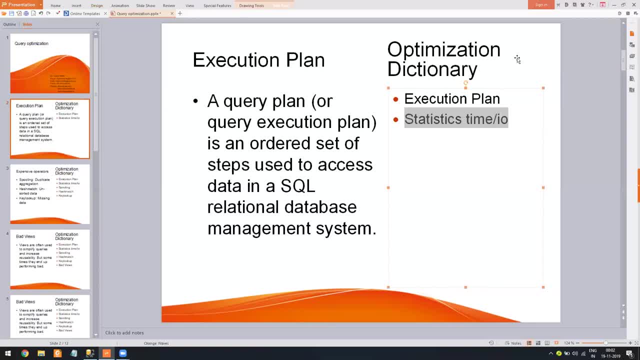 execution plan and use statistics, time and IO. Now a lot of people think like long running query is a problem, as I told you in the initial itself. but a lot of times small running query- it can be more problematic- Means suppose you have a long. 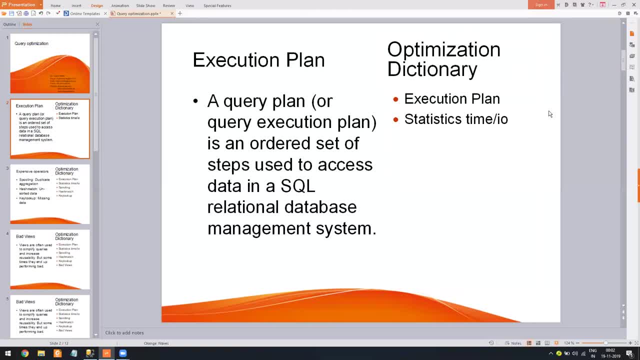 running query which you need to run in a once a month or twice a month, Then what will happen is you still can afford for two or three hours query, But if a small running query which is taking three seconds- and I use that query one million times- in a second- 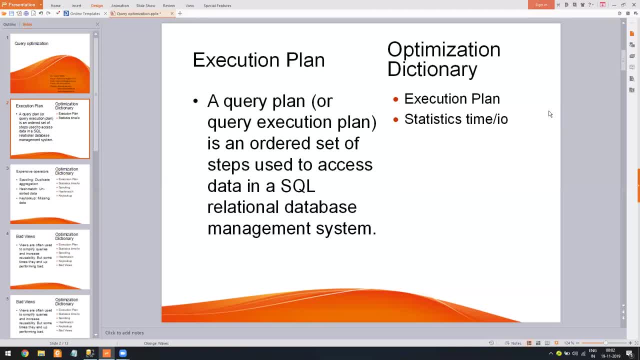 then your server has a problem if that query is not tuned. So all the things goes to that, like how many you can say times the query is running and how bad it is making to the server. So let's start with a basic execution. 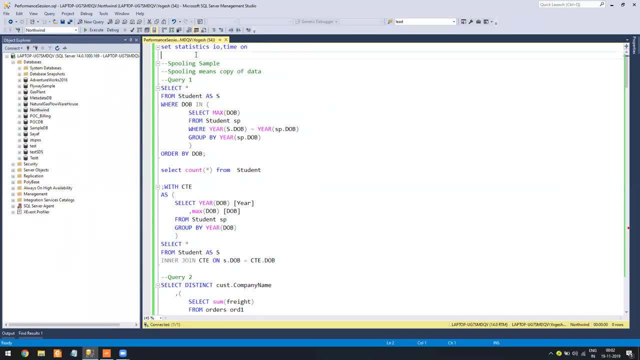 plan. Now understand one thing: If you are a DB or a SQL developer, still you need to follow the same statistics. So next steps. So first is, you should always enable statistics, IO and time on. So if you don't, 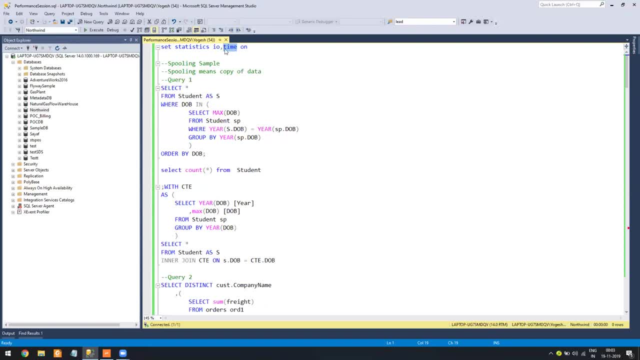 need time because you know the time, so then you can ignore it. But IO is the most important part, and why it is most important part is suppose your query is. so if you are not familiar with a few terms, let me just introduce I. 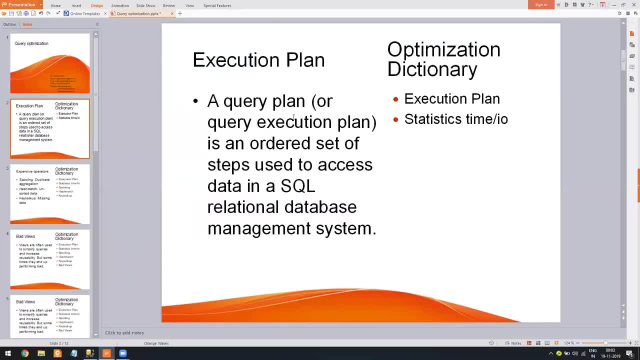 haven't made them in slides, But let me explain you. So there is one term called as physical read and logical read. Physical read is nothing but actual reading of data from the disk, and the logical read is reading the data from the memory. Now 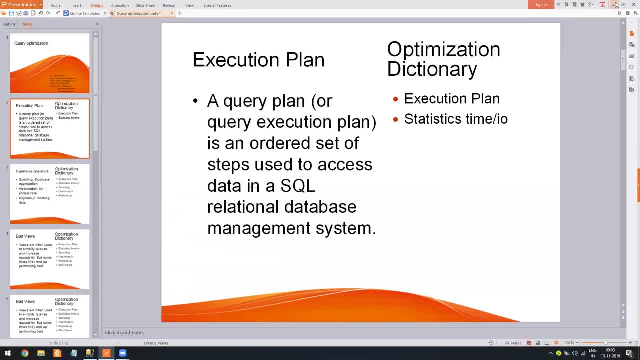 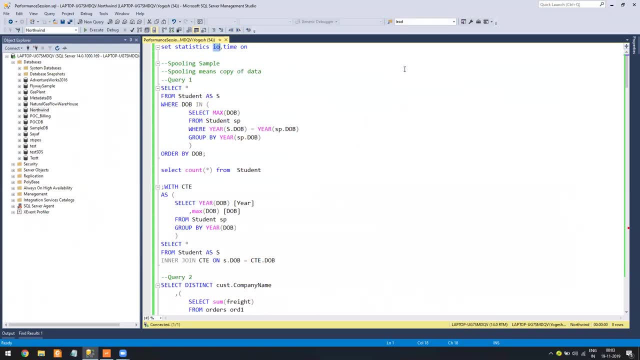 when this thing happens. so your SQL server do a lot of IO operation. IO can be logical and physical. IO means input, output. It has to read data from the memory, It has to put the data into some memory and it has to give you data from the memory or 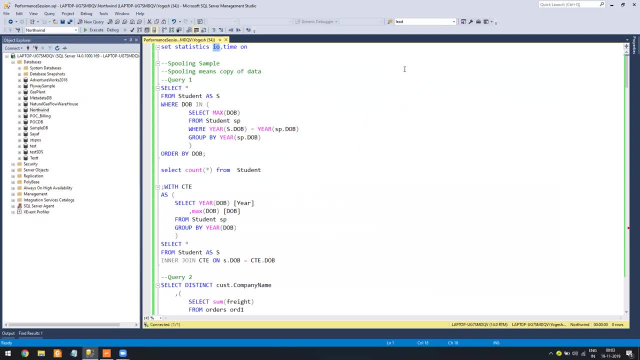 it has to read data from. So there is some steps like it could be possible. you are querying two tables. both are in memory. It is reading one table, filtering it out, certain record, then reading again table, filtering out certain record, and making a join and giving the output. 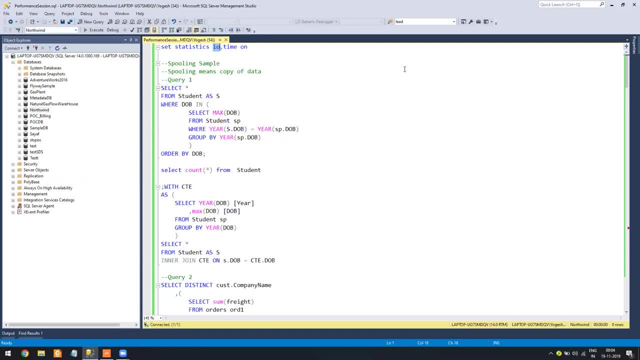 So in all the operation there is an input output involved and there is a time always there. So time is a secondary unit. The first thing is input output. Suppose I have a query which runs in one second and do one million logical reads. 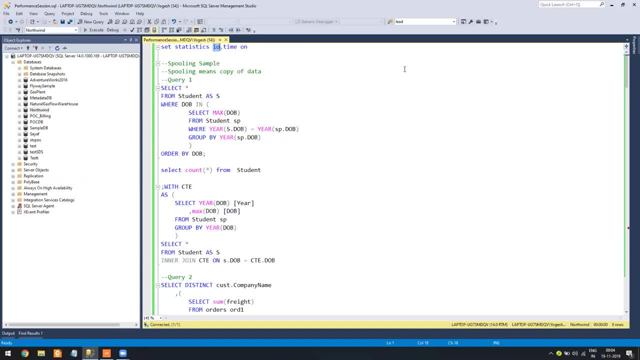 and now I optimize the query. and I said so still. the time is like less than one second and still I am able to optimize that query. instead of one million reads, logically, it is doing 10,000 logical reads, Believe me, even though you don't see change in time. 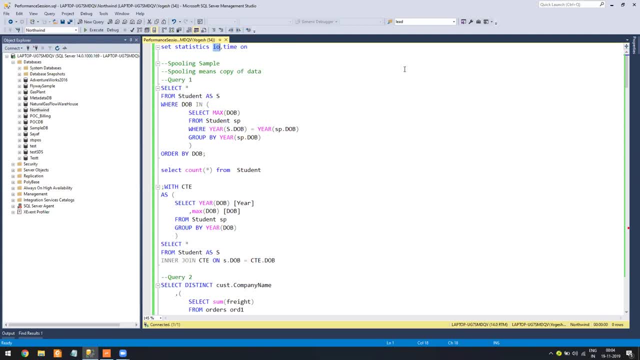 but it will be far better for your server, because now you can run 100 queries in parallel, because still they won't be able to make one million reads, Okay. So let's start with a practical example. So first is I will turn on this set: 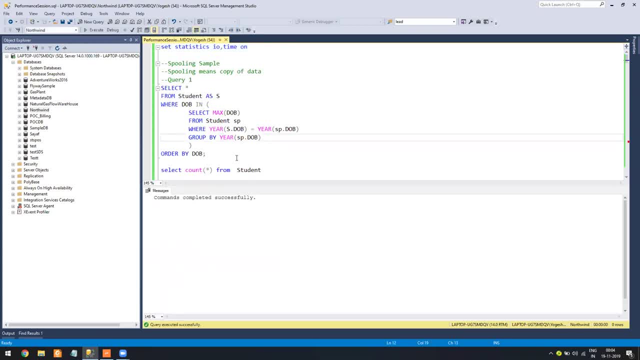 statistics: IO on IO and time on. and I will run this query. It will take a bit to complete. Let it run and you don't have to see in the query what it is doing. First is like what is wrong with the query? Let's focus on that. 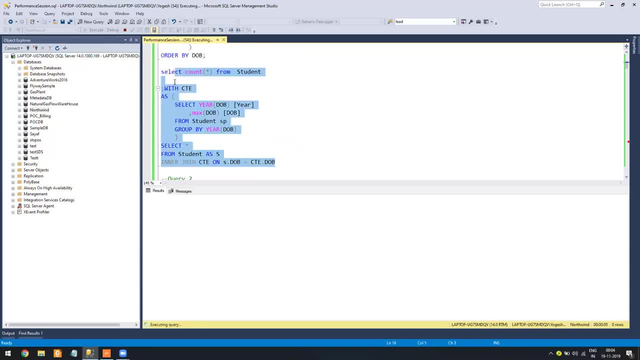 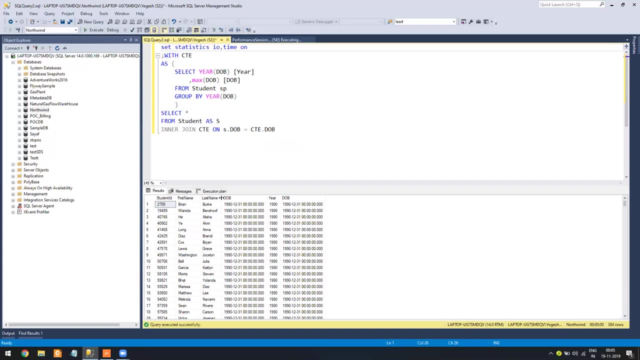 and this is the second query, which is the second version of the same. Let me just put into other tab, run the set statistics time on time and IO on here as well and run this query Now. this query just ran in a fraction of second Now. 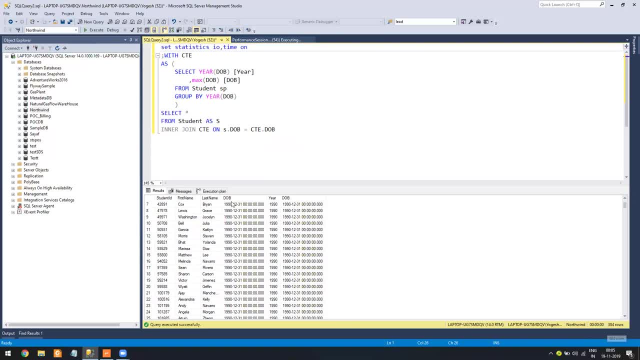 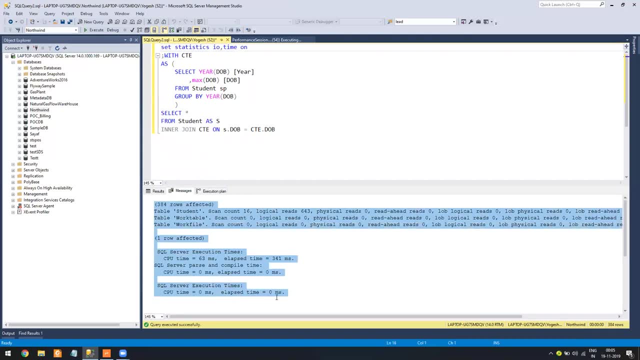 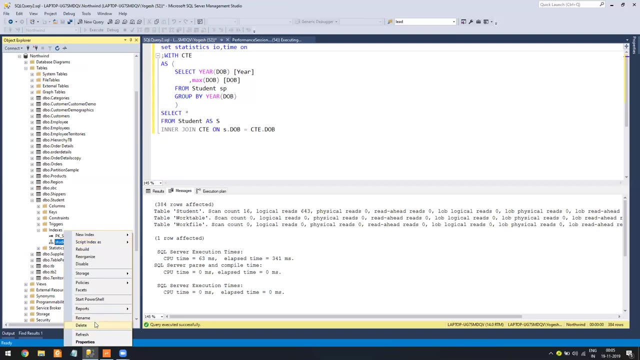 the total number of recorded gave me 384, and this is a very simple execution plan and if I see these are the statistics I got, Okay, Let me just drop one index, because that I will be covering in next session also, like in this video. So let me just 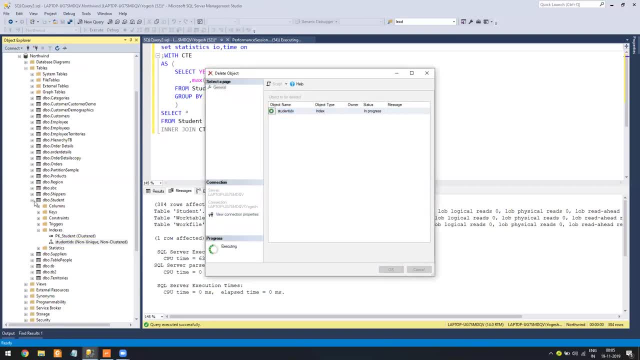 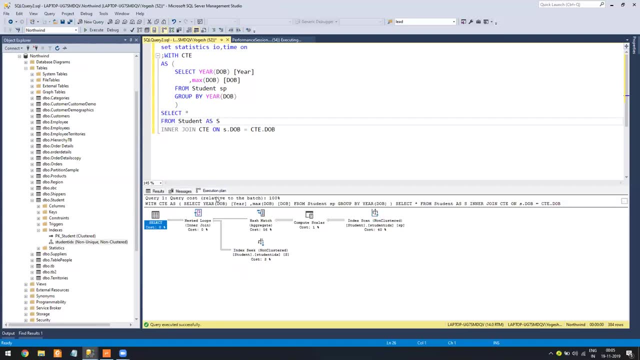 drop that and see the performance without an index. Okay, Let me just run this query again. So again, it is taking less than one second. The execution plan still haven't dropped the index. That's crazy, But that's my time. 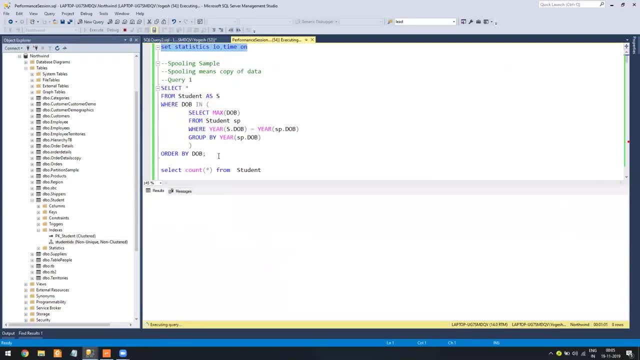 Okay, Oh, I think this query is running. That's why Let me, Okay, Let it run. Let it run the query because it's in the use and also, like this query I am running, It's still executing. and let me show you my SQL Server. 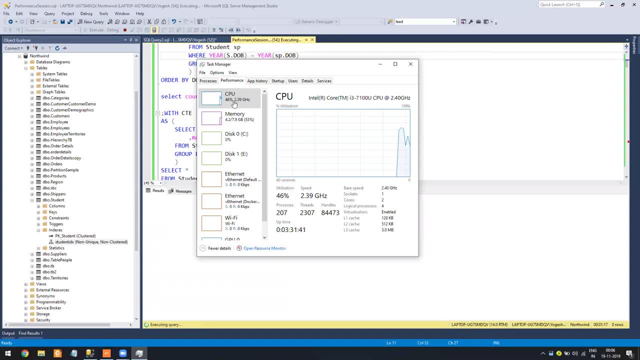 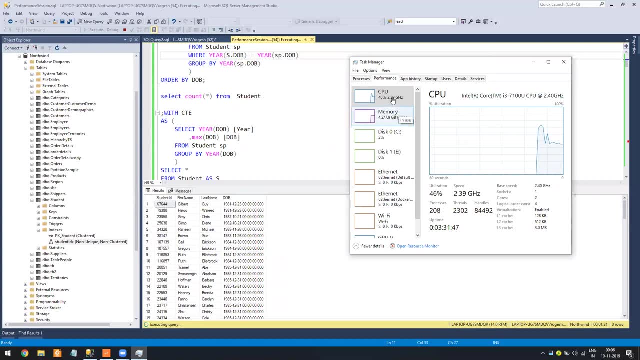 performance, like my system performance. Here you see the CPU is going high and see now the query is giving the data, Let it complete and you see a certain drop in my CPU usage as well. And this is one single query. My system is 8GB RAM. 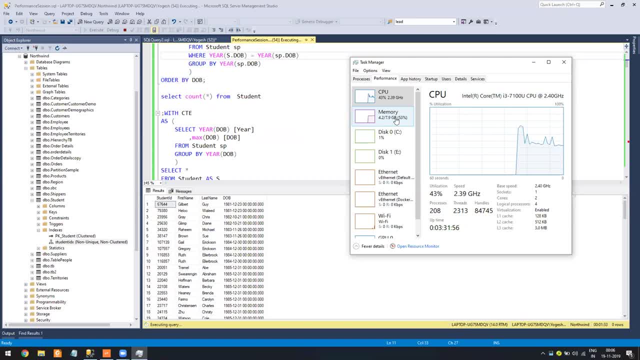 with i3 processors, So just one query can make it go high. Okay, Let it complete. It will take a minute or two. Just bear with me, Sorry, I want to show you and this is the only query, which will be longer. After that, you will understand. 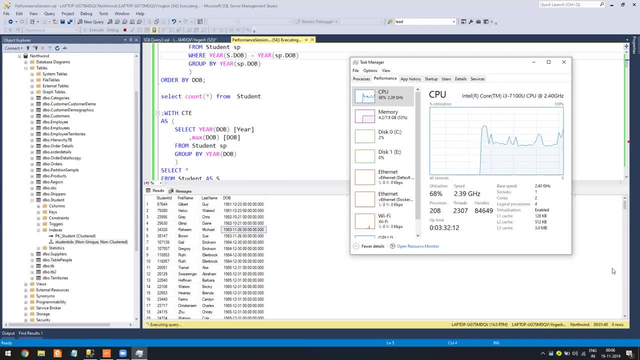 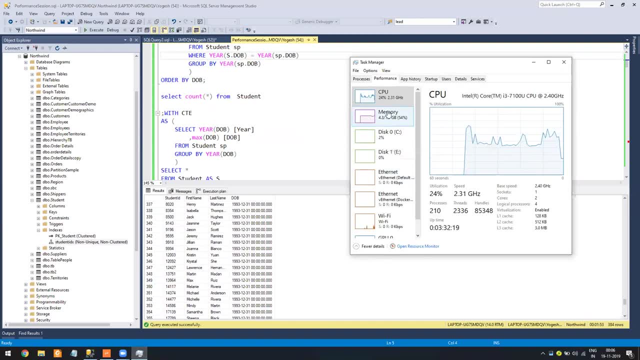 even I just give you a hint like this is bad. We are coming nearby. So now the query is complete and you see the CPU usage Now it was between like 47 to 56. Now it is just back to 20.. 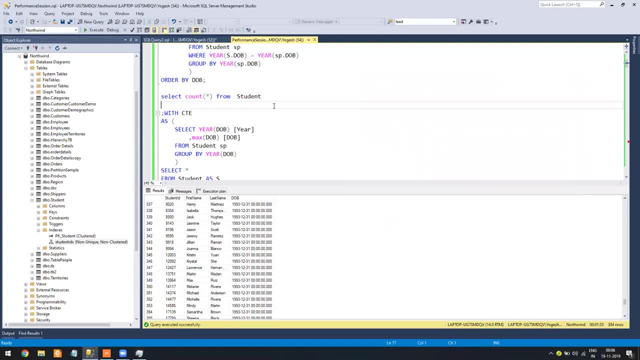 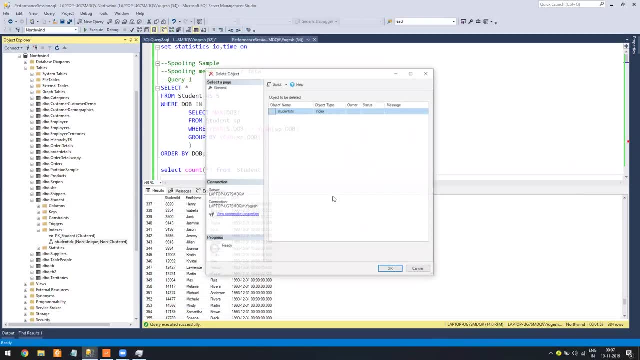 You can see a certain drop in CPU just with one query. Okay, Now let's see what is happening in this query. Let me just drop this index again. so that query was using the index, So let me just drop it. It won't take that much time and 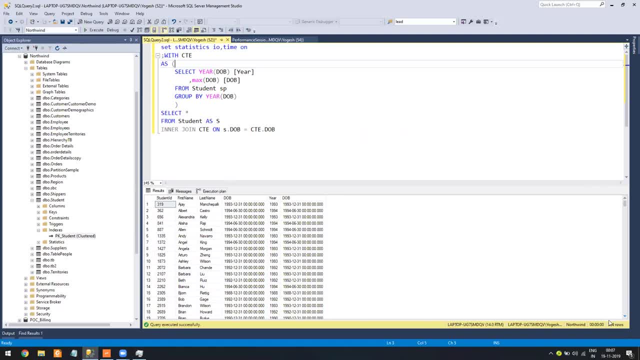 rerun this query. So here see the output: 384 records. Here the output: 384 records How much time taken: 1.53. seconds, and here it's less than a second. If I see the execution plan, it's a simple execution. 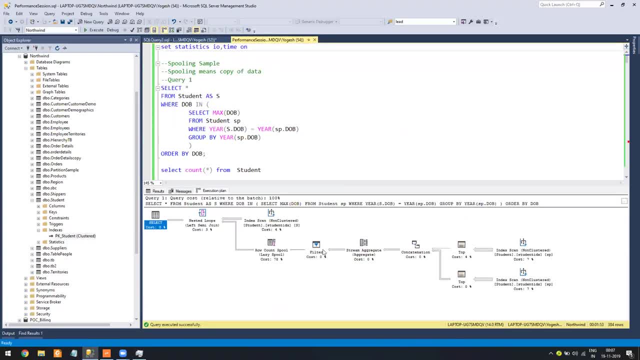 plan, and if I see the execution plan in here, it's kind of little bit bigger, Okay, So now we will break down the execution plan in multiple things, but first let us see how to analyze the statistics, because now here I am, running this query, I am 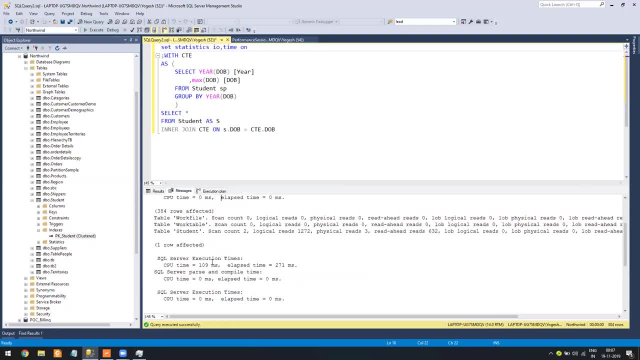 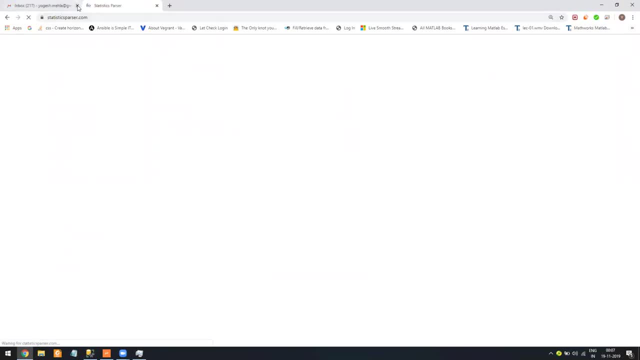 suppose there is a thousand table involved. So this statistics will not be that small, It will be very big. So how you will analyze it? You have to go in one website called statistics parser. It's very good website, It's free to use. 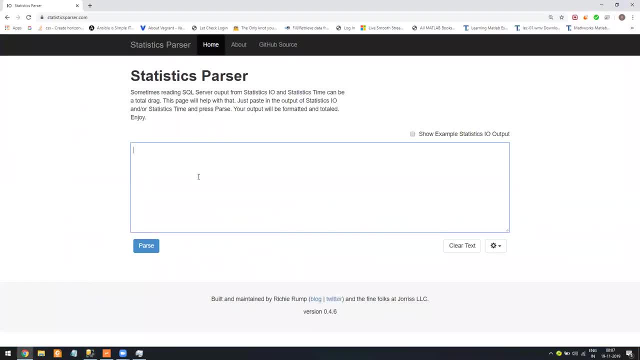 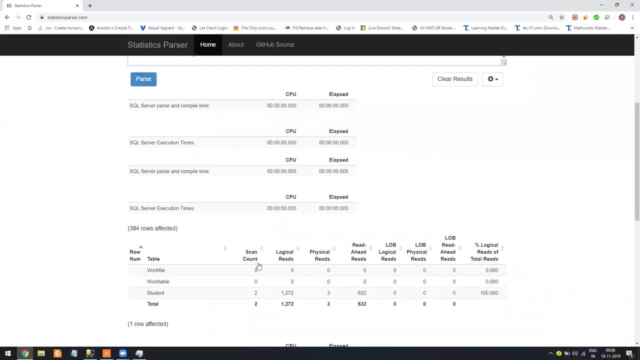 What you have to do is you just have to copy your statistics, paste it here and click on parse So it will give you a more readable format, like how much logical reads. You can see the scan logical reads. So this student table has 2 scan and 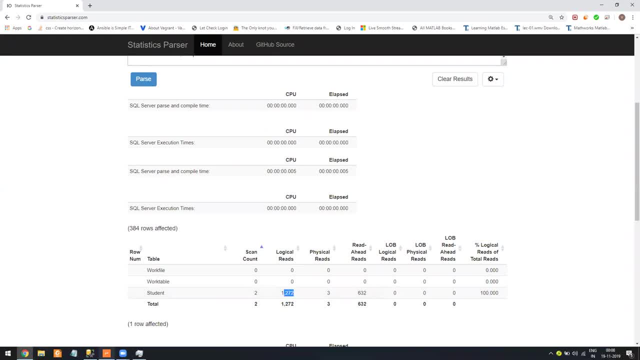 1200 logical reads, and so on and so on. And now let us have a copy from the other query, which was taking more time, and let's see what its statistics says. Let me just paste it and click on parse. Now, here you see, how many logical 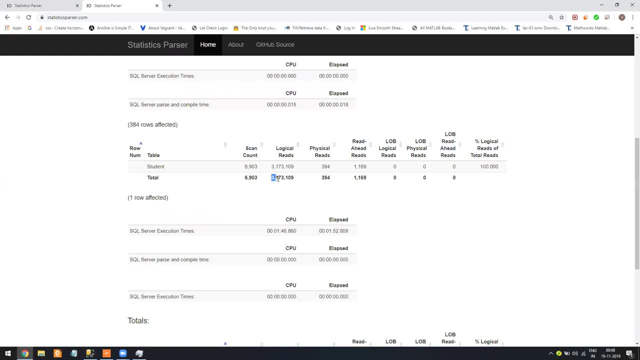 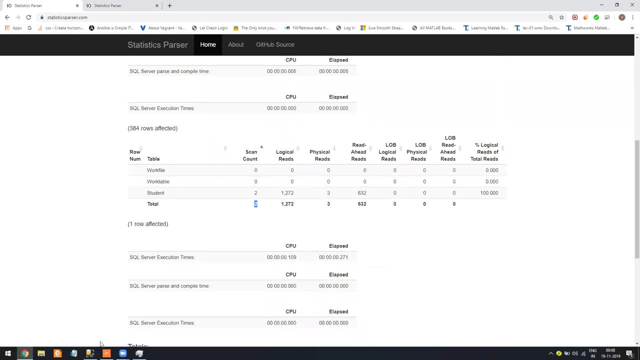 reads I am doing: Scan is like 6900 and the logical read is like 7 digits. And here the logical read is 4 digit and the scan is 1 digit. And the thing is the irony is both has the same data. 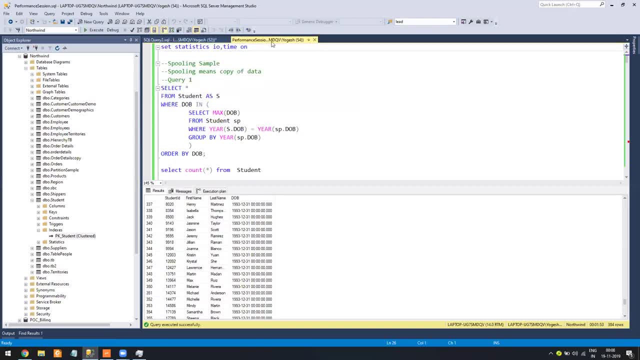 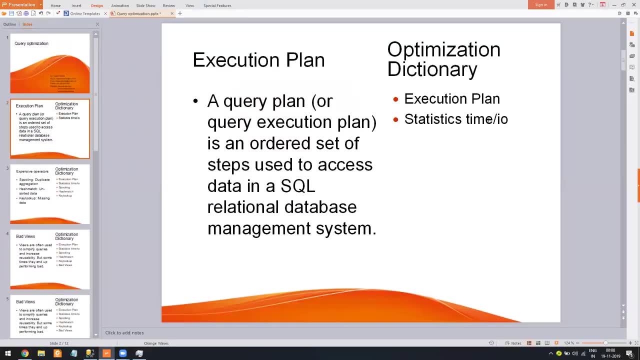 384 records, and 384 records Less than, once again, almost near to 2000.. Now, what is the difference? Let's see the execution plan, and here your first lesson will come. One is using statistics, time and IO on to determine which query. 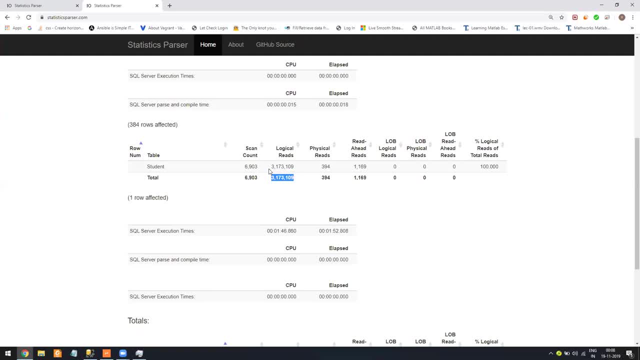 is expensive and which is not, which is based on the logical read and physical read. Usually physical read doesn't matter a lot because a lot of times they- if you are reading first time the data, it may have a physical read, But logical read matter a lot if it. 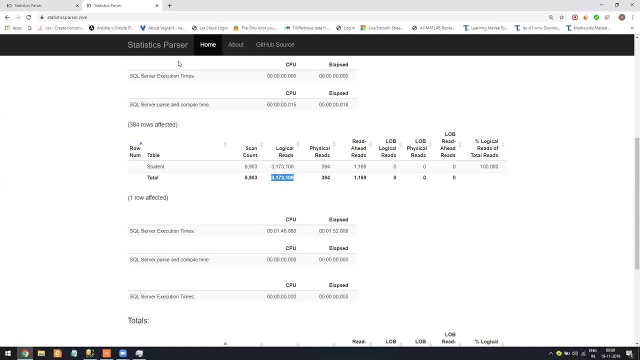 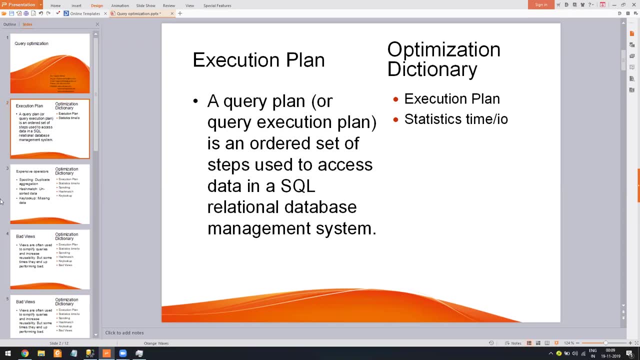 is more, means every time your query has to do a lot of input, output in the memory. So first thing is statistics, IO time, UNC and seeing the execution plan Now what we will look into. the execution plan Now. this first example is: 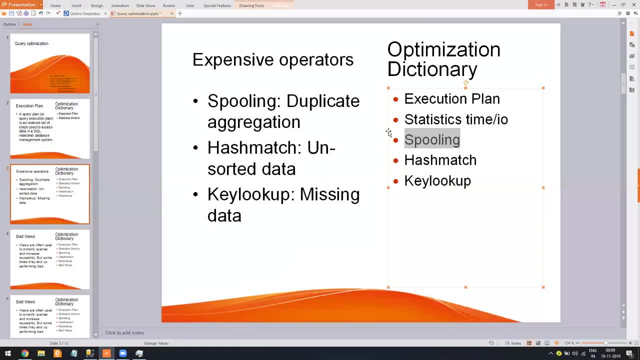 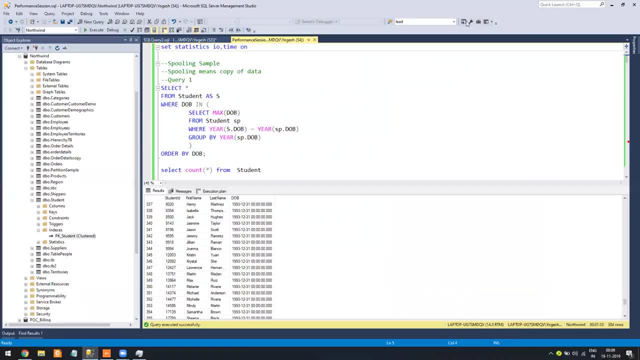 for spooling, So there is something called as lazy spool. There are multiple types of spooling. One is lazy spool. Whenever you see an execution plan, let me just hide my icon. sorry, there are so many icons. 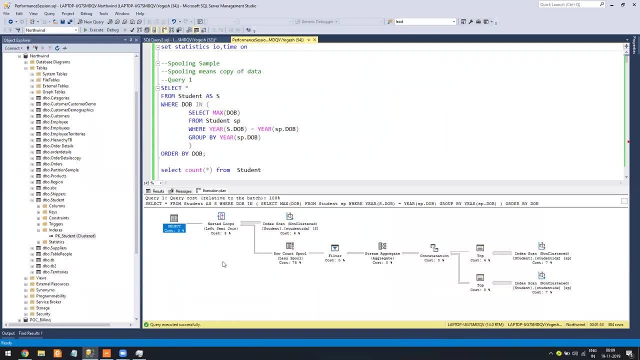 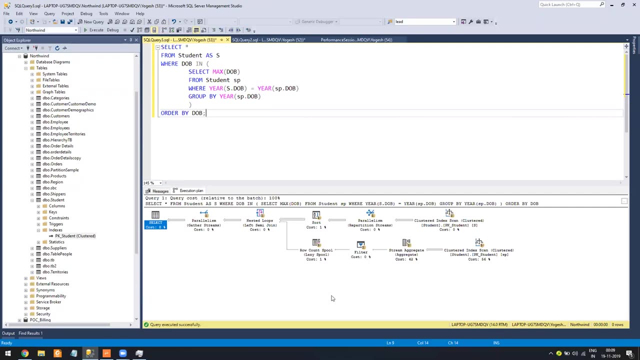 So, whenever you see an execution plan and contain any operator called lazy spool, believe me, that is the problem. So now, if I just do, let me do one thing, because there was index use, so that's why it is different. Now let me just get. 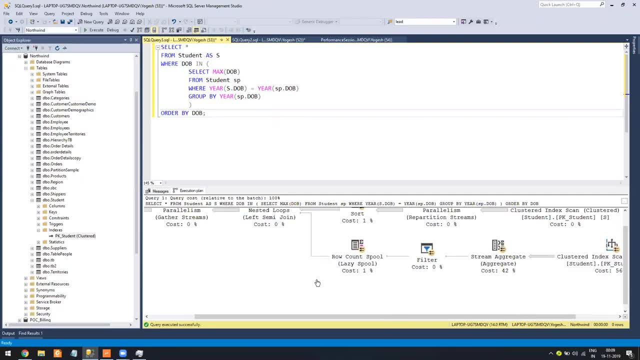 So here, execution plan. Now, here you see, there is a lazy spool which says 1% of the total cost of this execution plan. Now why lazy spool is bad? See, it says 1%, but if you see after it it says 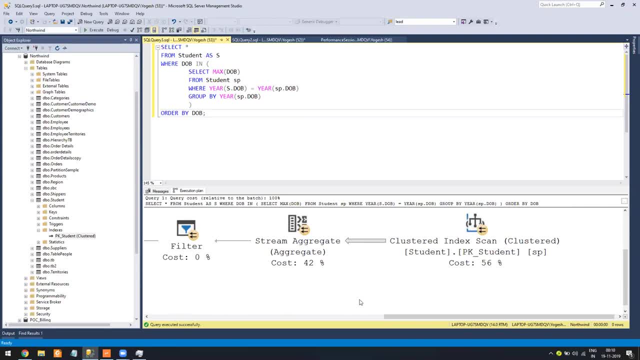 98% of the total cost is spent In this part of your execution plan, plus one which is 99%. So 99% of your query performance is happening in this part, Just this part. So whenever you see a lazy spool, 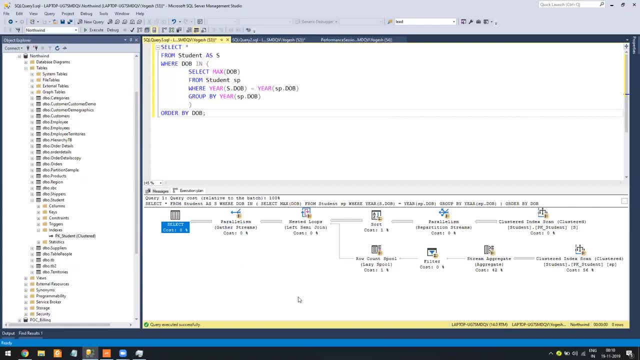 this is the most expensive operator in total SQL Server. So whenever you see a 1000 line or 200 line execution plan, just see the part where it is doing a lazy spool, See the things which is happening after that 1% and then. 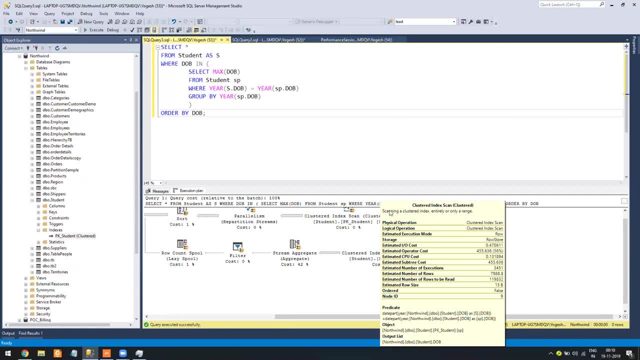 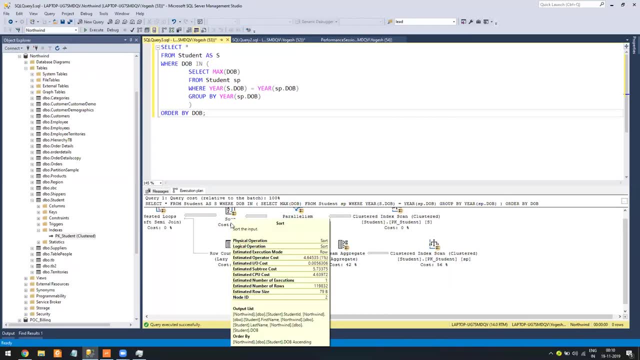 try to figure it out. how to fix it Now. how to fix it comes with how. why it comes Now. lazy spool is not bad in a way. Why it is not a bad. It is meant for solving a problem, But the problem is when there is no. 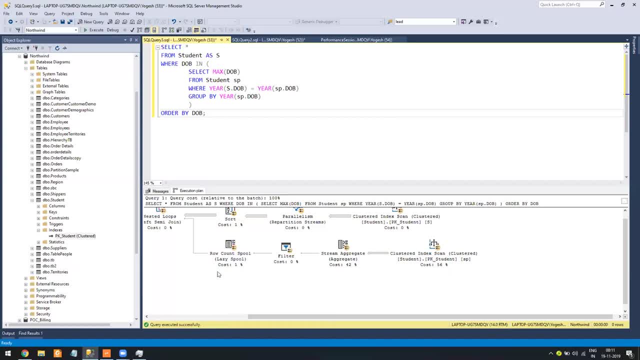 problem and we are telling SQL Server to solve it. Now lazy spool comes when there is a duplicate aggregation. Aggregation is group by some minimum, maximum or any of those kind of operators. Whenever there is a duplicate aggregation happening, a lazy spool will come. 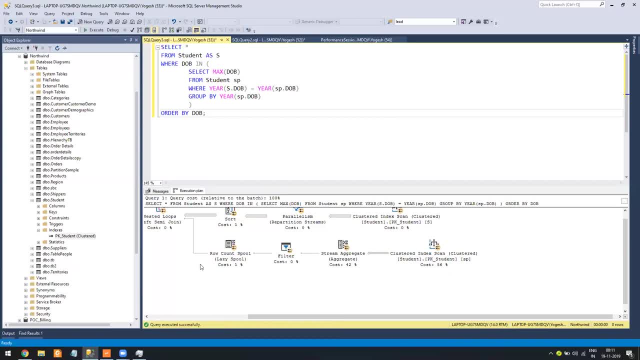 So why are my queries doing duplicate aggregation? If I can fix it without doing a duplicate aggregation, then I am good. So here, if you see the query, what I am doing is I am selecting my students and from the student I am getting their year, when they were born and in. 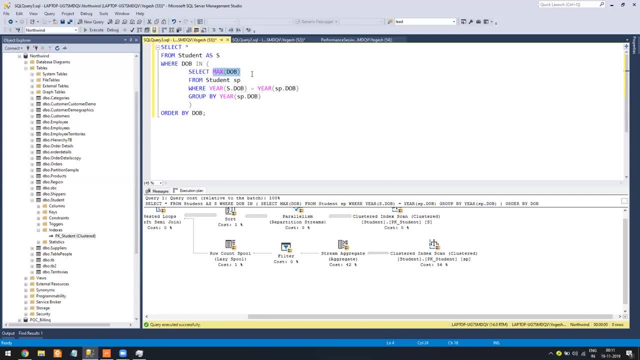 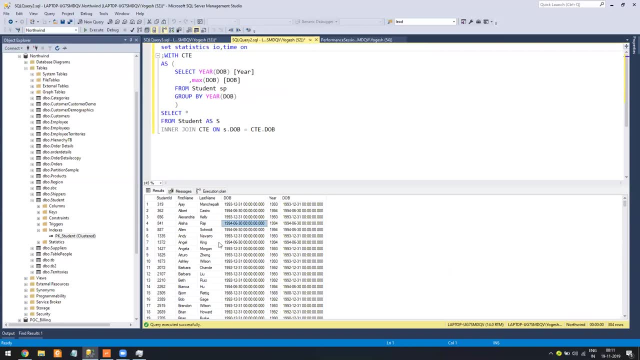 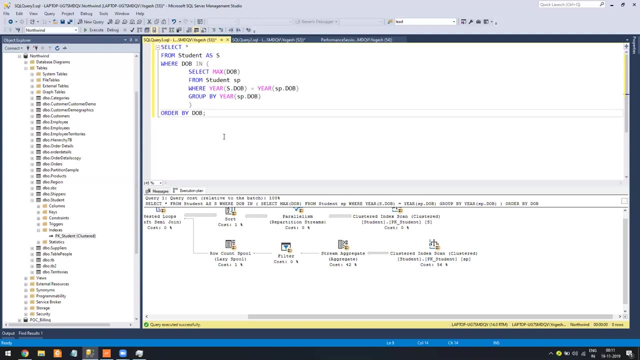 that year. what was the most? you can say who was the most youngest student of that year. get me that record. So 384 are the most youngest student from each and every year. That's how I am getting the data. So one year can have multiple people with the same. 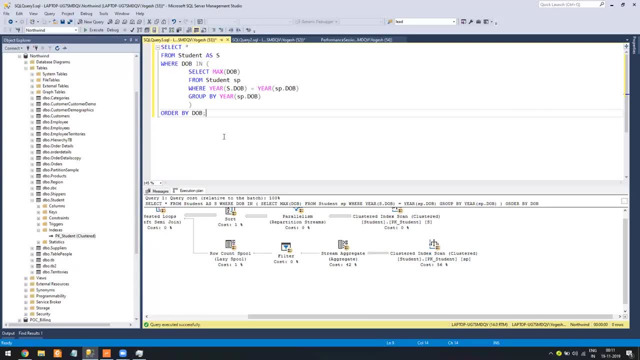 date, which are the most youngest, like all people born on 31st December. So they will be youngest among all. So those kind of things. But what happens is for each student- suppose I have 1 lakh students- Okay, From that 1 lakh. 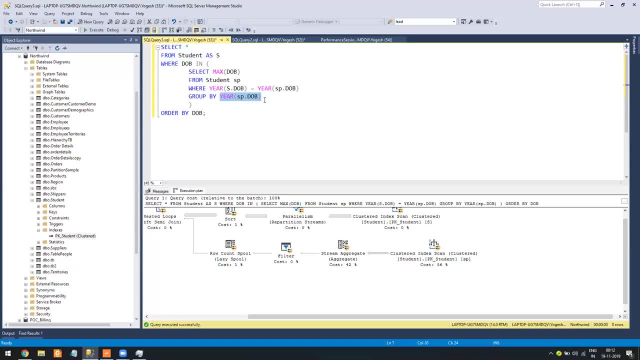 student year. they are born now. most of the students will be born in 90s, So let's say like 100.. So there will be 100 year only, for which I have to get the data, Even though there are 1 lakh. students. still there are only 100 years. So if I am getting maximum date of birth of that year, it won't change, because if you are, suppose I am born in 1991.. So suppose the most youngest child was 31st December. Now you are born. 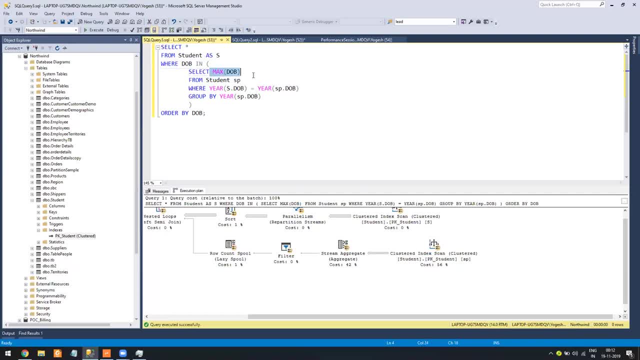 in 1991. again, the most youngest will be the same, because maximum DOB is just getting the maximum date of birth of that year, So it won't change anything, Okay. So in that terms, what happens is every year, every time I am calculating this max. 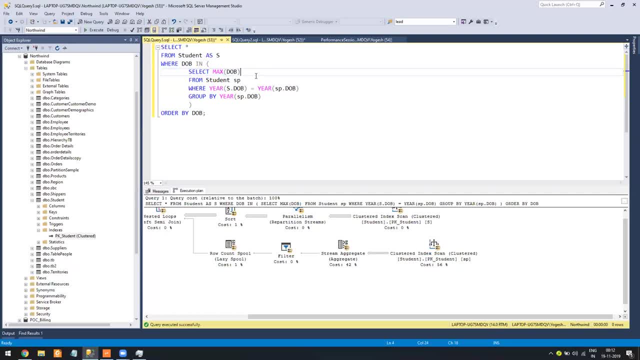 DOB. So I am doing duplicate aggregation even though it won't change. So what SQL server do is it try to maintain a spool. I will not be going in deep- why, what is spool and how it works, But the concept is. 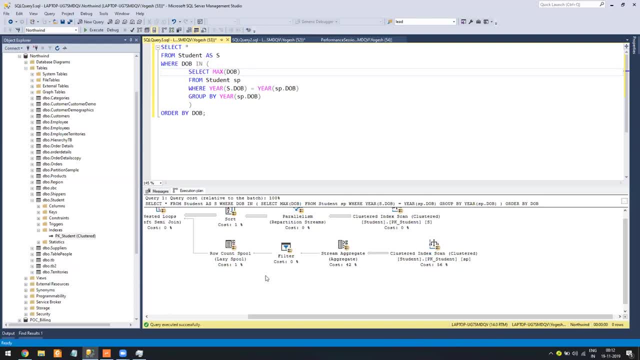 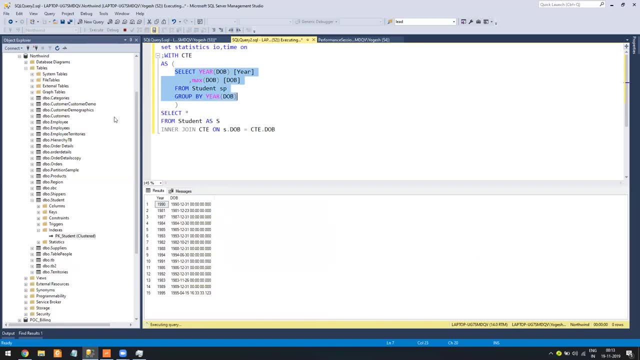 lazy spool means it's a duplicate aggregation. Now, how you can fix a duplicate aggregation Now, in this example, what I did is I calculated the year and their max DOB before even joining with the student. Once I got that, I just joined it with the student and I got my output. 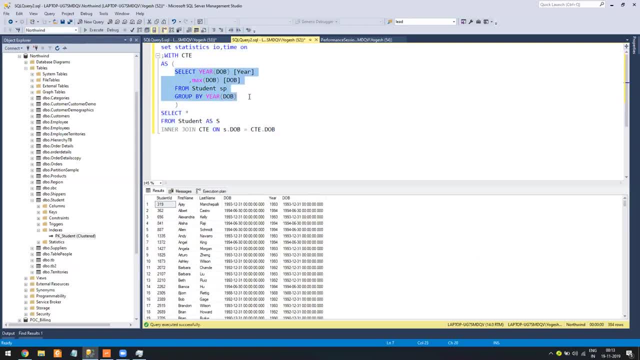 So what I did is to remove the duplicate aggregation. I just do a summary Before my query. I can use a temp table, I can use a CTO, who can use anything, So what it helps in where my logical read was sky high. 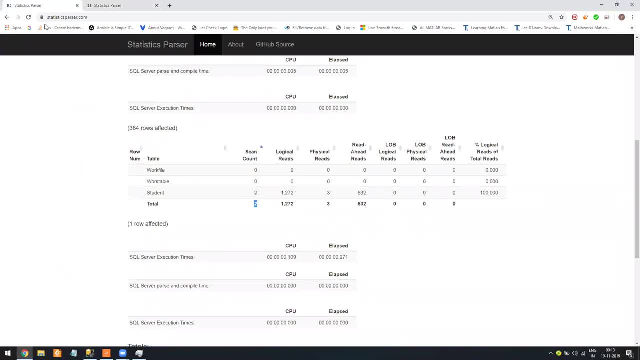 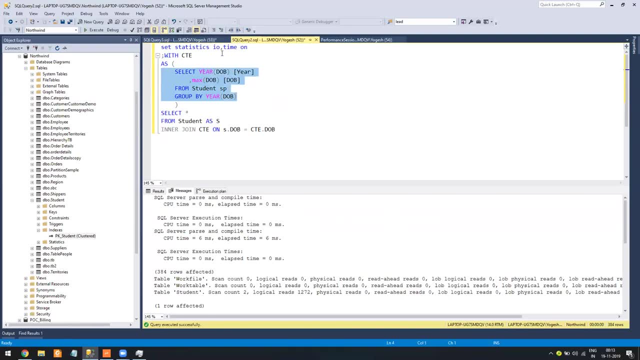 7 digit and 4 digit. The moment I did, you can say I computed my aggregation before the query, So there should not be any duplicate aggregation. The moment I did it it came to 4 digit And for sure there will be a. 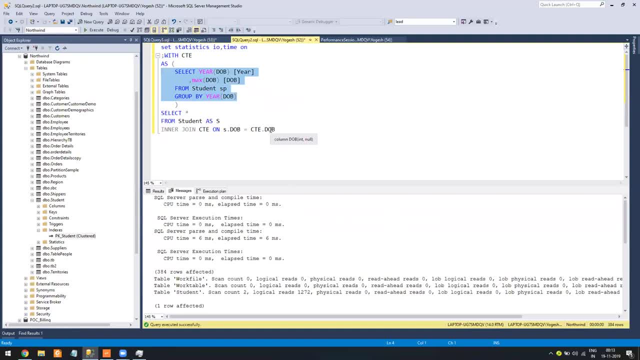 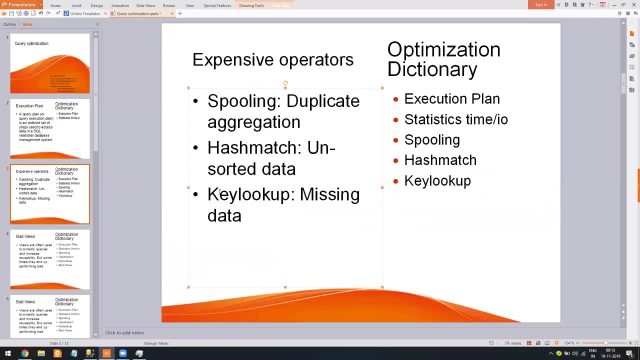 difference in the performance. That was 2 minutes and it is around less than a second, So you understood. So whenever you are seeing an execution plan, the first thing is you get the expensive query. as I told you Once you got the 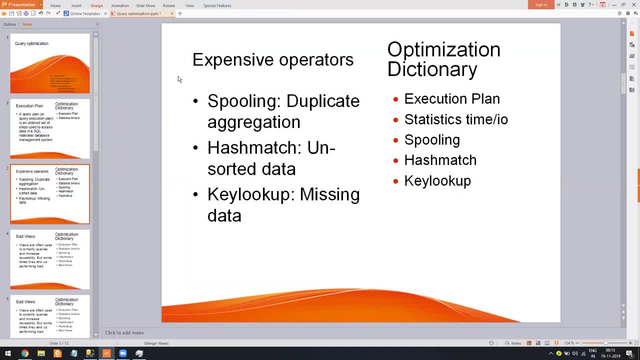 expensive query. see which query or which part of the query is having lazy spool and try to fix that before, because that's almost very easy to solve. Because most of the time it's always because of duplicate aggregation, which you can fix by using table PP or 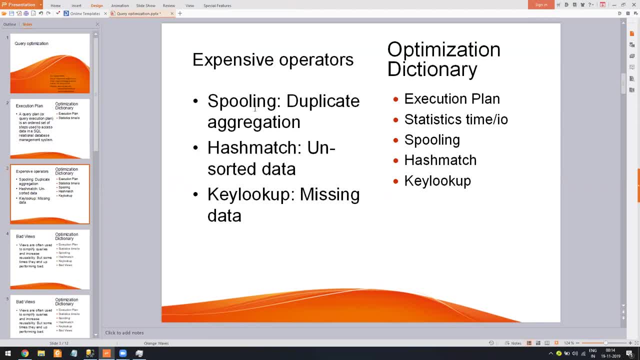 whatever you want to do, That's the one thing. So spooling means duplicate aggregation, So you don't have to remember all the things, what I will take. So by the end of the you can say: I will give you this list. 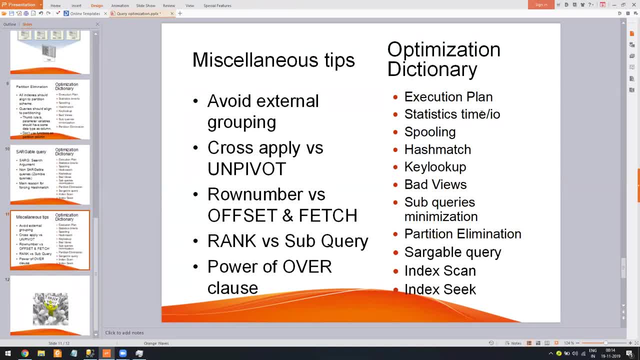 You just need to remember: If there is a spooling in any part of the query, try to fix it before, because that will have your massive change. Here you can see 2 minutes to 1 second, So it's almost like. 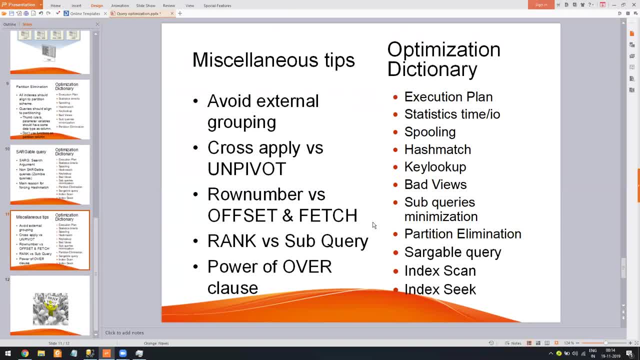 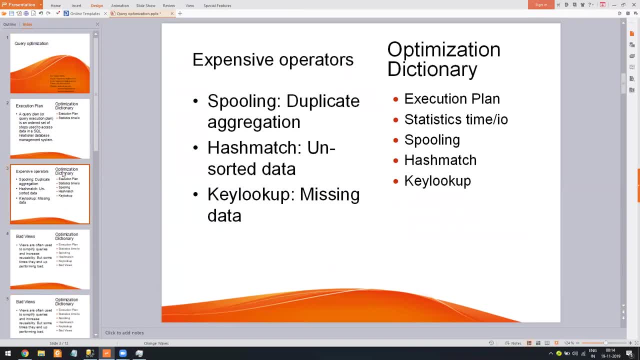 200 times. the change was there. So that is one thing. and then, after this, you will see the hash match. Let's say: what is hash match? Hash match is nothing but an unsorted data. Now suppose you are. first you have to see the spooling. 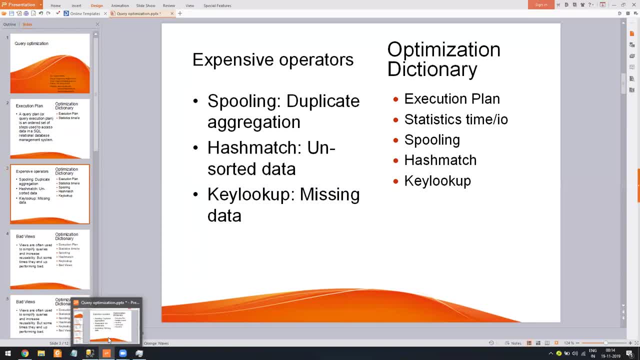 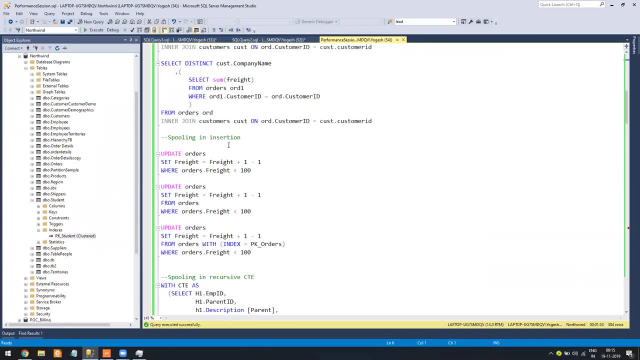 Second, you have to see hash match. Let's discuss more on spooling. Let me cover few more examples so that you can understand. Now is all spooling wrong. No, So here, what I did is I just created an update statement. 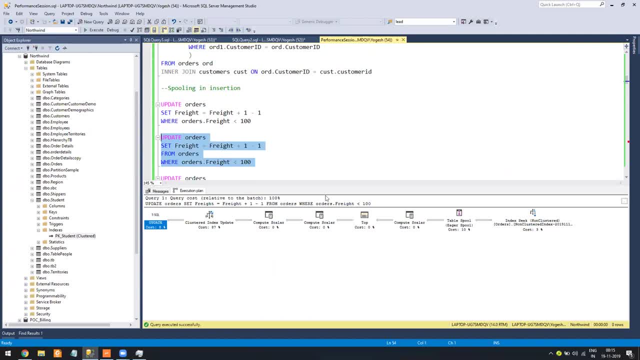 and I have an index on this: fright. Fright is nothing but a total. So what here my execution plan is doing? it is using in just an update statement. there is no join happening, there is no grouping happening, And what is eager spooling? It's nothing. 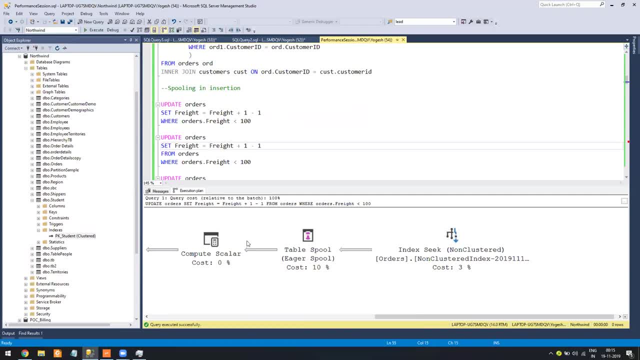 as I told you, there is a spooling involved. Spooling is nothing but a temporary saving of data to make a compute easy. So why there is a spooling involved in just a simple update? because what happened? your table has a lot of records and 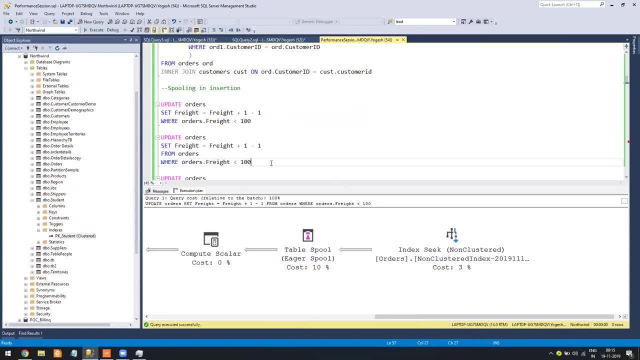 there is an index on this fright when I am running. So first SQL, what it is doing is trying to filter it out, all the records, which is having this condition true, and then putting into a temporary location and then taking those records and going into the physical table and updating. 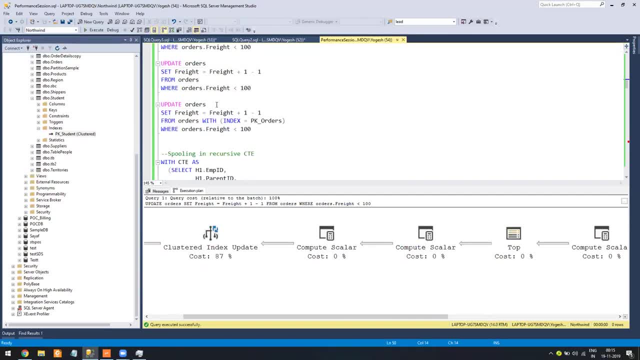 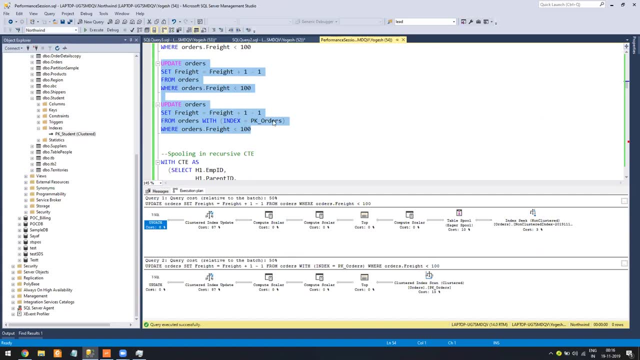 them. That's how it is working. So what happens is: spooling is never always bad, So this is one more way of doing. is now even? you see, if I force it to use primary index, it still say that 50-50% is the cost. 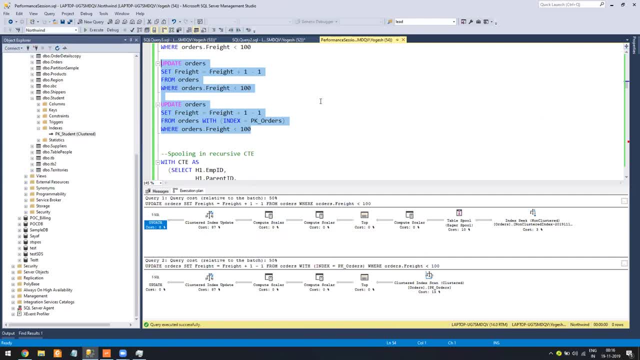 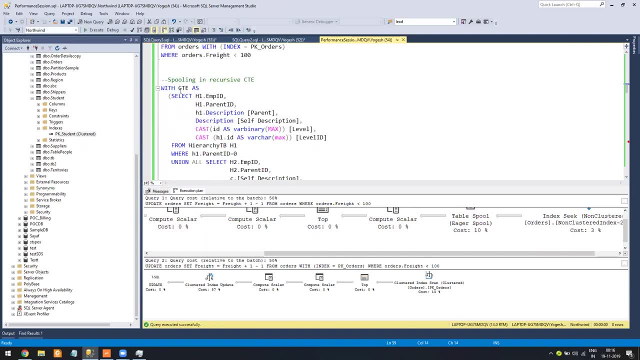 but still, in a lot of the cases, when you have a huge table, eager spooling will be helpful. So spooling is never bad, but lazy spool is a bad. Okay, One more example: where are the cases where you cannot avoid a spooling? 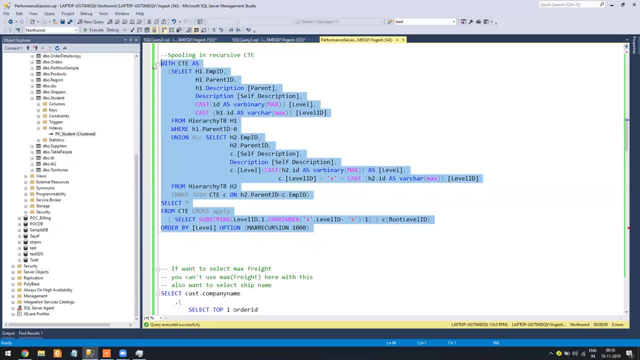 Now I created a query. I am not going into depth of this query. This query is getting me a hierarchical data. Hierarchical data is nothing, but like you have an employee, you have a manager. that manager is having certain, like again, sub-employees. 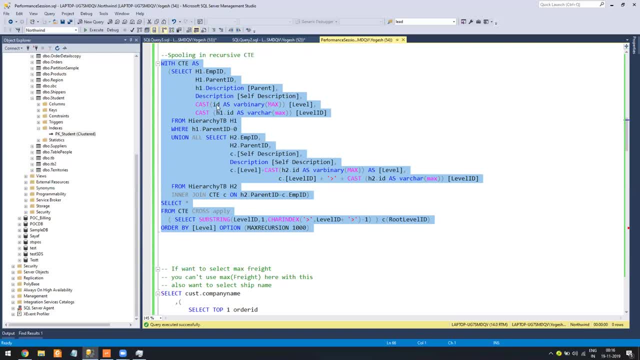 those sub-employee can be manager of other people and so on. So it's like, like you say, multi-level MLM, multi-level marketing kind of structure. So suppose you want to get all the hierarchy who works under whom? in that case you have to write a recursive CTE. 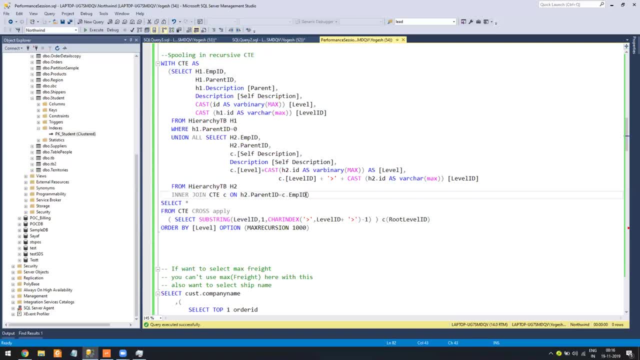 If you are very familiar with recursive CTE, then it's okay. else you can watch my CTE video, which is already there. Okay, Come back to this. So I am writing a recursive CTE Now. if I run my query, you will see a lazy spool happening. 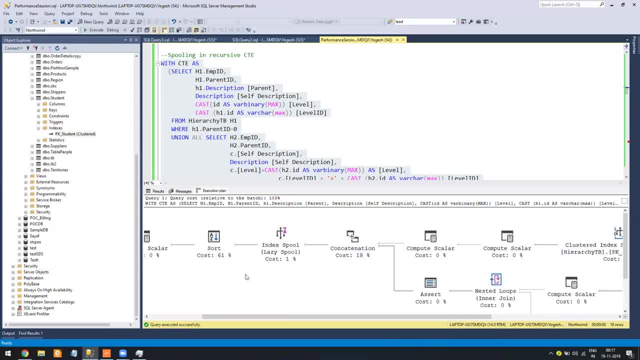 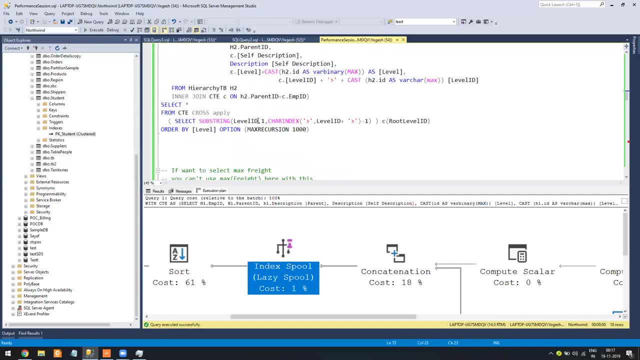 Here you see, You see a lazy spool happening Now, in this case you cannot avoid. Why? Why you cannot avoid? Here there is no aggregation happening, but there is a recursion. So recursion, in that case lazy spool will come and you cannot avoid it. 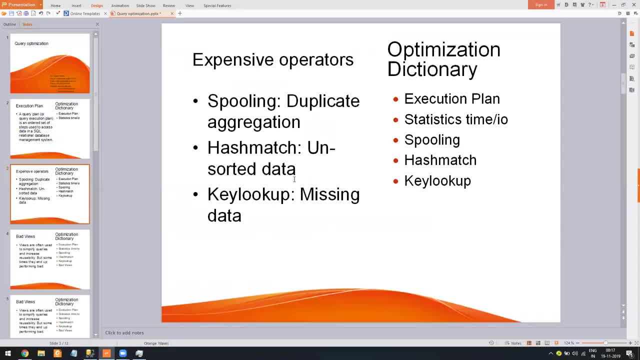 So first thing is you try to find a query which are expensive. Second, is there any spooling? If there isn't spooling, whether it's because of recursive query. If it is because of recursive query, just ignore it. If it is not, 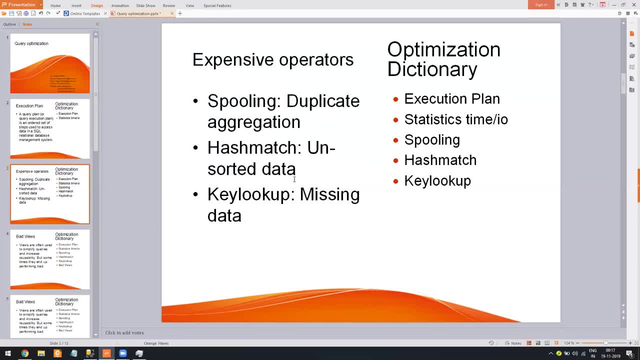 because of recursive query, it is because of duplicate aggregation. then try to fix it Okay. Once you do it, your query will be half resolved. Then, coming to the hash match Now, hash match is nothing but an unsorted data. Now what do you mean? 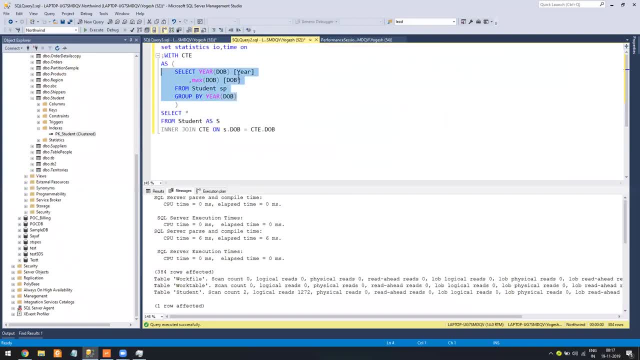 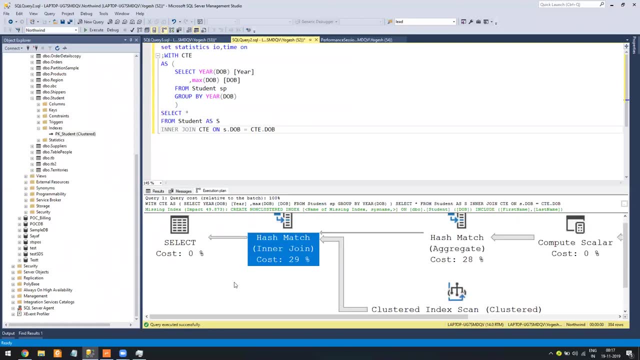 by unsorted data. Now, in my this query, when I am seeing and running, I am let's see the execution plan. So here you see, a hash match, Am I right? What is this hash match? What is happening is when I am calculating, 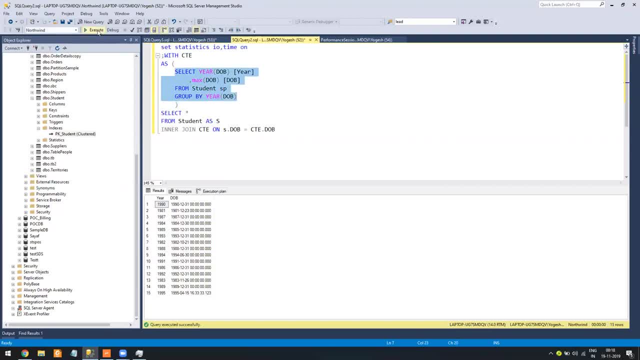 year and the maximum DOV. Now group by: why it is considered as expensive. operator Reason: group by: always includes sorting of data. So when you do an order by people say, don't order by the data if you are not required because it is expensive, But when you do. 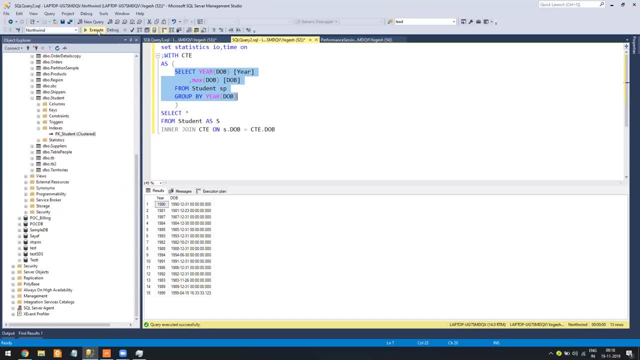 group by, it becomes order by first and then grouping. So it's always double the amount of you can say on sorting time. So first time you can say grouping data and getting their maximum, you can say DOV. Now, in this case data will be sorted. 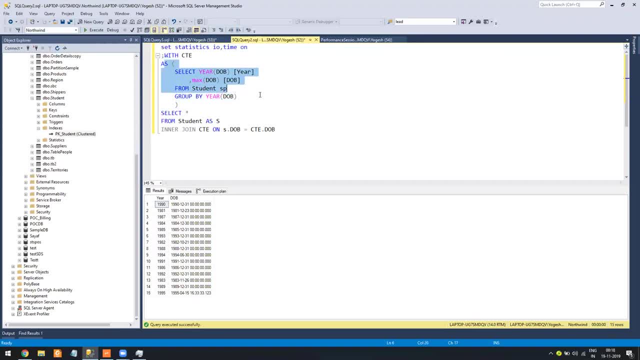 in certain way, because that's how the grouping works. Okay, Now here is the sorted data. but when I am joining with the student table on the base of date of birth, there is no index there. So student doesn't have any index on. 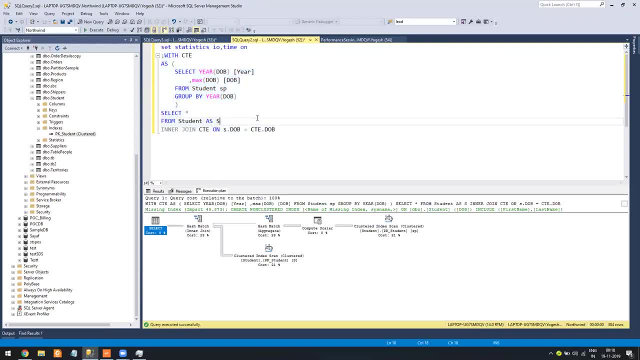 date of birth. So what SQL server has to do is it has to sort the data based on the DOV and then it has to make a join. So to do that, what it do is it calculate and hash and then make a join. So how you can resolve it? 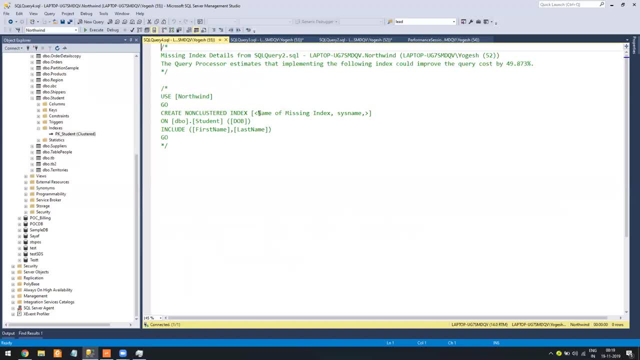 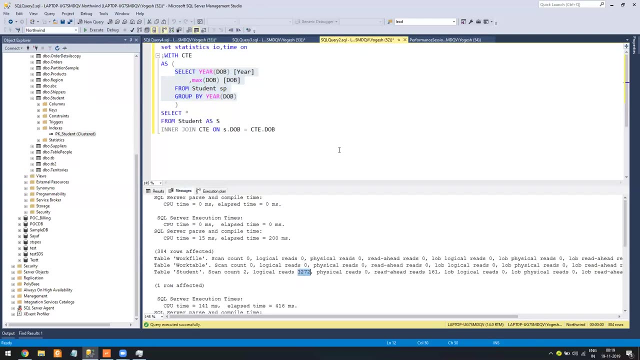 One is there is an index missing. First is first case is there is an index missing, index for student, say. and I create this index. So one more thing to remember is here. you see, my logical read was four digit. Now let us see I created the index Now. 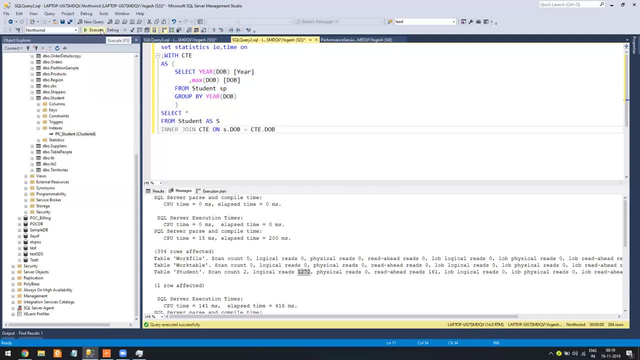 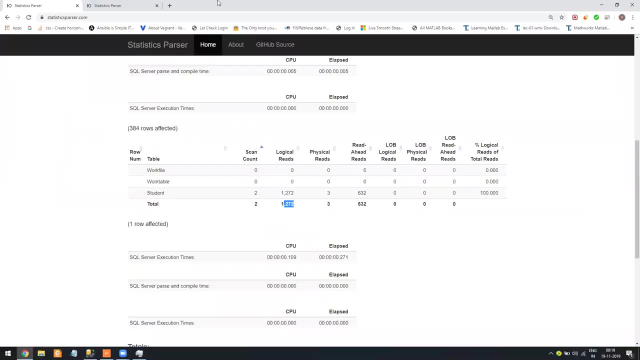 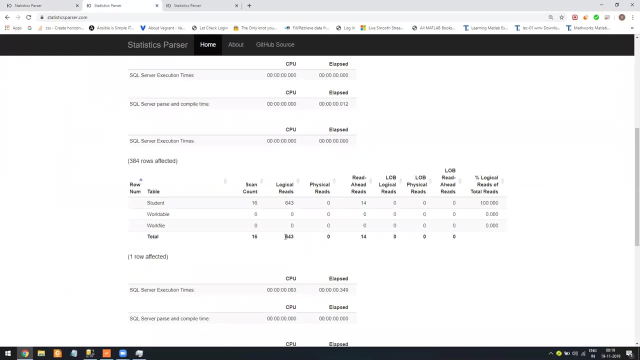 let me just close this and run my query again and see whether that brings the logical read down. So let's first see the logical reads. So this is my: after creating the index, paste it. So here my logical read is: you can say reads are reduced. 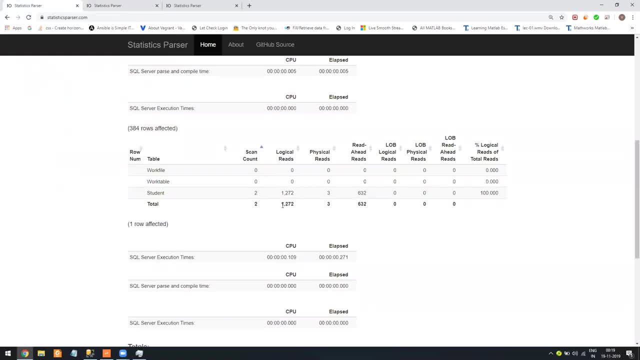 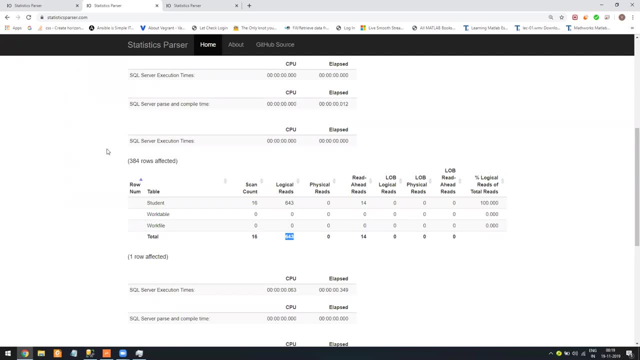 from four digit to three digit and it's almost you can say half, like 1200 to 600. so hash match has like half the advantage in our scenario and the scan or more scan are okay because the same data it has to scan. So scan you can ignore till the time. 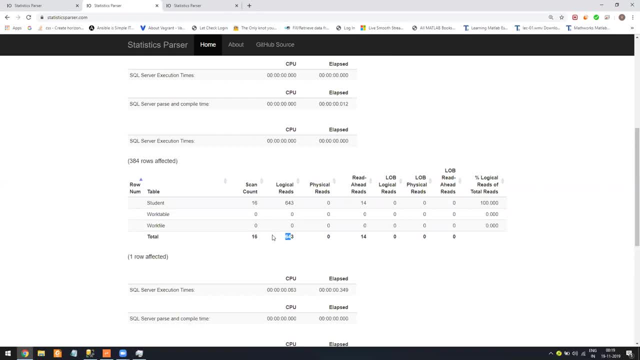 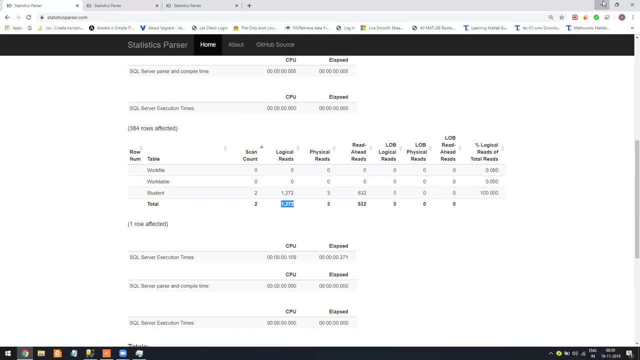 logical reads are going down Means like in. even in that way, logical reads still the scans are less. in here the logical reads are more, so scans are still less. doesn't make any sense. So now, if I see the execution plan now hash match this. 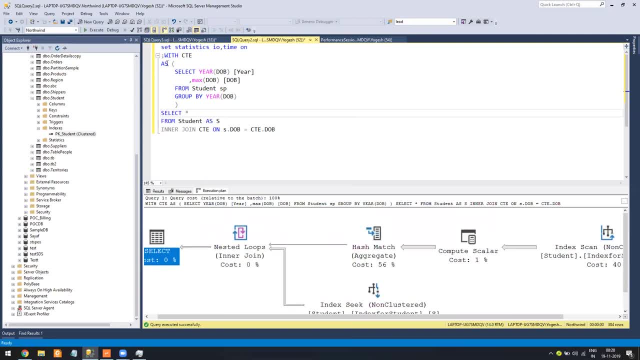 is hash match aggregation So you don't have to hash. match aggregation means it has to hash the data before doing the aggregation. So that's. but here the join got changed to nested join. The reason is: now the data is sorted. it can. it knows. 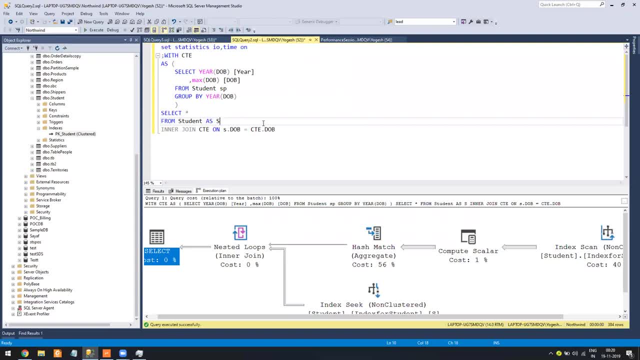 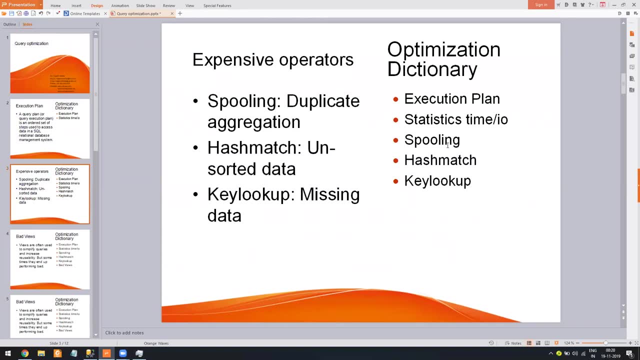 okay, how to find the data between the index, like using the index. So your after spooling hash match is your target for hash match. you have to see whether there is a missing index. that is one Second. sometimes index is already there but your query won't utilize it and 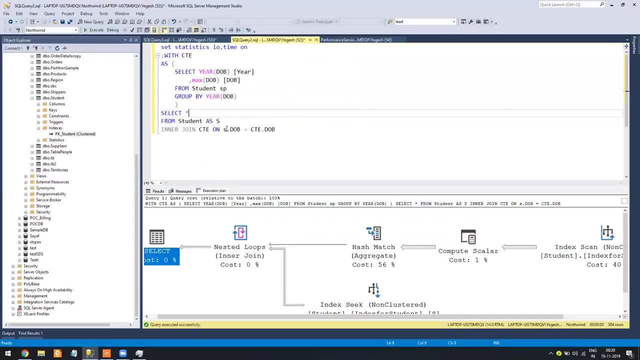 why that case comes. Let me give you a simple example. Let me add date, add, and I will say: add zero date to my date of birth. Now this is, you can say, logically wrong, but nothing has to be done like that. but I am just saying: 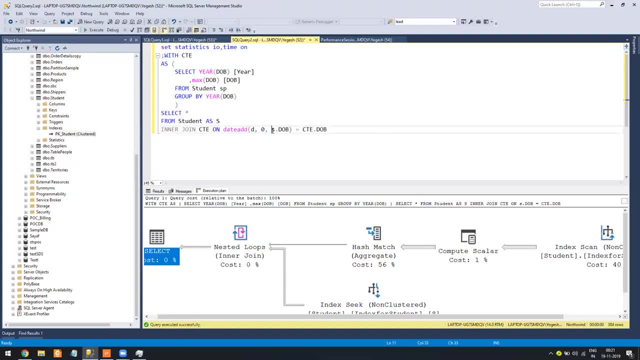 there is a function working on your date of birth, like you said: date, date, date. what I am doing is I am trying to convert my cast as date as date and I will do the same for this side cast as date, and now I run my query and see the execution plan. 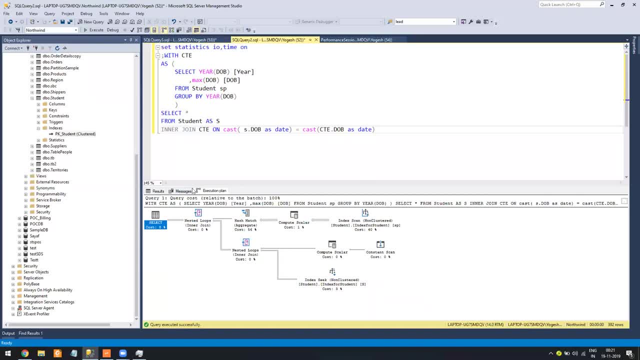 now one thing is, execution plan got increased but still hash match doesn't occur. but now what I will do is I will say date add and I will say d comma zero, just add a zero date to it, nothing else, and just remove this one. and let me just run the same query. 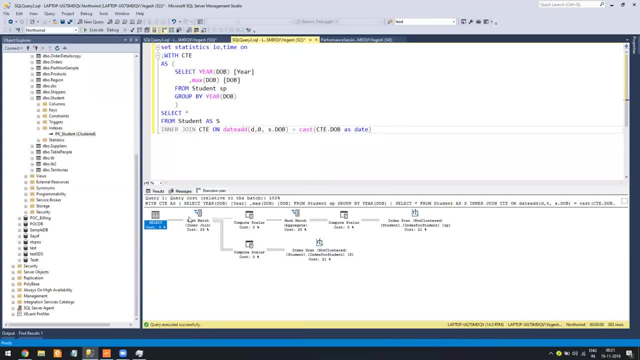 again. Output is still the same. now, here you see, hash match came again. still, index is there. but hash match came again because when I added a function on my column, now SQL Server cannot determine whether the data will be sorted or not. because there is a function means there is an output. 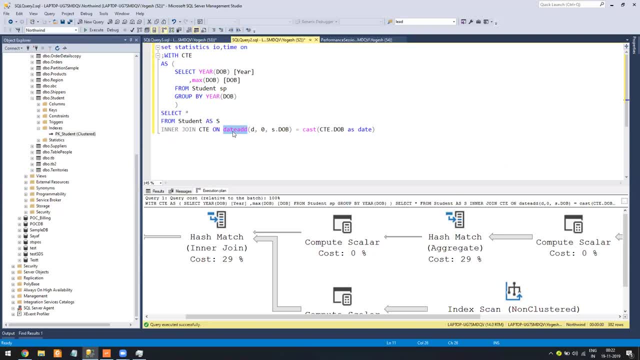 coming out of the function. so SQL Server cannot determine whether the output is a sorted output or not. so in that case SQL Server will go for hash match. so one reason is missing index. the second reason is index is there but people has used function on their columns. 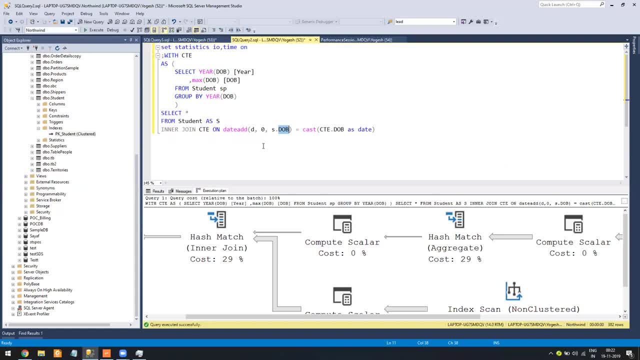 in where clause or in joins- especially this is for the join, because we are talking about hash match join. so they have used a function on a column. then first thing is you have to remove that right. another way to do that, because if there is a function, still there is an index. 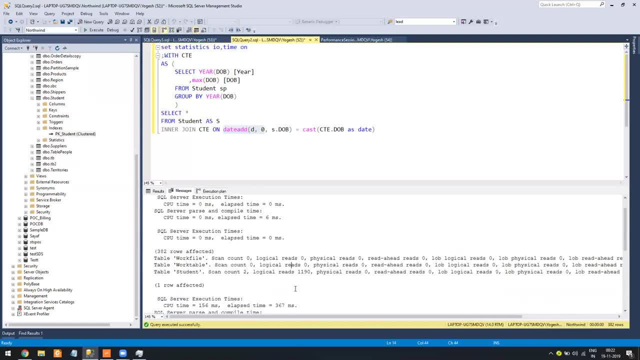 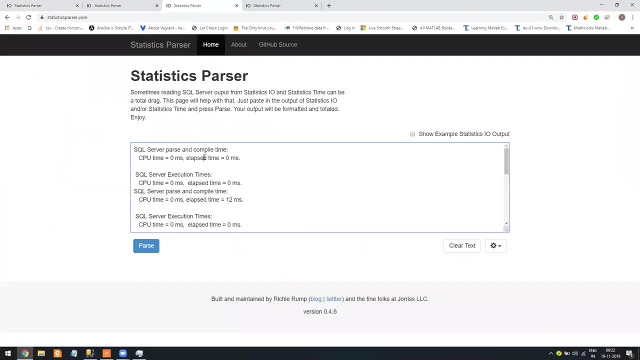 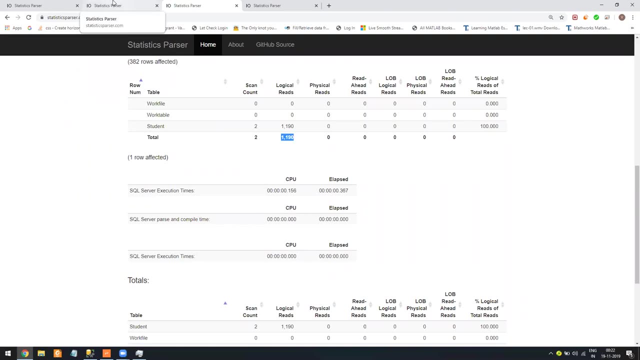 still it is going for hash match. there is no benefit of it and if you see the let's say and see the logic, read and run it. still it is less than that without indexing, but still it is more than the without like, without hash match, when the index was getting properly used. 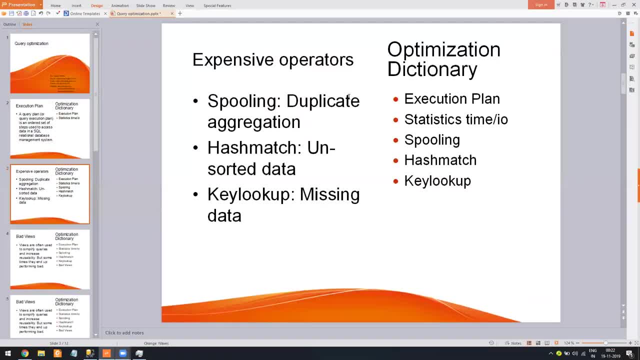 so this is the second lesson to you. first is find the queries, see spooling, see the statistics. if spooling is there, remove it. if it is because of CT like recursive CT, ignore it. if it is hash match, is there? see if there is an index: is there or not? 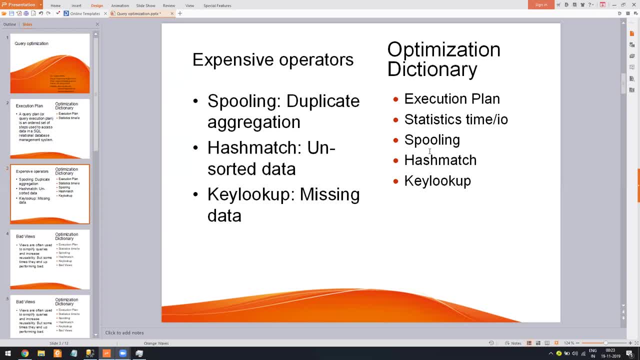 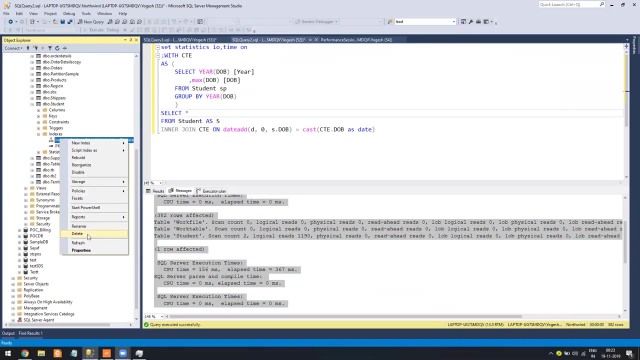 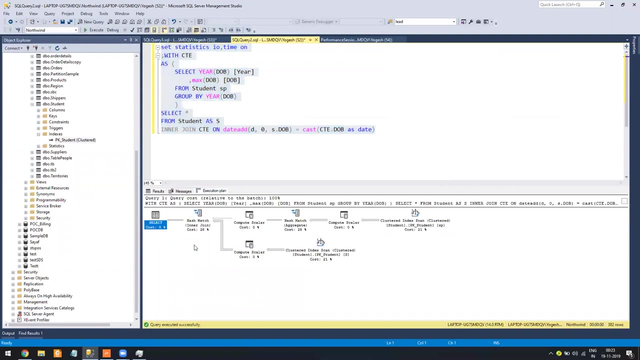 if index is not there, create an index. if index is there, then try to see why it is not getting used. okay, key lookup. I won't be covering, it's very simple, like: okay, try, let me just create. so let me run this query again now. it is not telling the 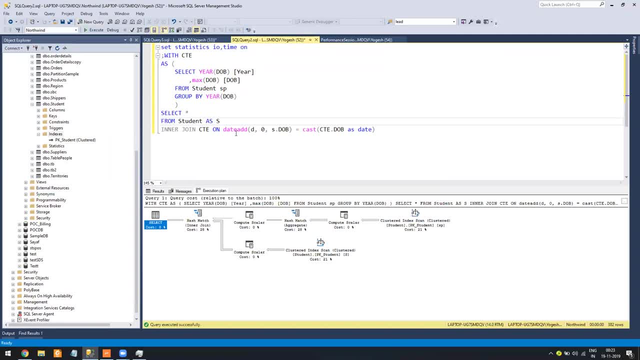 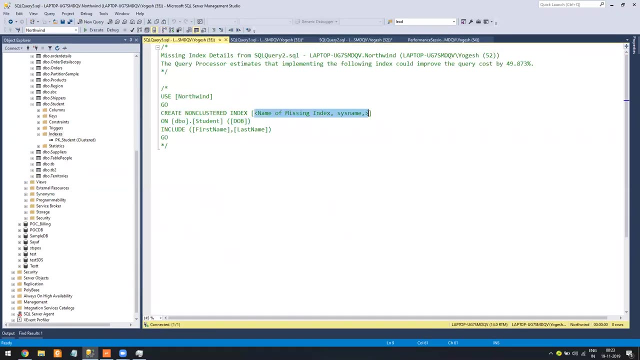 missing index. okay, let me just create an. okay because of this, again see if the hash match key lookup comes or not. but key lookup is nothing but a missing column from the index student and I will just remove the last name from the index right now. here you see. index contain index. 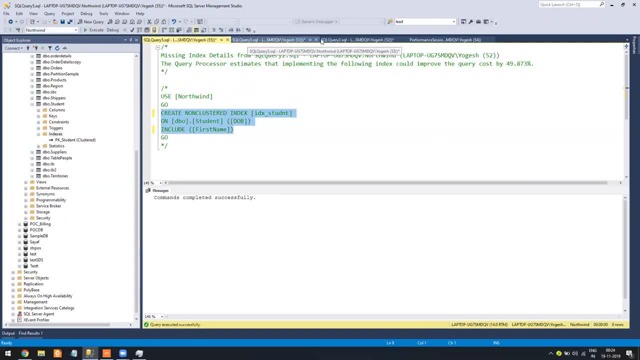 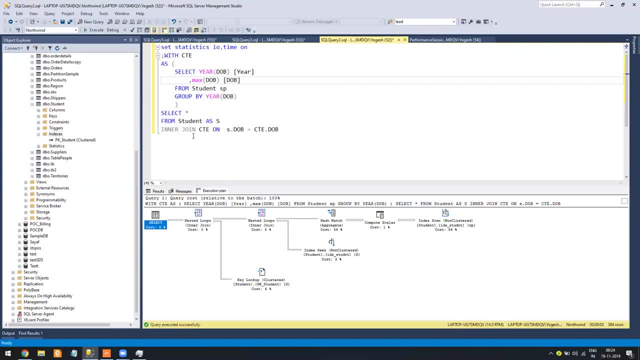 key is dob and the include is first name. and let's try to run the same query again: yep, now see what happened. is it still went to the index because it has the dob for the join. join is nested. but as my output includes star means output do contains. 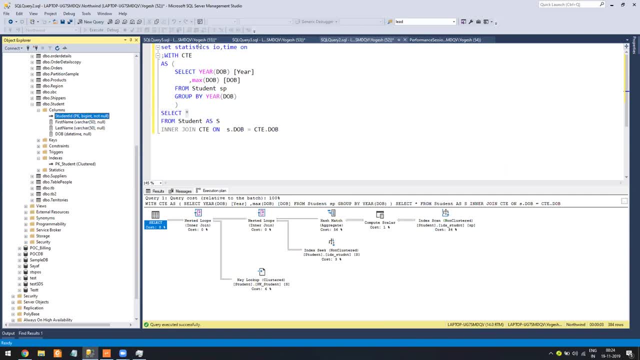 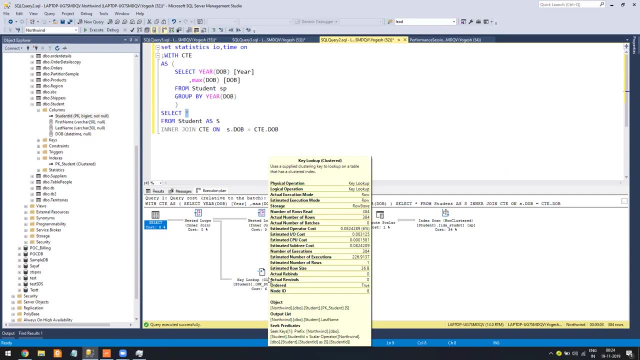 first name and last name, dob and student id. now it cannot find last name in my index so it has to again go to the table to get just one index or just one column. so this is the key lookup thing. your index is missing some column. now. solution to key lookup is: 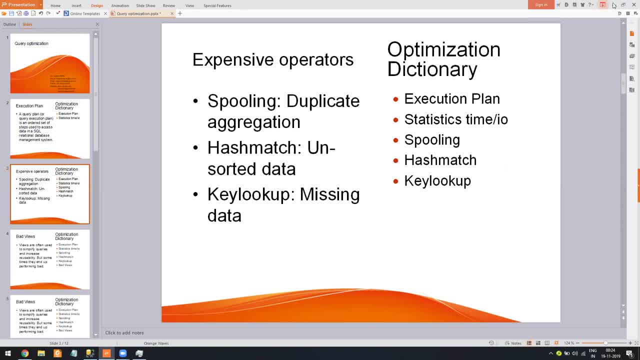 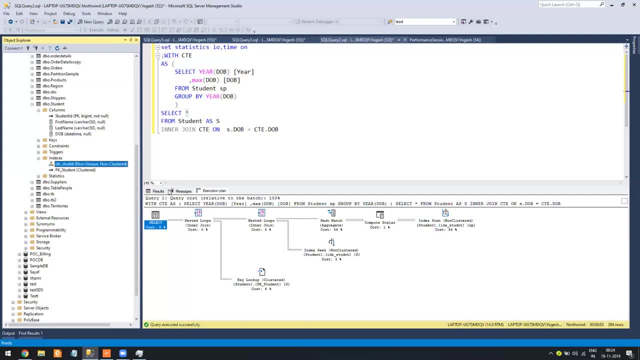 add the column to the index. now here I can see there is an extra column, so what I will do is I will go into my index, add that column and see whether my key lookup goes or not. let me just add my last name to the column. let's see. 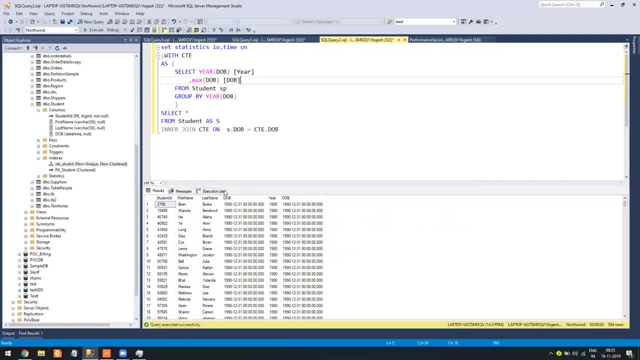 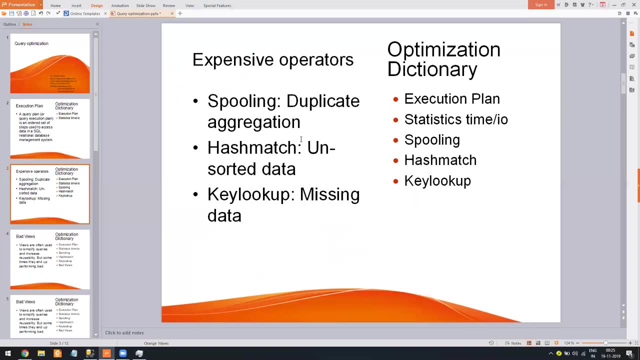 problem recreate and I rerun it and here you see there is no key lookup happening. and reason for that is because now it contains the column. now, sorry. solution to key lookup is if there is a missing data in the index, now how you can fix it, add the data. but sometimes 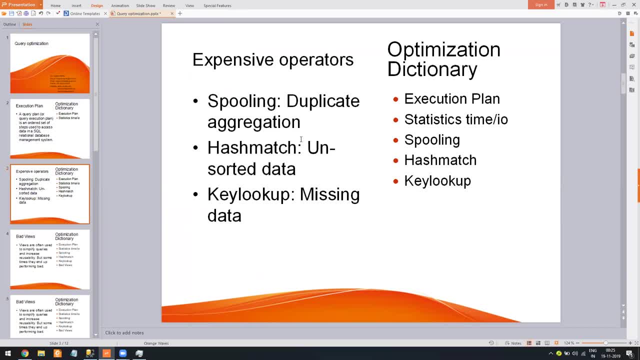 it's not possible because a lot of times suggestion will come with add all the columns. you cannot add all the columns to the index. it will be like miserable updates you will have and inserts. so key lookup is if you have a huge table and huge index and just one column. 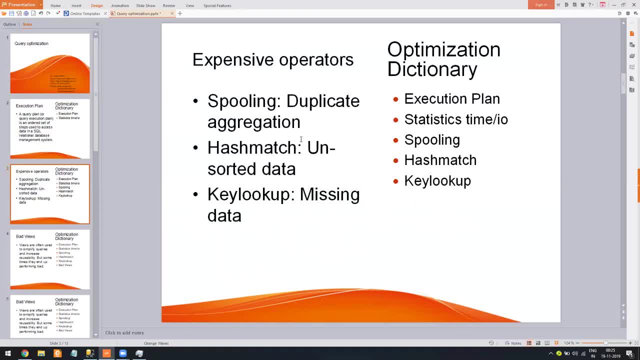 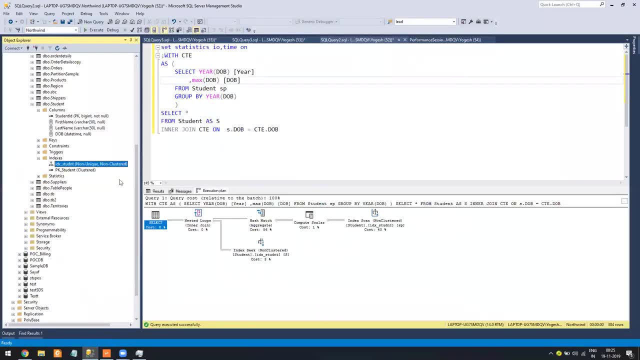 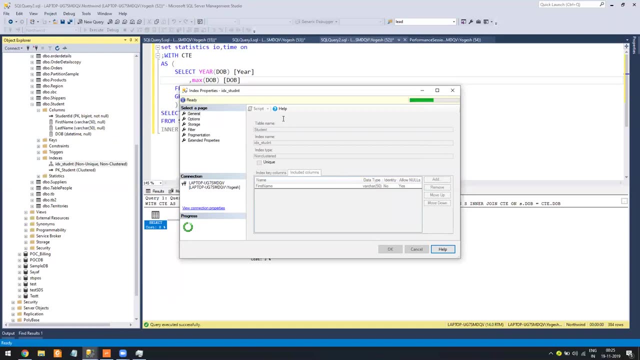 is missing from the index. take a chance, add that column to the index to make it far faster. and you want to see whether the key lookup increase the logical read or not. let's check. let me just remove my index again. run it again. so now let me. 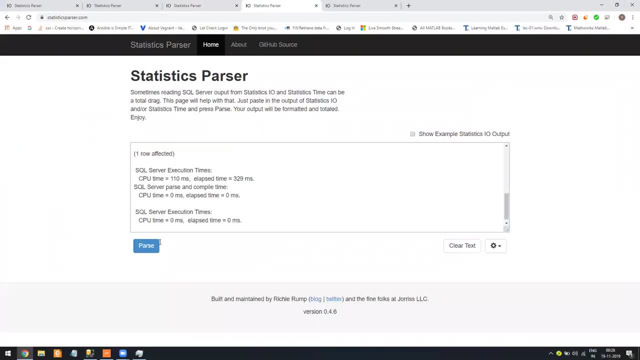 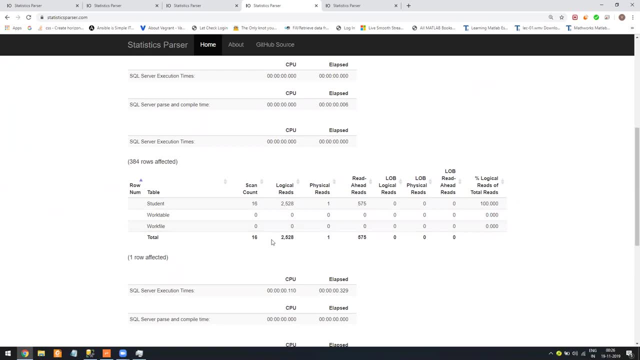 just duplicate the thing and run. now here you see it. because there is a key lookup, it end up doing more logical reads than the actual query without the index. see the irony. so because still it is using the index, because the filtration is faster, just to get the data again it has to again go to the table. 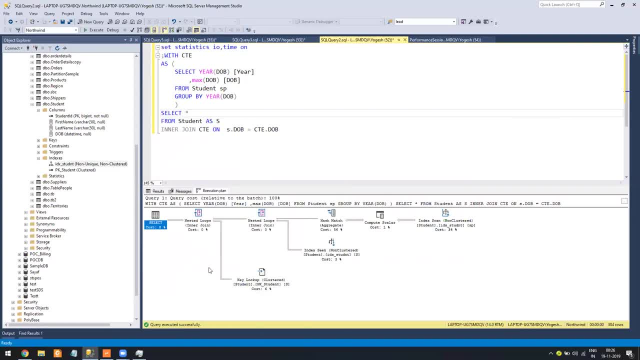 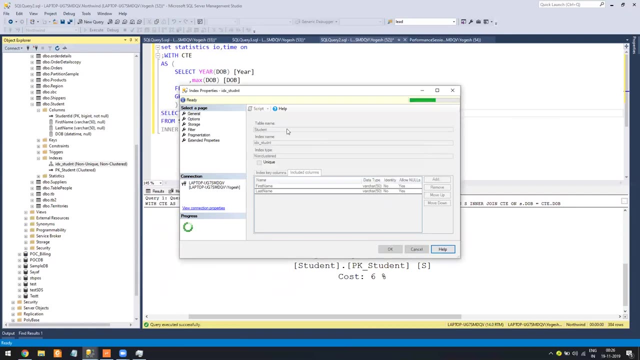 it has to read more data to get just one column out. so that's why this key lookup is doing more logical read than the actual query. so if i just fix it by adding that one column again and run this again, again it's back to the three digit. so all. 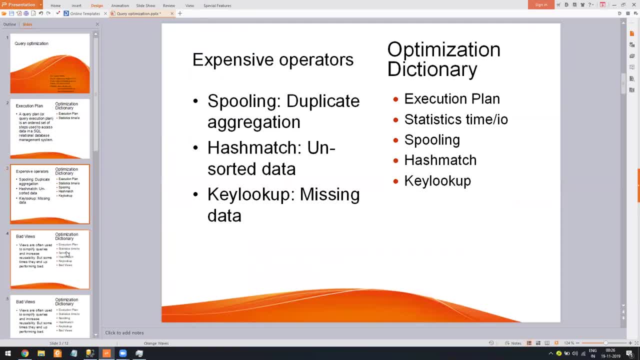 good so far, because this is the main part- because whenever you are seeing a query, you need to know whether there is a spooling or not, how to fix the spooling. if it is duplicate, you can remove it using cp or table variable. unsorted data- missing index. 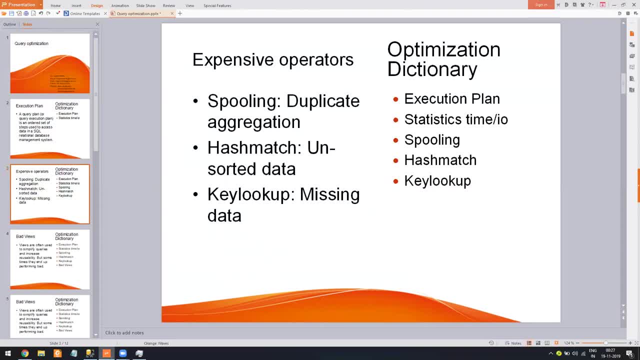 whether index are getting properly utilized or not, because i have seen a lot of time indexes are there and people do crazy functions. you can version of date and date time just to make their life easier by writing that small syntax, but it end up doing bad. whether there is a key. 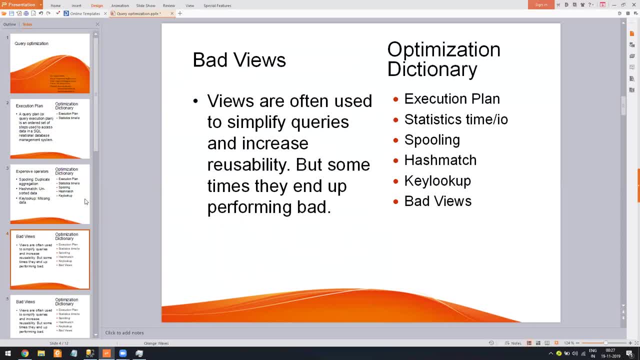 lookup or not. okay, once you have done that, see whether there is a bad views or not. now, views are often used to simplify the query, so they are not bad, but a lot of time its performance they become a problem. now we know, like the definition of views, it's just a stored. 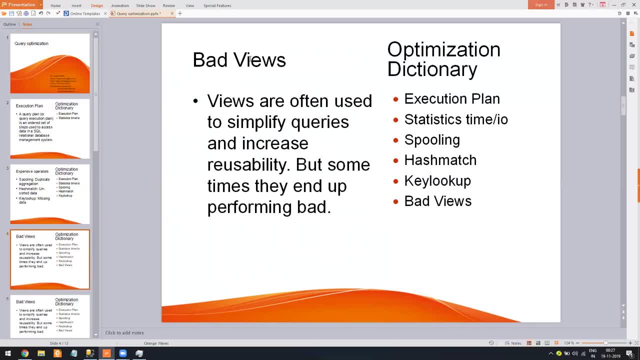 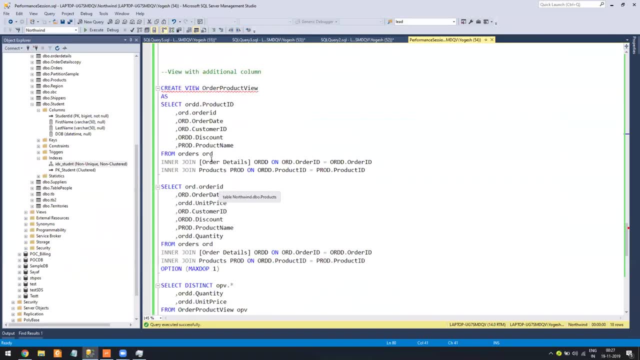 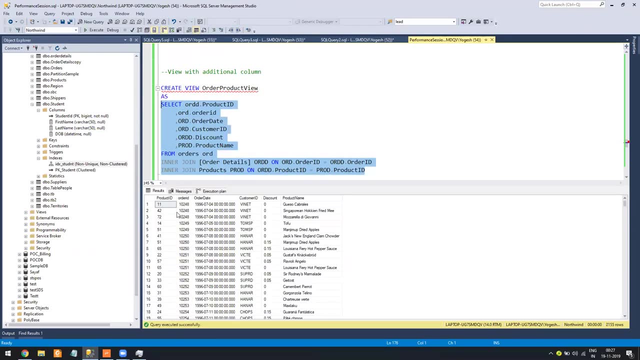 query now how it can be a bad in the performance. let me show you a simple example. so i created a view. let me go to the bottom. so i created a simple view which is getting me. it is joining three tables- order, order details and product- and it is getting me certain like. 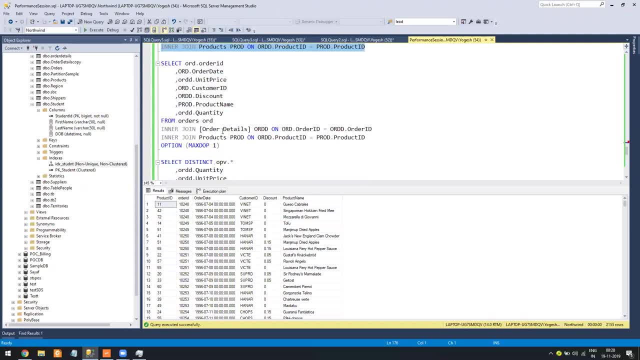 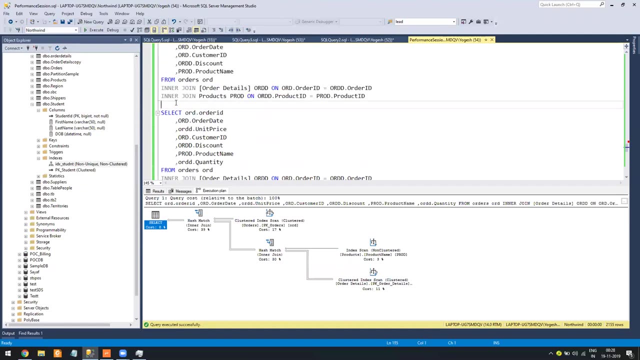 you can say six, six columns. okay. now this is one more query, which is exact query. there is nothing but just a max top. i added because to remove the and if i go to the execution plan, okay, let's, let me just run my cdnc, the execution plan for this- and. 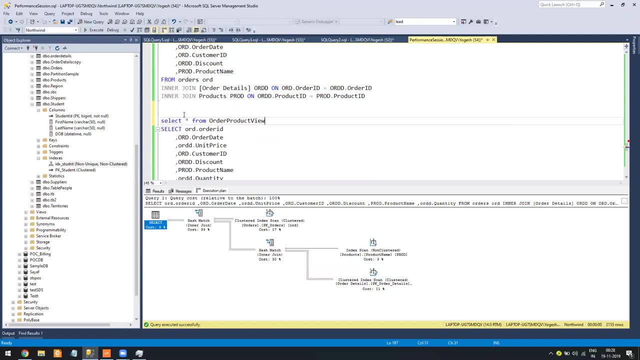 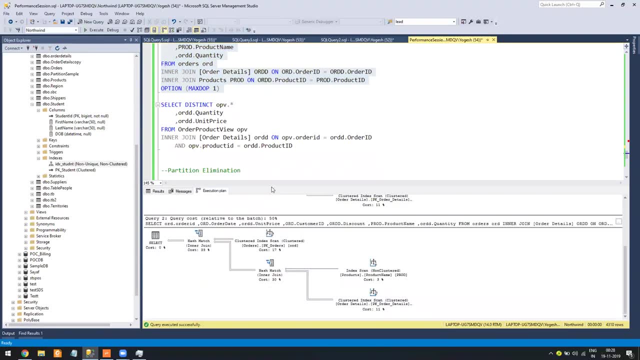 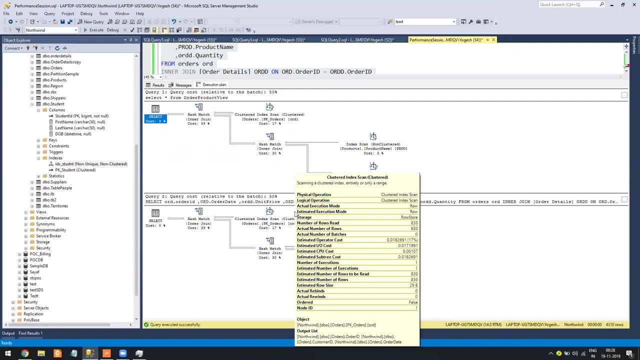 the below: yes, and i will run and see the execution plan of both the queries. now, here you see, the execution plan is exactly the same, so there is no performance problem. the cost is also, it says, fifty percent. so the execution plan if i run ct and that same query outside. 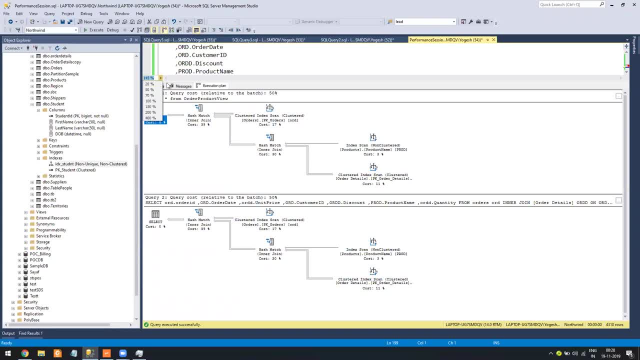 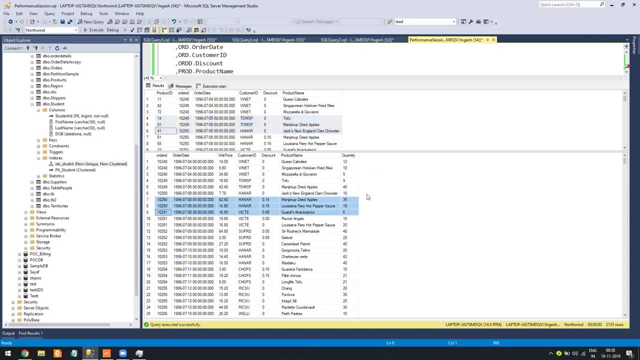 is the same, but there is a difference in the data. now, what is the difference? in my view, i am getting six column, but here i am getting one more column extra. now, a lot of time there will be situation where someone has to write a new stored procedure or function or query where they are. 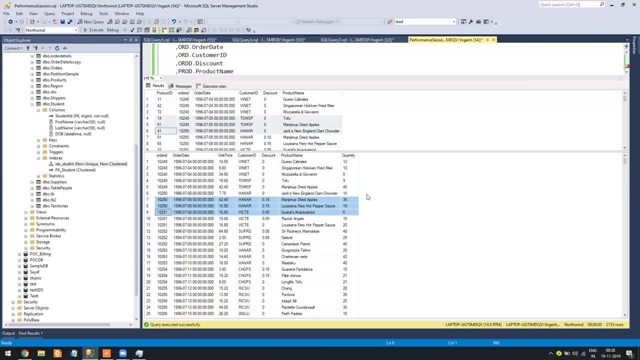 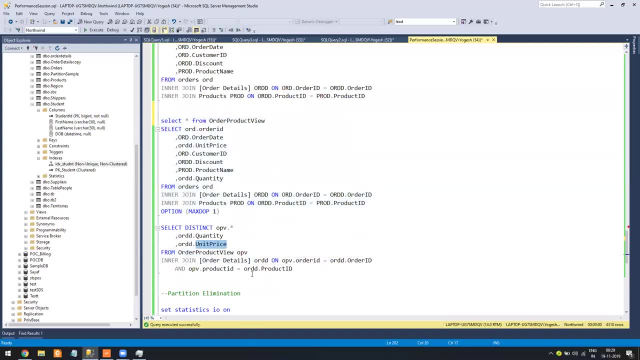 using existing views, and views are missing one column from the table. so what they generally do is they will add one more join of the view to the same table again, just to get that one column out. now what will happen? let's compare. i am using the view going to the table back. 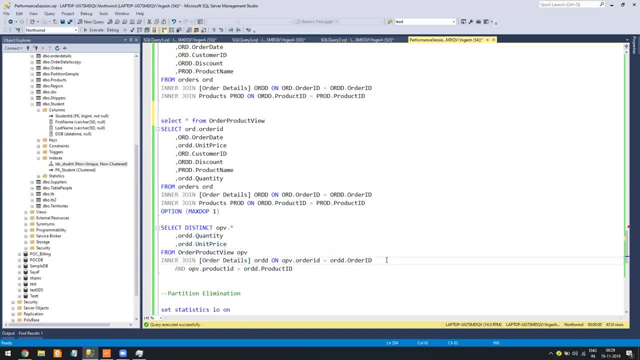 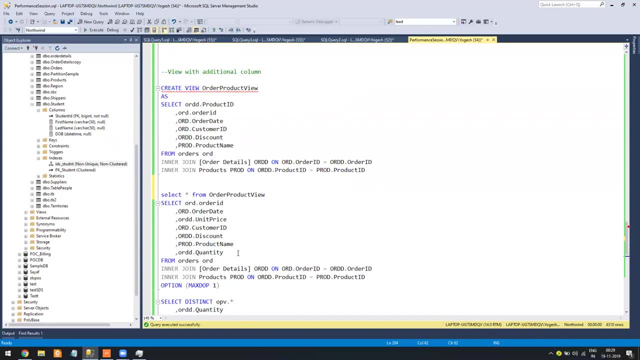 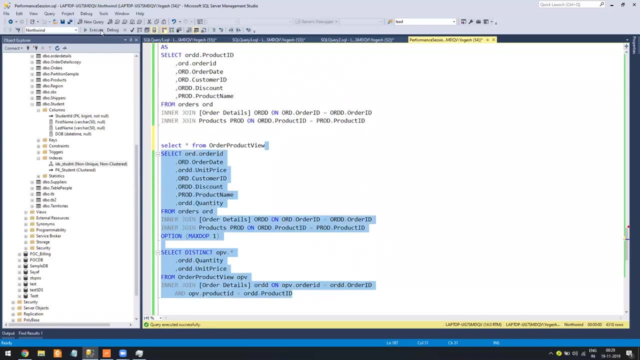 just to get one more column. okay, i think there is something missing. okay, let me. i think there is something missing. okay, let me just run so that you won't get much time to waste on this. okay now, if i run my both the queries now see the execution plan. 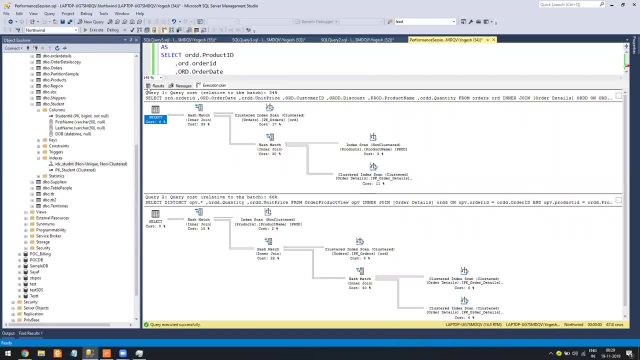 this execution plan is again the query, even though i am getting that one column. but here in this, just getting that one column, what has happened? it has to go back to the table again to get this, that one column, okay, but here in this, just getting that one column, because here you see it is. 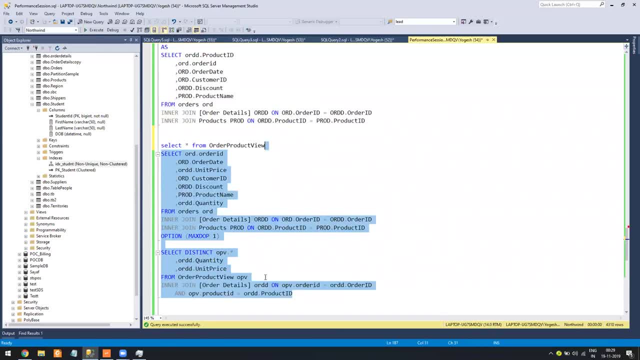 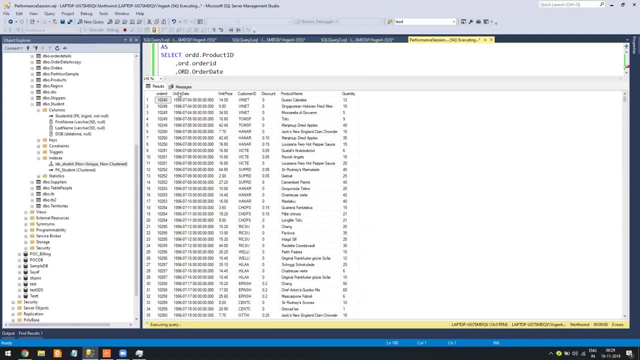 joining with order details two times because just i have to get the one more column. and logical reads. if i see the logical read of this. if i see the logical read of this: let's say it is 2 and 22 and 11. let's say it is 2 and 22 and 11. 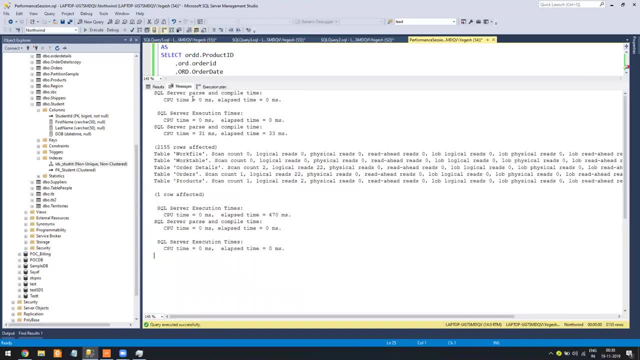 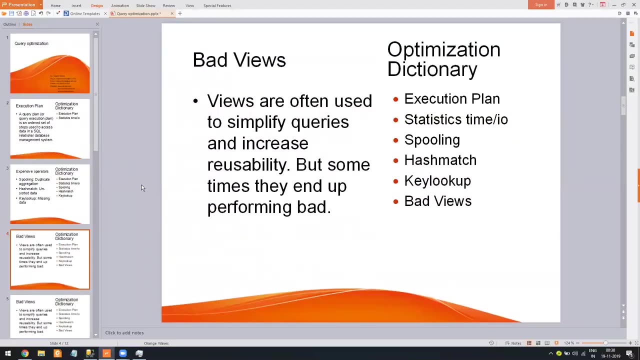 simple and if i run the logical read for this fellow, so 11 become 22 again. because it's become double, because this is order details, okay, order details. as it has to refer, two becomes the double. so bad views are like. there is no technical term as bad view. the bad views is if 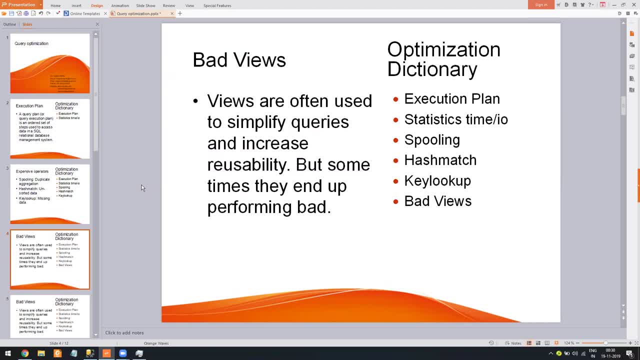 there is a view which people are using in all the queries, and if they are missing columns and instead of writing a new view or altering the same view, what they are doing is trying to join the same table which are already part of the view, then it's bad. so what? what is the solution? either, 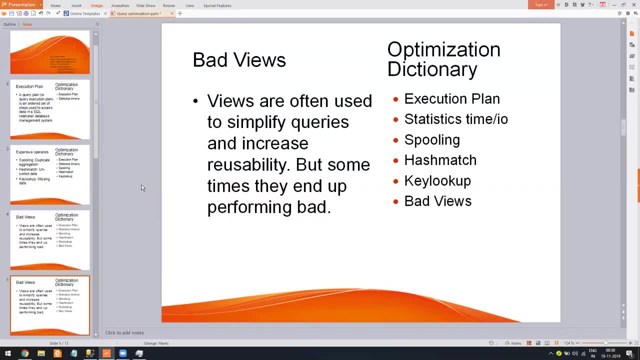 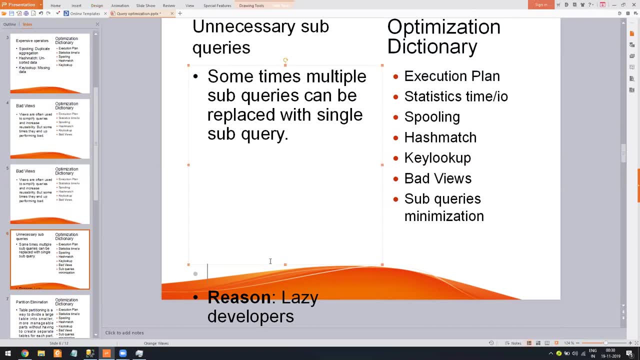 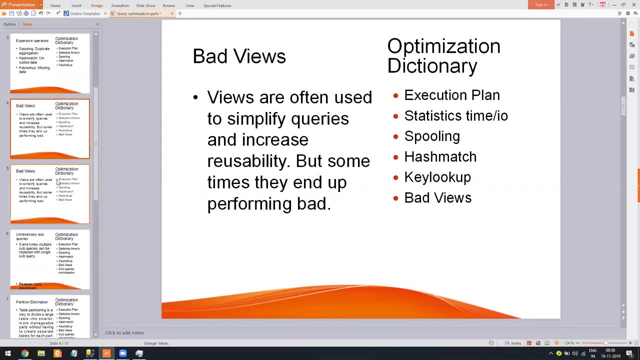 create a new view or alter the existing. that's the simple thing. okay, okay, now coming toward. okay, let's see. okay now. unnecessary sub queries now. this is one of the best example i why i have to click: it slides. okay, unnecessary sub queries now. i will give a simple example. i will give you. 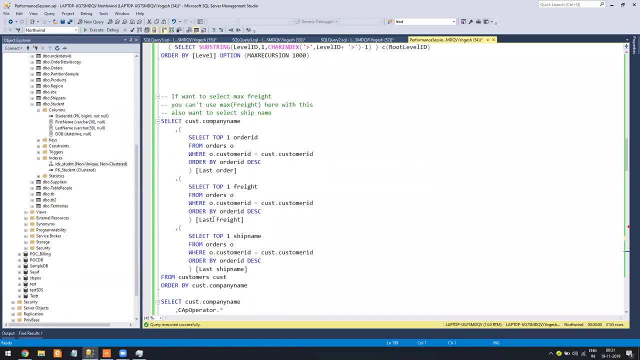 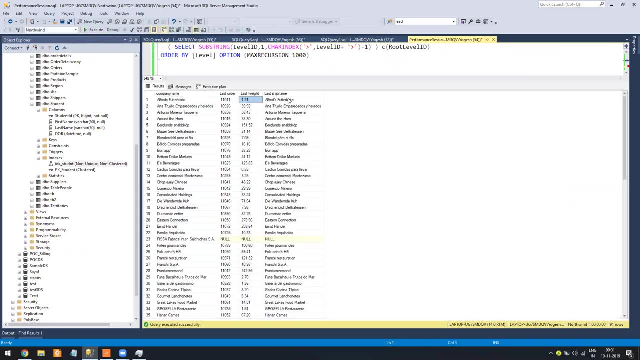 time to think what will be your query and then you tell me: okay, i have to get me my all the customers and their most distant order, last order, what was the amount of that order and what was the- you can say- ship name with which what they ship like from, uh, with which ship they ever ship to the customer? 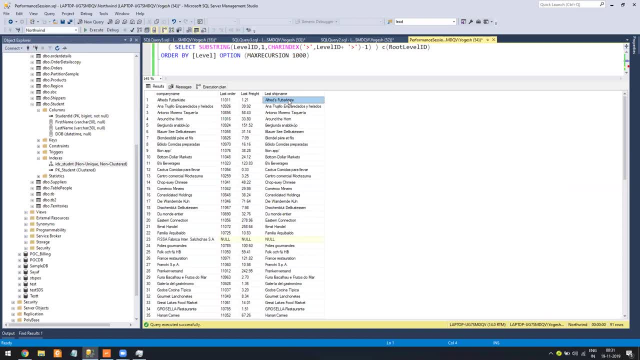 now i'm just getting the last, which most recent order, not all the orders. so i cannot do a join with orders because then it will get me all the data. i cannot do a maximum order id because if i do a maximum order id, then how i will get them by last right? i have to get maximum right now it can. 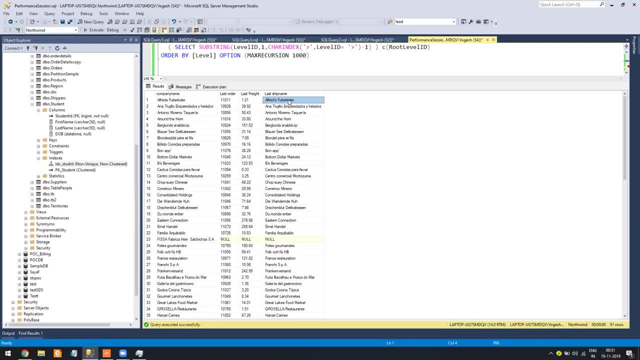 be a fold order, so it won't be right. so just by using maximum order id i won't be able to get. so how i should be able to do that? just think about it getting just the most recent one or not multiple, any idea. so usually what people do is they will write. 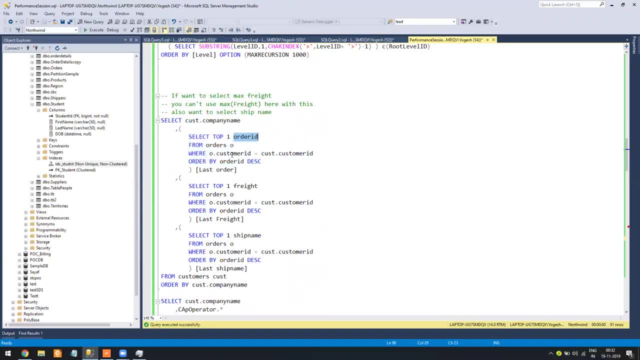 sub queries, like they will say for this column. get me the order id from the table, join it on the customer id from the table orders. order it by order id descending on. get the maximum order id- there's a separate thing- and then in the thread, similarly, get order from the most recent top one order from the order table: join on. 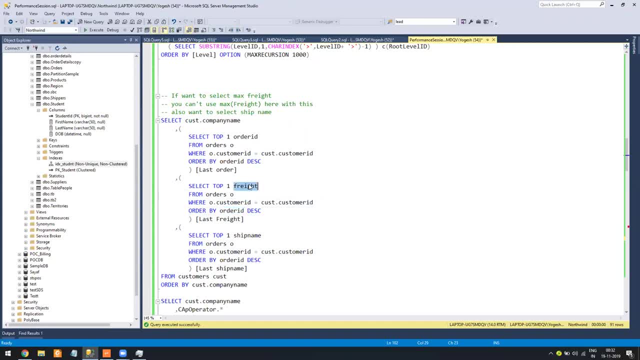 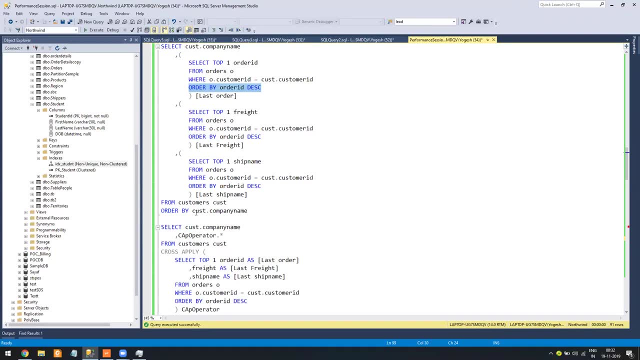 the customer id, order by order id descending and get the freight means it is from the same order, because i am doing order by order already descending, so i will always get a most recent order and then the ship name: same, exactly the same way. now suppose i want to get the order date. 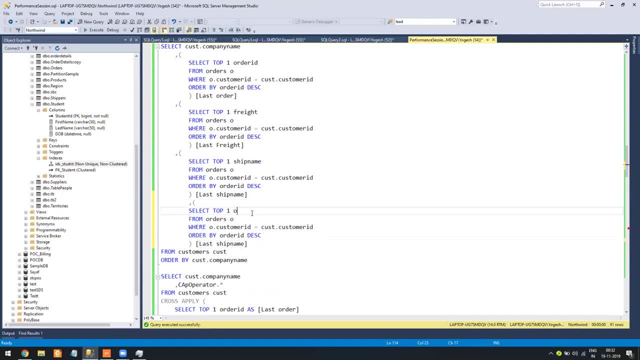 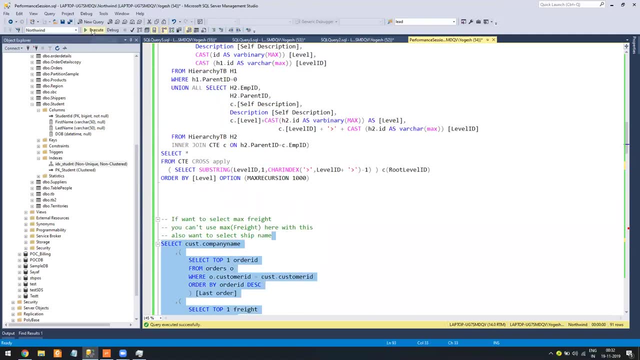 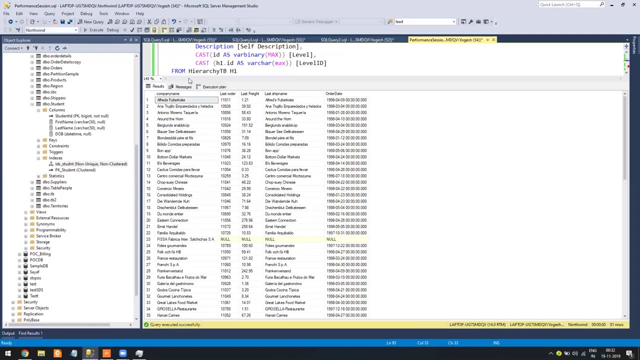 what i will do is i will copy: add one more order date and i will copy this one out. So what this approach do is for n number of columns I have to write n number of times I have to write the subquery. So this becomes very problematic because I want to get all the you can say you can. 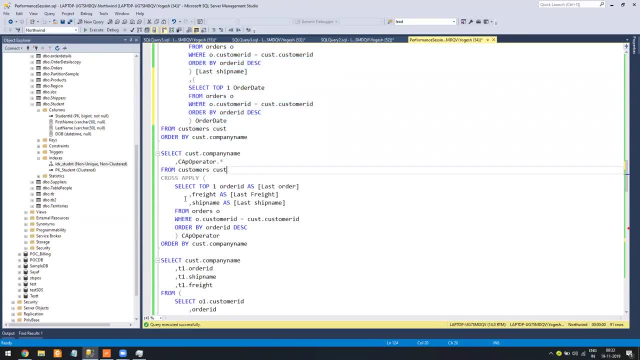 say most recent, just the most recent. So how I resolve it? I can dissolve it by using cross apply. Now in cross apply, if you haven't used cross apply, it's a separate topic And if you have to go in cross apply it's. it's a small topic, but it's a very good and 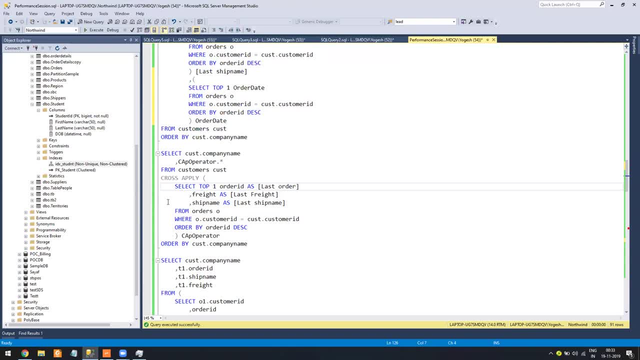 interesting topic. If you know cross apply, you can do a lot of things. What cross apply do is for each record coming from the left side, it will run this subquery. So here what I'm doing is, instead of running four subquery, I'm saying get me one record. 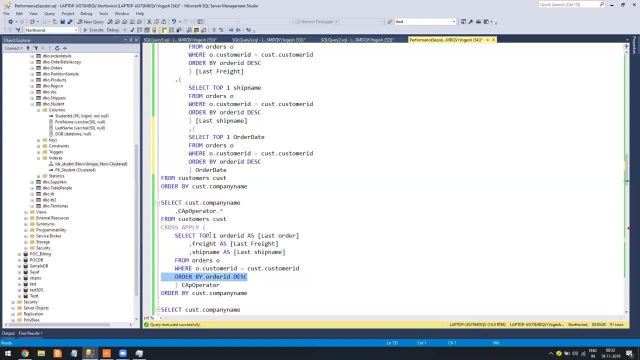 from order where the customer ID matches order by order ID descending, And in that one record I'm getting all the columns I need to order date And if I run this, I can get the same exact output. Now, if I run both the queries, let's see. 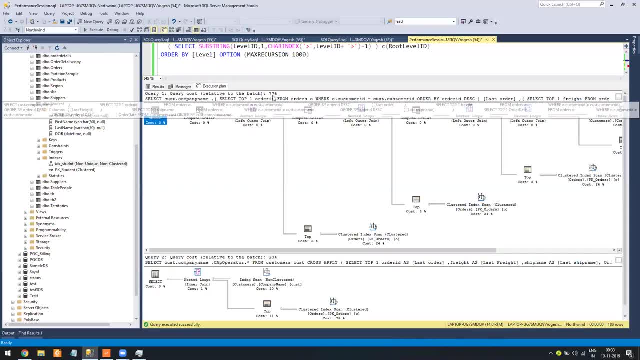 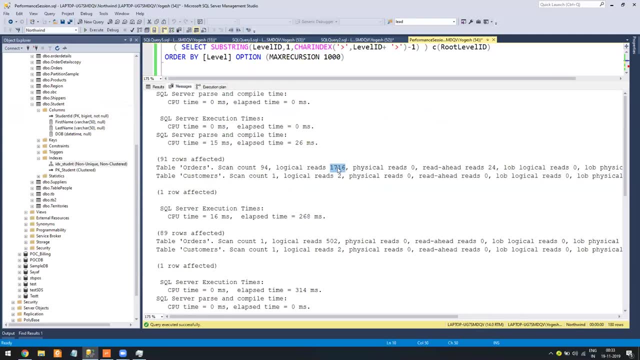 What will be the performance? So above query cost me 77% and the below query 23%. in the batch, Above query logical read is like, let's say, zoom 17,, 16 and logical read for the below queries seven or five, zero two. 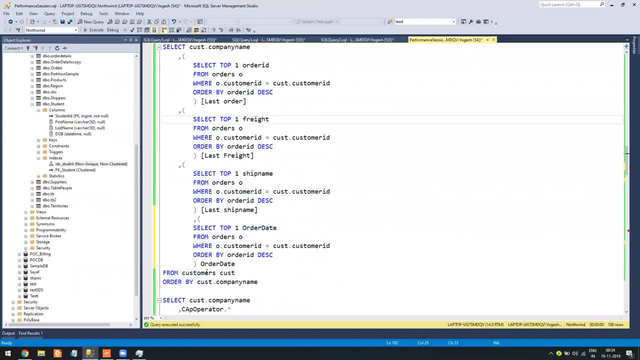 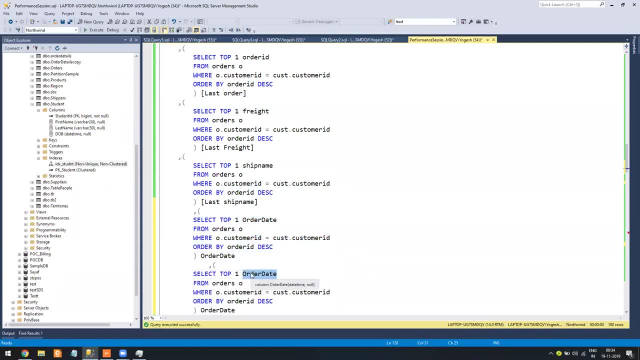 So it's like three times smaller. And the problem with above query: if I have to get more columns, I have to add more queries and it becomes expensive. like every time, it will become more expensive. let's say ship country. Let's say ship country. 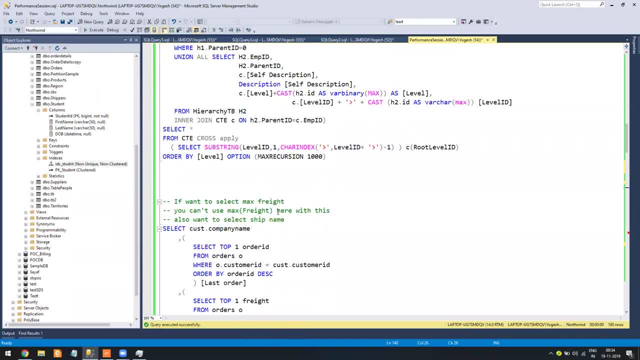 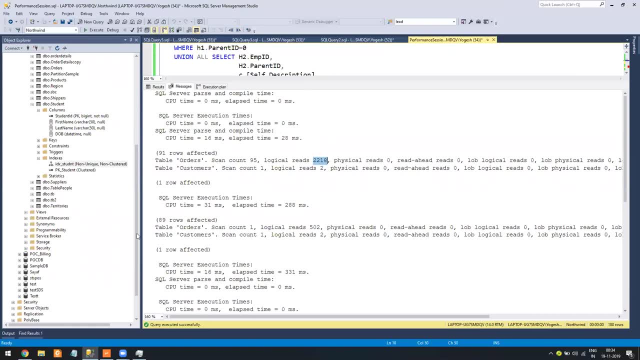 And if I run both the queries again all together and see now it becomes more logical read because it is increasing. but the below query is five zero two. It's the constant because it has to get only one time all the records, all the columns. 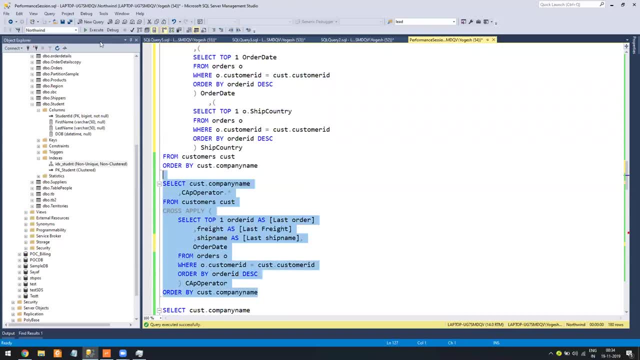 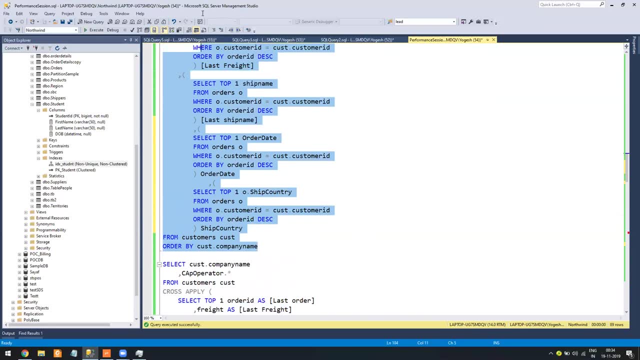 whatever I need. Okay Now here, one problem will be like cross apply, You will have 89 records. The above query will give you around 90 or 91 records because it's getting all the customer first. cross apply only gets a common customer. 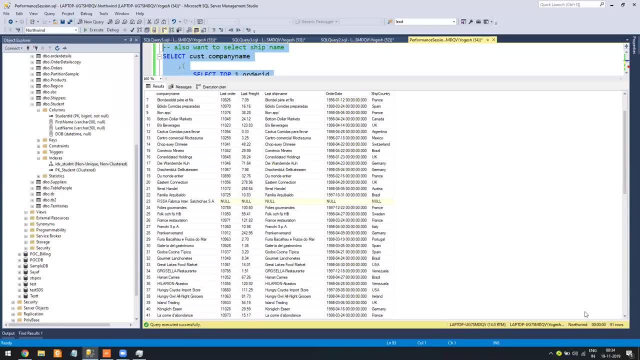 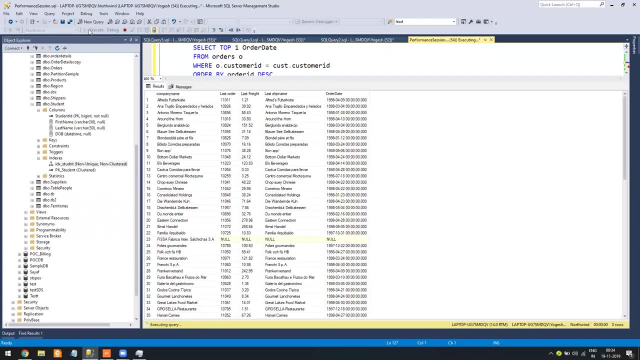 You can say, uh, output, So here is 91. So how to fix it? There isn't something called an outer apply, So it's similar to cross apply. It's like a left John. So it will get all the records even though the patient, the customer, hasn't placed any. 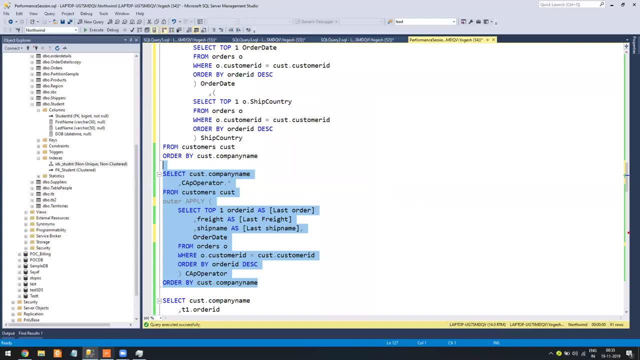 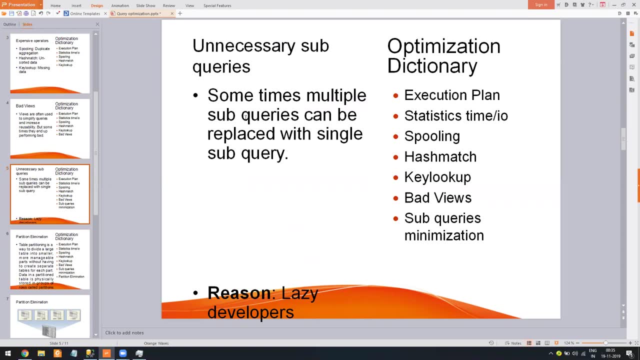 order. So it's very simple, Okay. So I hope this video is helping you out. So the concept is like unnecessary subquery using cross apply, uh or any other logic. whatever you want to do, that's all on you, but usually cross apply, use for that. 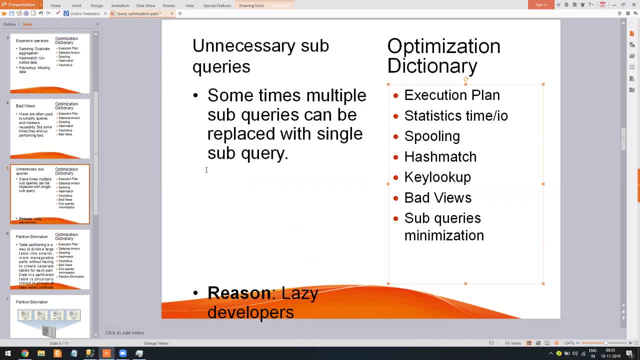 And sometimes I use temp table also. So if you remove unnecessary sub queries, it will for sure reduce the logical rate. If logical reads are getting reduced, everything is good. Okay, I don't know why my slides are duplicated. Let me just remove it. 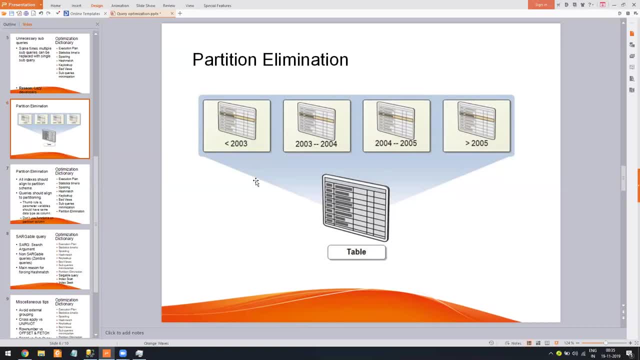 Okay, Now this is the most important topic. Understand, because this will make a huge impact on your performance, And this is partition elimination. If somehow your database is partitioned, your company use partition. Okay, Believe me, if you can see your query, are not using the partition properly and you make 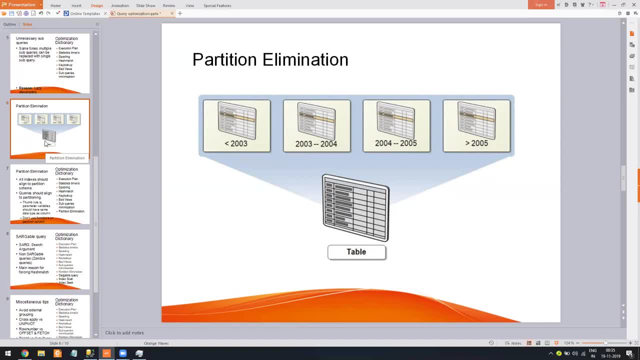 them use it, there will be a huge change in performance, and that I can just show you now itself. Okay, So partition is nothing, but like you subdivide table physically in terms of the partition means you said like I want to create partition yearly from less than 2003 records will be. 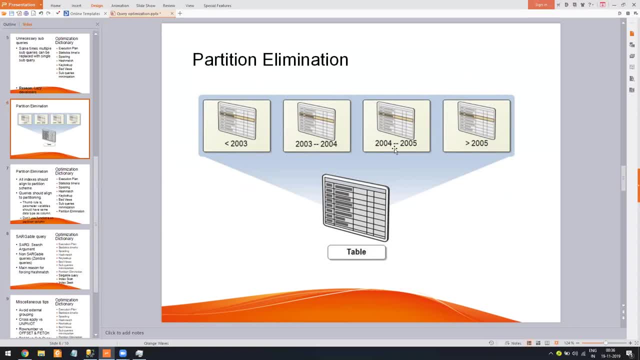 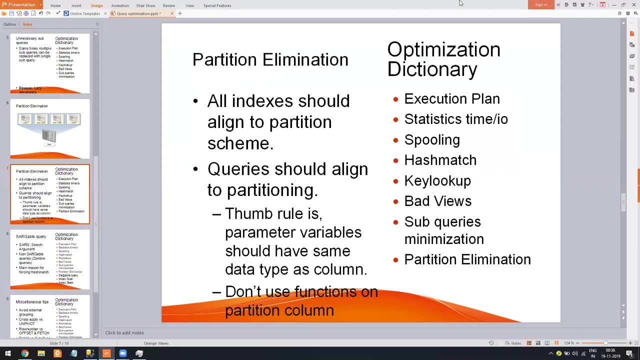 in partition: a 2003 to four will be B, four to five will be in C and Great. So this is the difference: You can do your data in partition, but you can't do it in your query. You can do it in your query in the same way that you did in your query. 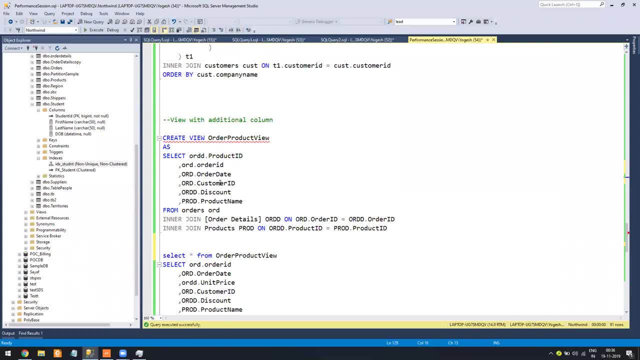 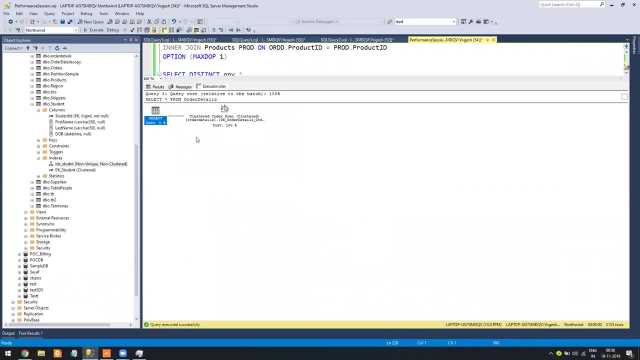 Now what happens is your data is partitioned, but your query is not using those partitions. Now how to fix it? I will just give you a simple example. I have a table, order details, which is partition. Okay, If I run my sub query, go here, go into my properties. 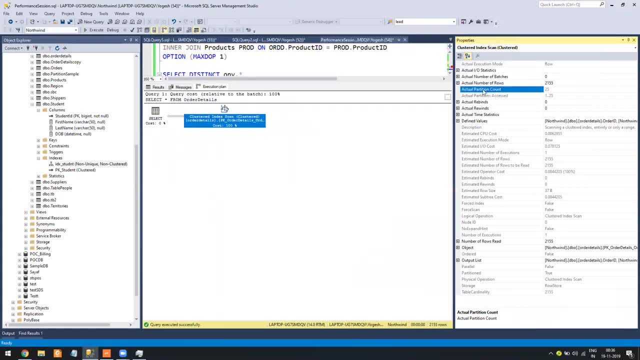 Let me just select. So here you see there is an action. So this thing- actual partition count- you won't find in other queries which you just have. Okay, So if you want to look at the data in the sub query, you can have a little bit of a look at this. 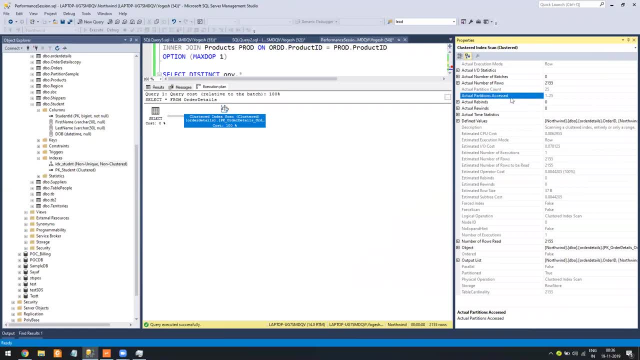 You can have a little bit of a look at this. queries which on other query which doesn't have the partitionings. So this will be always on the tables which have the partition. So here these two things will come: actual partition count and the actual partitions access. So it is getting how many it used, like 1,, 2,. 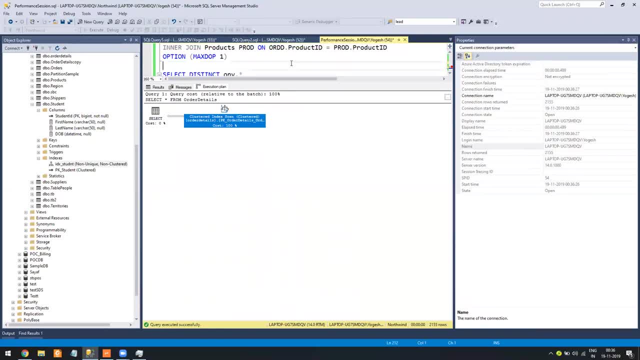 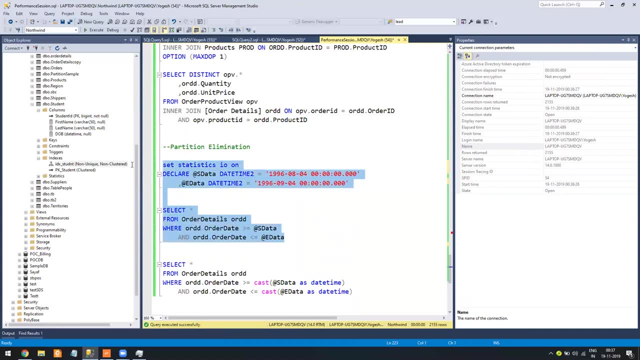 25, and 25 are the total use because I'm doing star. So what I have to do is I have these two parameters: start date and end date. I'm getting the records between these two dates and the below query is exactly the same, but just there is a casting. like I'm using casting, 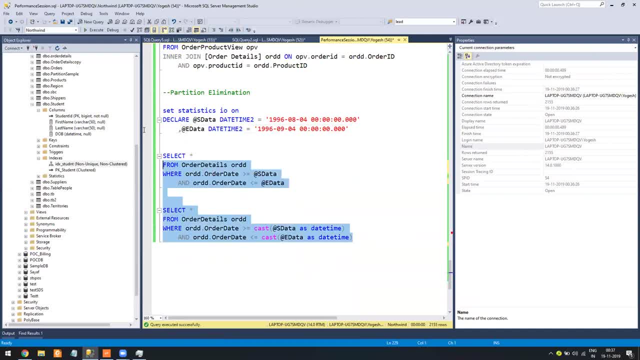 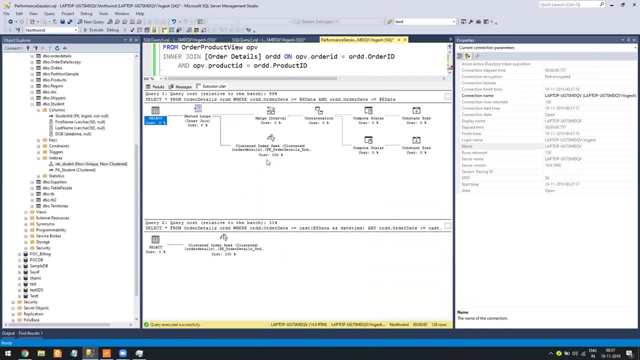 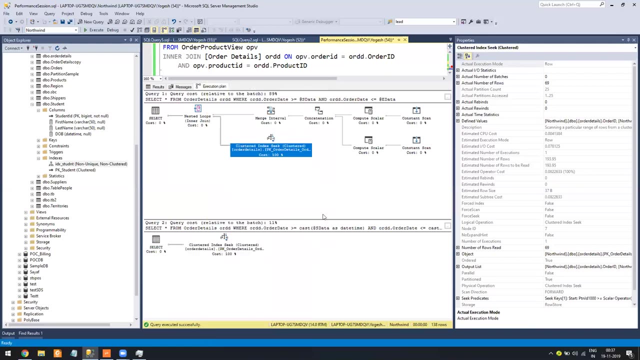 the date time 2 to date. Now let me run both the queries together so that you can see what is the difference. So the first query is seems to be little bit complex, but if I click here, what it has done, it has, let me. yeah, So the first query, what it has done, it has selected. 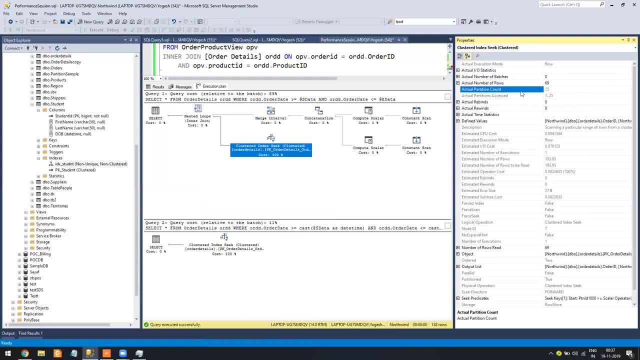 all the partitions means total partition in the table are 25.. It's still used All the 25 partitions, So there is no partition elimination happening means no partition got avoided. But let's see the second query. See, the first query is little bit complex also. 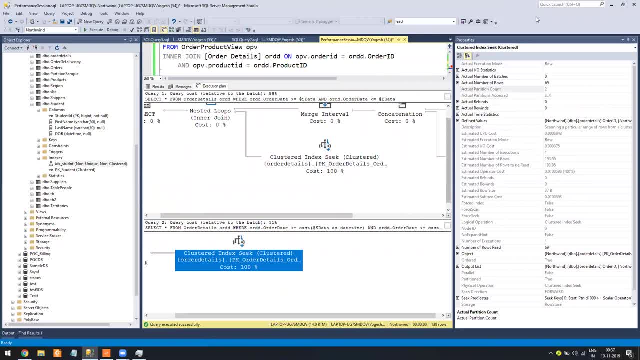 The second query. Now, if I click on this and see the exit, this my properties. here you see actual partition count is 2.. Only 2 partitions. it has to go to get you the data. So it was able to eliminate 23 partitions. Total partition was 25.. 23. it avoided Only 2 partitions. it 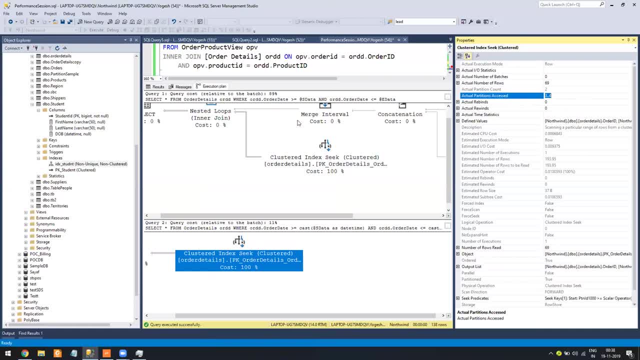 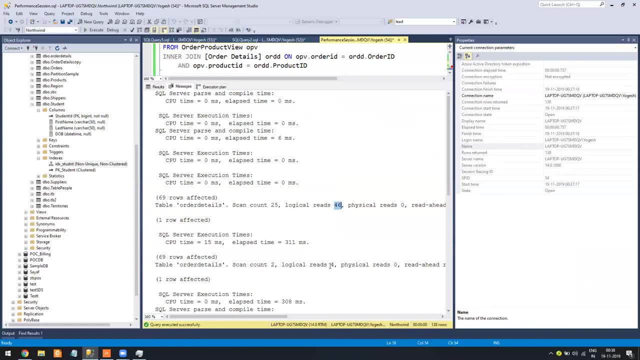 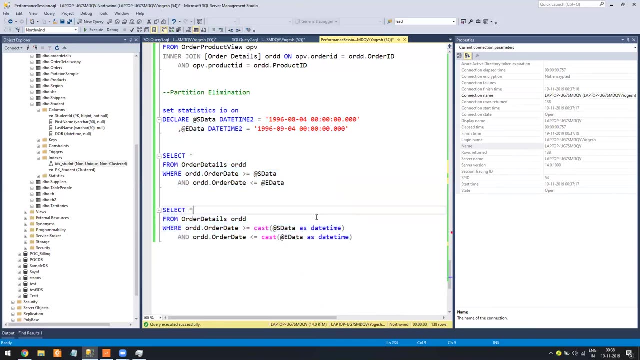 has to go to get you the data For sure, faster. So here see the performance above query 89 percent, This query 11 percent. What is the logical rate? First one used 46 logical rates and second one used only 4.. Now what is the difference between both the queries? The column, 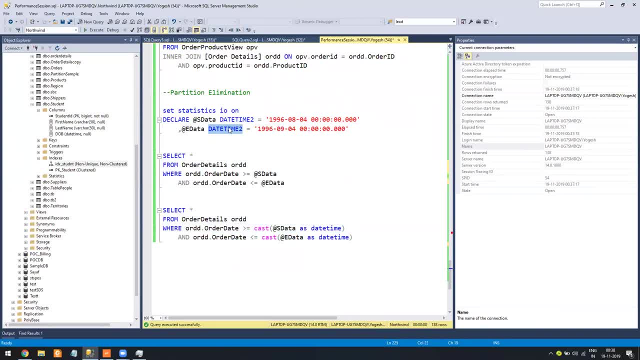 data type. order date was date time, not the date time 2.. Just a basic difference. The parameter column type data type doesn't match with the column data type And this just gives you the data type. Just don't go for the partition elimination. This can also work with other. 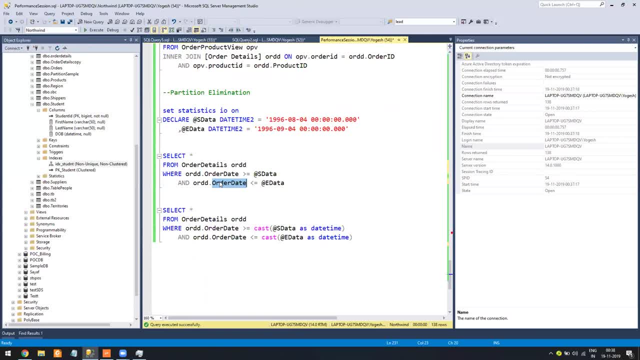 things also Like without partitioning also. But here you see, in partitioning for you date, time to end date may be almost the same if you are not considering the millisecond part of it, But for SQL Server it's a huge difference. So what SQL Server do is, if it doesn't match. 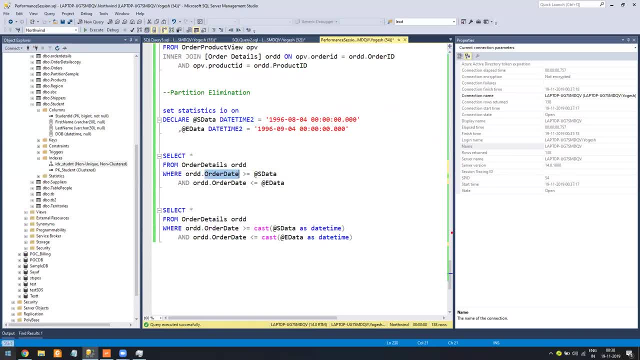 the data type. it goes for all the partitions And, believe me, this thing has made a huge impact in my experience. There was a query we optimized from 90 minutes to ten seconds and it was able to get you the data type. So in this case you can see that it was just. 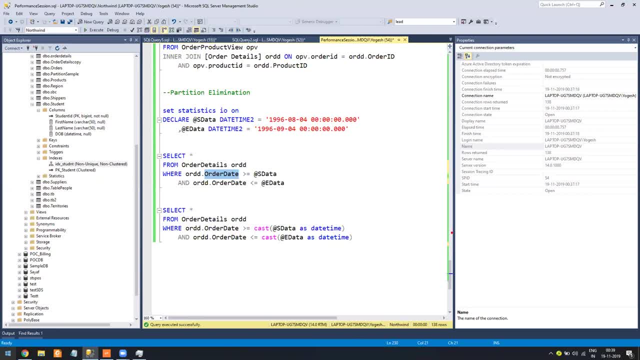 second, how it happened was I was able to get that query from 90 minutes to two minutes by other spooling and other thing, but from that two minutes to 10 seconds just this partition elimination brings. and why? because our table was around 200 GB of data and the moment we 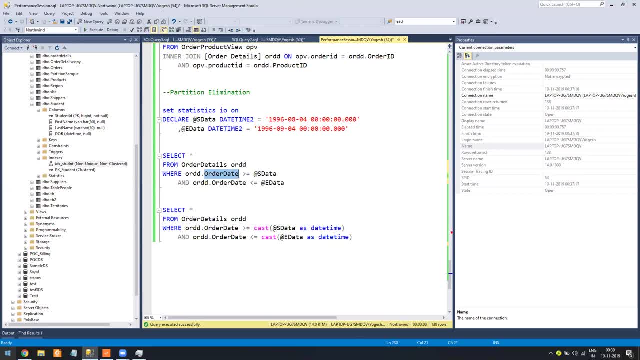 did partitioning. it has to just scan few records or few partition to get the data when there were like around almost around like 90 partitions and it has to just go in one partition, get the data like not the 90, it's like almost like 100, 200 partition because there was like 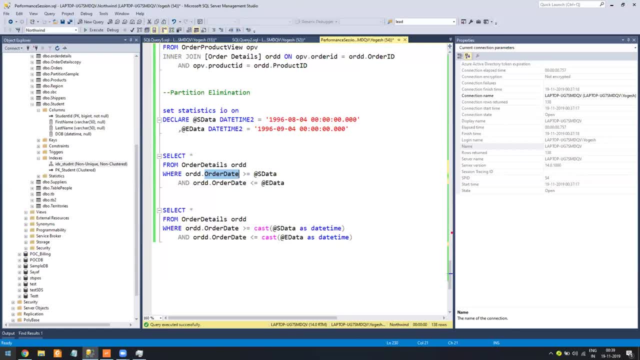 around 8 months data and the moment there is a partition, it just have to go in one or two partition it. there was a huge difference to get the data. so partition elimination why it doesn't happen? one using a different data type and second, there can be different reasons. 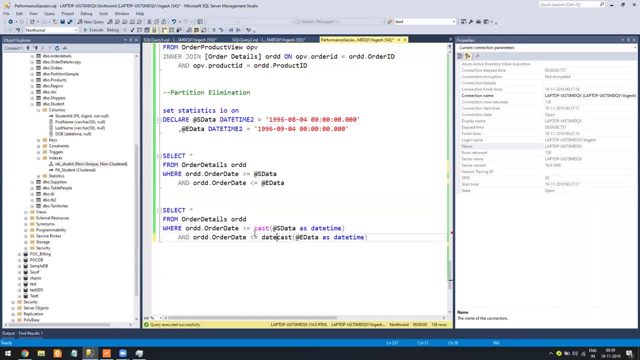 also, let's say I added a function, date add. you remember this is my favorite function, to show an example. so what I did is Now not here. let me do it on the other side. So now, if I run the same query again and see what happened to the partitioning, now here: 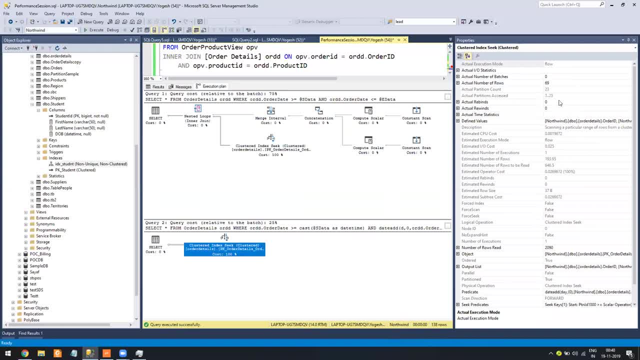 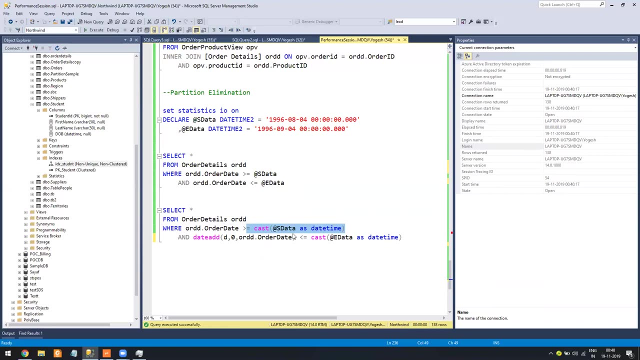 the partition is same, 25. now if I go here, what happens? it only scan 23 partition. it only was unable to. it was able to exclude only two partition. the reason was it was able to determine The start. You can say date, because start date was very simple, but end date it was unable to determine. 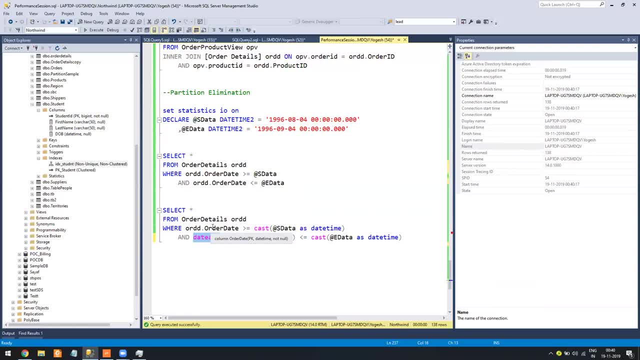 because there is a function used on the column. you have to be very sure never to use function on the columns in where clause and in joints till the time you can avoid them. okay, because if there is no other like way to do it, then you cannot do it, but if there is a way, always. 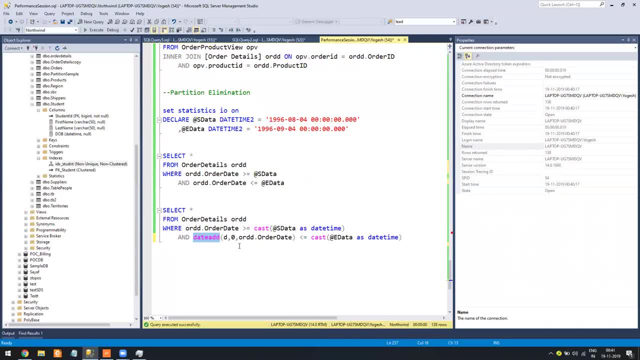 avoid using any function. this thing mess up your whole query. so what I just did is I just use a function. Same query remains, like whole query remains same and it has a problem. now I will just transfer it to start date. okay, so means end date is still deterministic. so if I run and 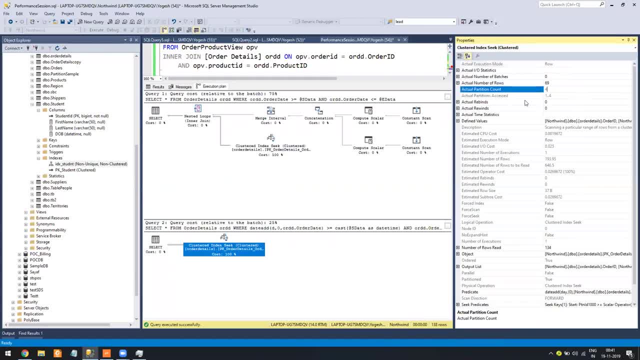 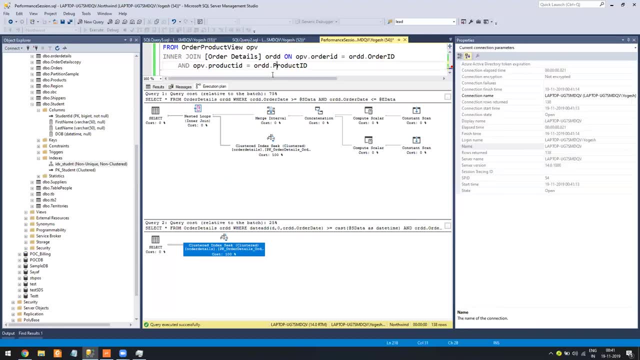 go into my query, click here and see how it becomes one to four. you remember it was using three to four, three and four partition, but now it is one to four because now it is unable to determine the start partition, so it is using four partition it is able to determine. 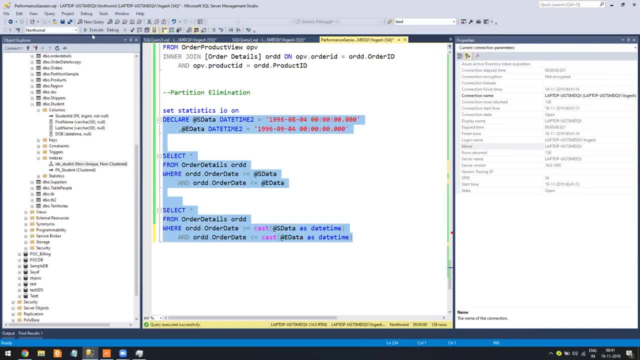 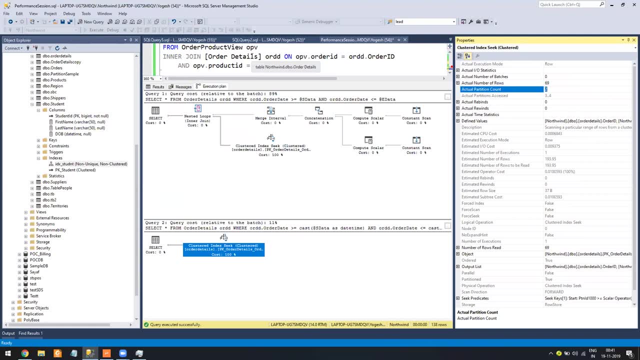 the last partition but not the starting partition. now, if I just remove, make it normal Again, I go. it only used to partition. so it matters a lot if your table is partitioned. the reason for partitioning the table is to run your queries fast. okay, if that is not. 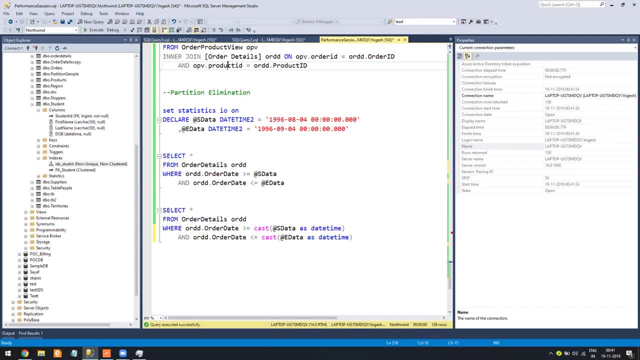 happening, then what is the use of partitioning? because partition is the headache on the maintenance. if you are doing the maintenance part and still your query doesn't use the partition you have to make sure they should use. so let's go back to the slide and see what we done. 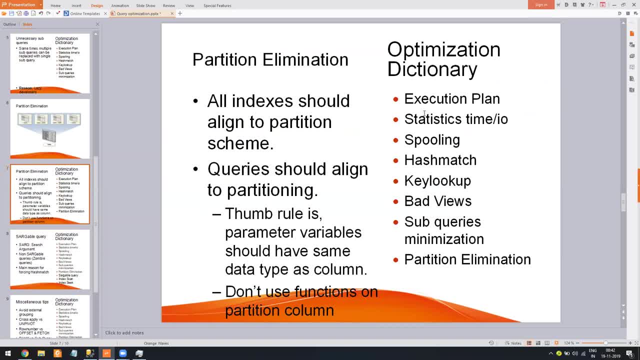 first We saw What is the execution plan, seeing how to use statistics, ION, time. then, once you have the bad running queries, see whether there is a spooling or not. spooling is nothing but duplicate aggregation. if there is a duplicate aggregation, remove it. how to remove it: different. 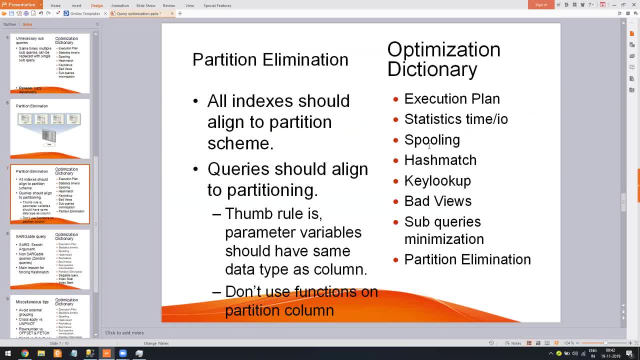 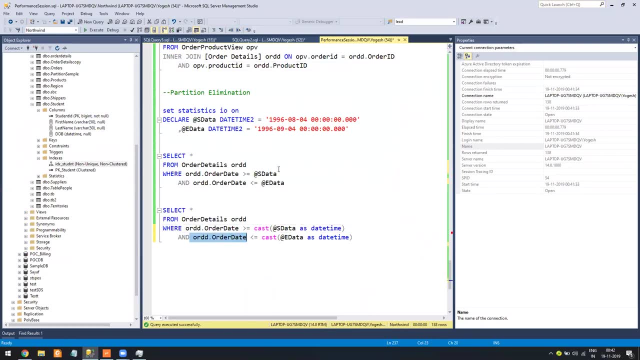 ways by CTE temp table or temporary table variable. then seeing hash match, hash matches, missing index because it's unsorted data, missing index or index is not getting used because of one reason: using any function on where close or join should not be there And it applies to partition elimination, it applies to hash match and one more. next slide. 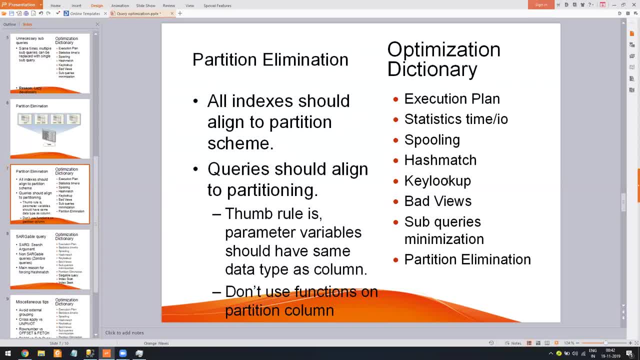 it will be the same for that also. Then, coming to the key lookup you look up is nothing but a missing data from your index. if you can add that, if it is one column and it doesn't make a difference, just add it to the index and it will be far easier for your SQL server to do it. then, after that, it comes. 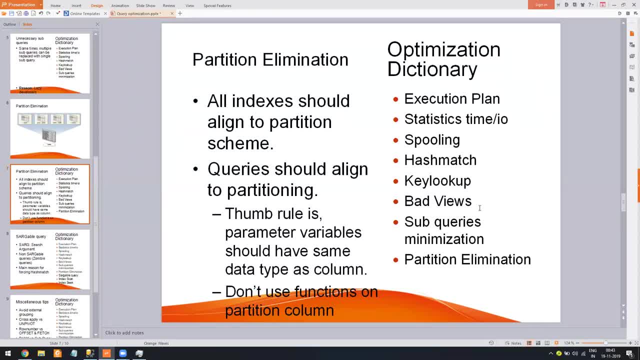 bad views. bad views are nothing. but when people don't alter the view just to get one or two column extra, If they make a joint to the same table, then it becomes miserable sometimes. So how you do it: alter the view or create a new view and use it then sub query minimization. 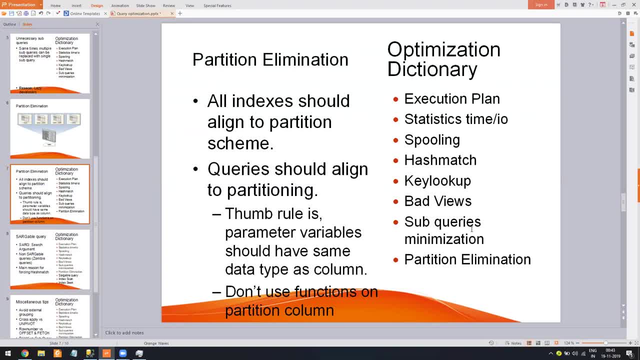 I use, just cross apply. we see the traditional, most common example where people have to get the most recent record and they start using sub queries and they become miserable. So how to fix it? just use a cross apply and get the data once and use it. 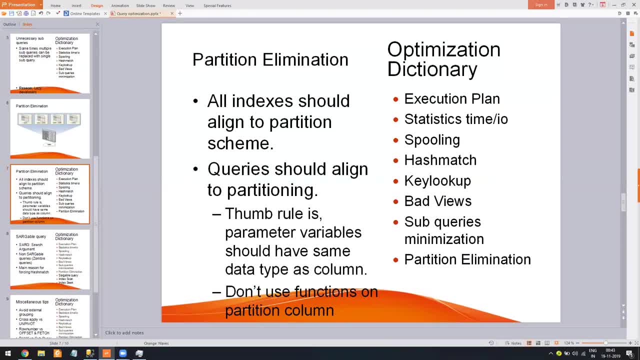 Last was partition elimination. this is most important. if your table are partitioned and your queries are not used, If you are using the partition properly, then there is a huge scope of improvement. if you just tweak the queries little bit and make them use your partition, it is awesome. 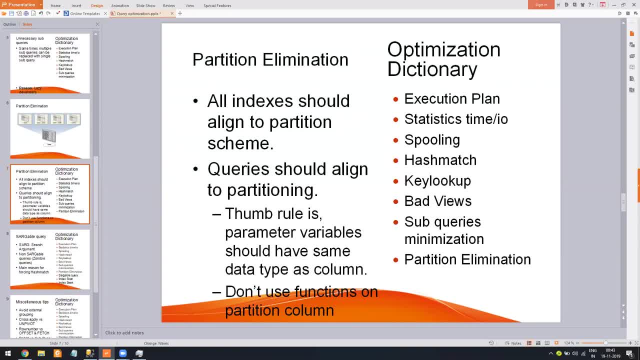 One more case I will let me discuss. it is not covered in the example. Now suppose I will give an example of casino industry, because I work there. So there is a table called player, then there is a player called game and then there is a table called jackpot. 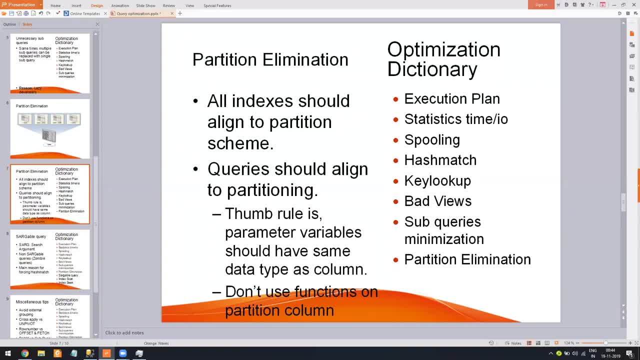 Now, once the player played a game, there is an order. You can say game date: okay, not in the player, like player game table. so player game table. he played, so there is an order date and that table is partitioned in game, not the order date, it's like game date when he played and that column is a partition key. 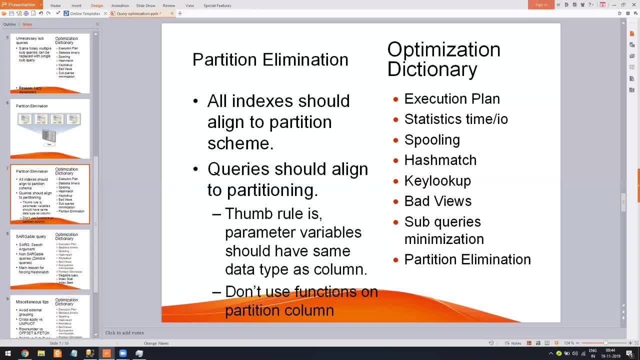 Now jackpot also have a game date. it also have the same column that is also partitioned. Now what happened? I used game date in a where clause on you can say player and game table, But I didn't used on jackpot. The reason is jackpot can only happen when there is a game. the person played a game. 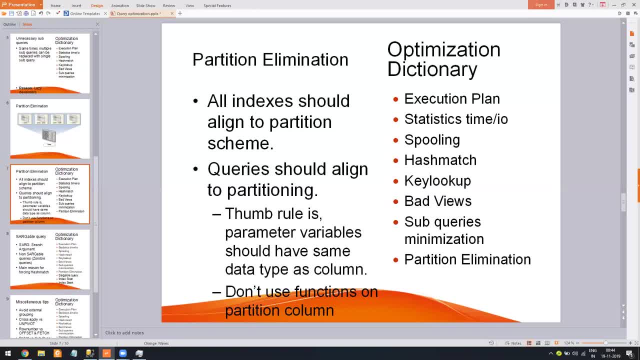 So I can put the same where condition on game date for jackpot as well as on this one. Now what will happen is both the tables are different, both are partitioned, So partition elimination will happen in both the tables, not in just one. So you can induce partition elimination if it is part of one condition and the same column. 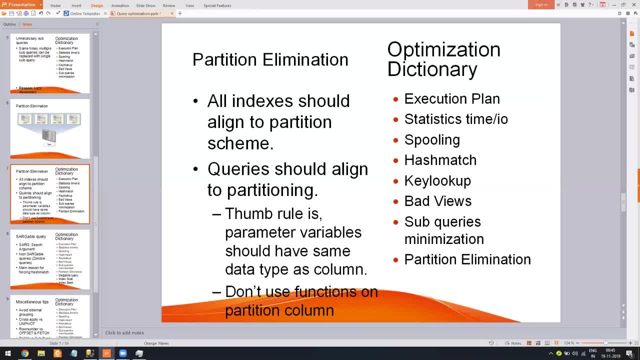 exists there and that's a partition column, why not use it, Even though this case doesn't mind, like not make you much clear, but avoid it. but main thing is partition elimination. make sure your partition are getting utilized properly, else there is no use of doing them. 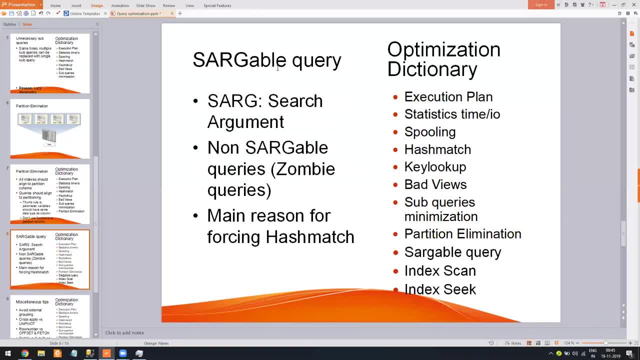 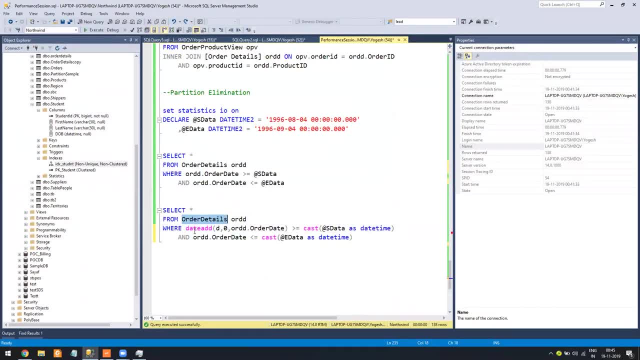 Okay now, last but not the least, is the searchable queries. searchable queries we have seen already in example. Now you won't identify, as I used this syntax where I added this function, So this becomes like non searchable query. searchable means search argument. the moment I used a function on my 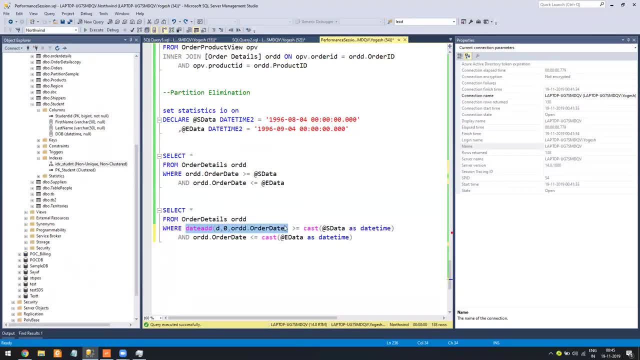 Any Column. it becomes non searchable because SQL server cannot determine the output While running the query. so it goes for crazy operation like it did. it did partition elimination, it went to hash match in the first example and so on something. So I will create nothing, but you make the output determined non deterministic, also like 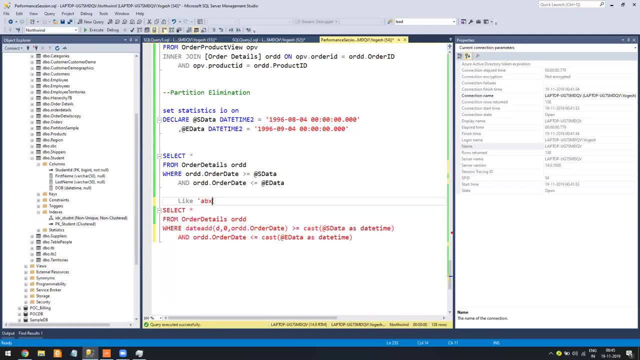 you use like. so when you say X, Y, ABC, Percentage, this is deterministic. it knows it start with ABC. but the moment you say percentage ABC, like It should, Then it Because it has to scan through all the data, so searchable queries are very common- never. 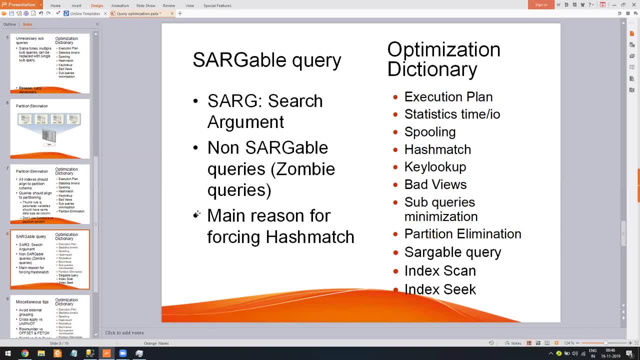 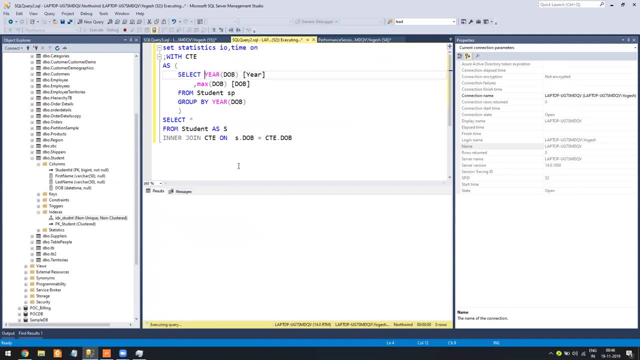 so the basic example is: never you can say, let anyone use functions on columns in where closer joints, Till the time they can be ordered what they have to do it, they end up doing hash match. you remember like we already have this index. let's see, we already have an index, so what? 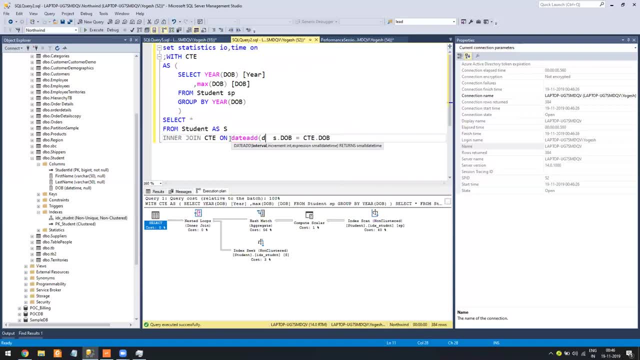 I do is I add this date add function, Just add zero date. So here the join is nested join. unless you look, so you can see if I run- now it goes to hash match, hash matches, again unsorted data, and now it even it is not giving suggestion. 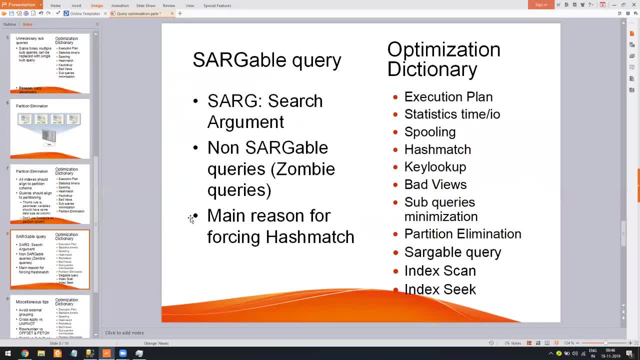 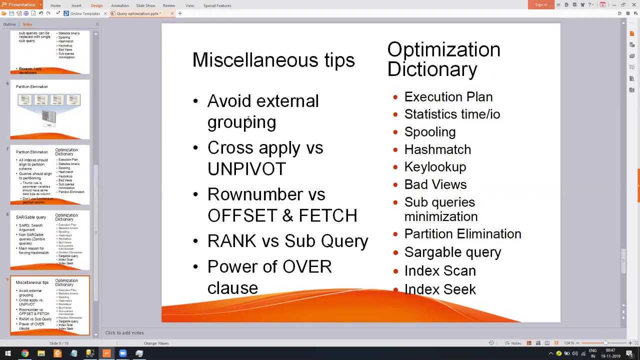 because it cannot determine. So what it do is it make your query to go for hash match in a lot of the sense. so always make your query searchable as much as possible. award as many functions as possible in where close You can say joins Miscellaneous tips. it's like award external grouping. external groupings like a lot of. 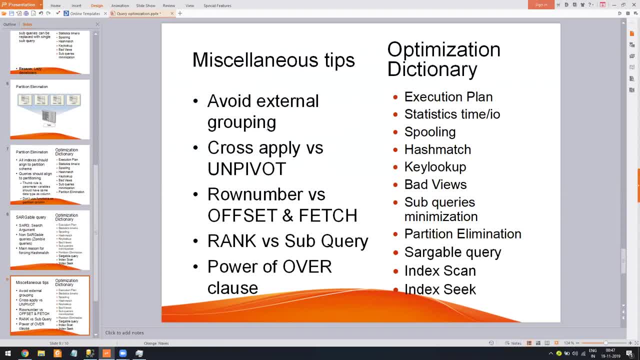 time I've seen people doing same grouping again and again, and again, Like suppose you have table order and order details and you want to also get the count of order one customers. you can say please. so instead of grouping at the bottom you can do it on the top. 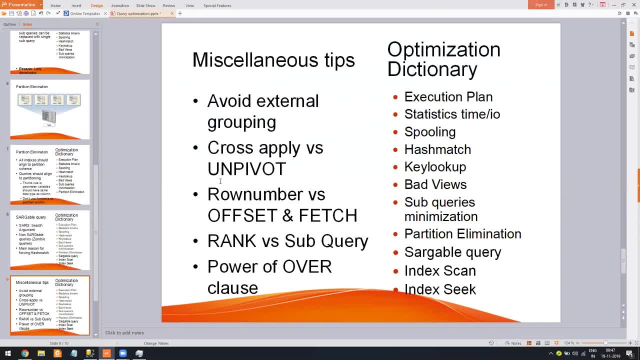 So there are multiple things: use cross, apply and pivot to make your data, Use row number and fetch. offset and fetch to get good, say, if you don't have to get serial number of the records and you just have to get top 10 and top 20 and those kind. 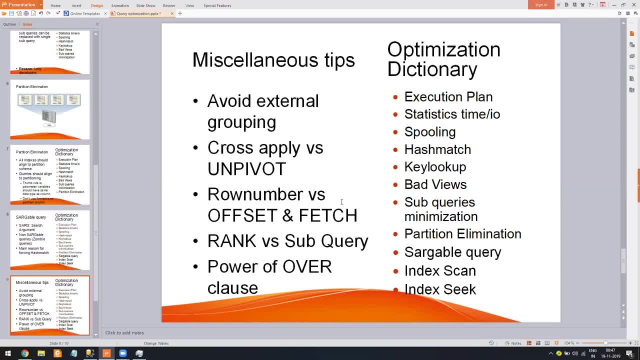 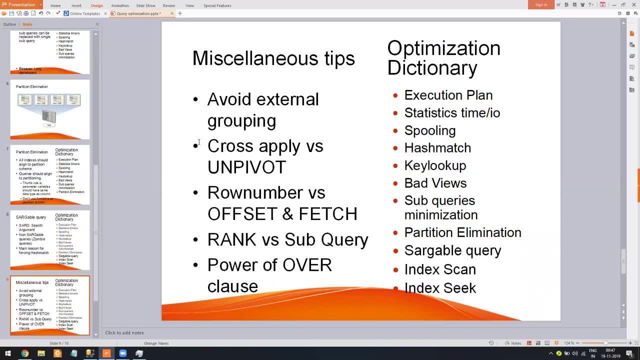 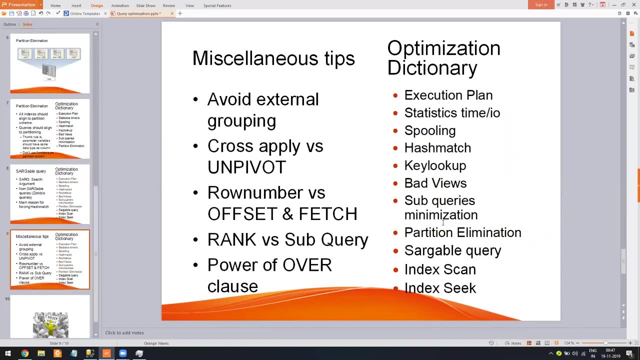 of records you can do, and with pagination you can do with offset and fetch. it's very good. It's now very better than using the row number and doing it rank versus sub queries, like use rank, like these are like which you can use. I hope you must have like now you have known like how to solve a problem, how to figure.